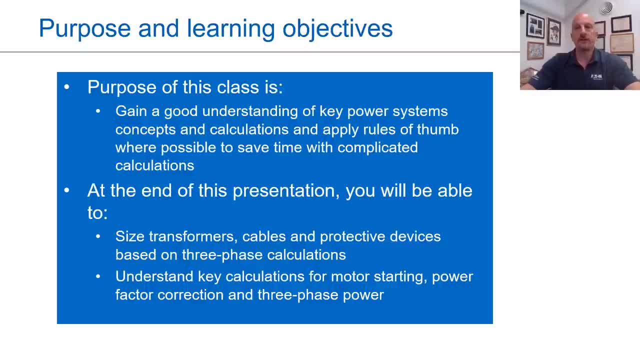 rules of thumb. So if you're thinking about the person sitting next to you that's been in their job for a long time, we want you to understand how do they come up with these calculations. At the end of this presentation, you'll be able to size transformers, cables. 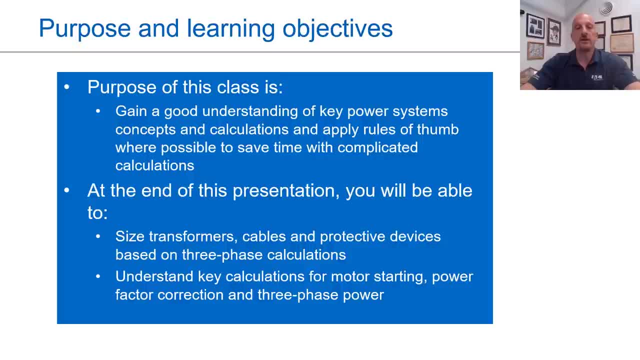 and protective devices based on the three-phase calculations, and also to be able to understand the calculation for motor starting, power factor correction and three-phase power. Engineers love to write on things like a napkin- maybe at the back of an envelope, as people always say. 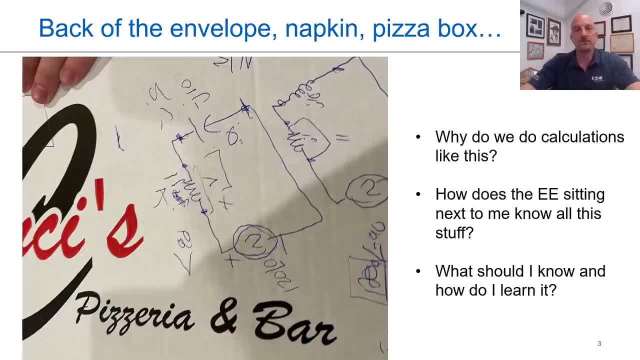 or one night when I was sitting at my kitchen table with my son, who's in engineering school, we were writing on the back of a pizza box, and it reminded me of the fact that engineers love to draw and love to do these calculations, to think things through, And so to me having the capability to 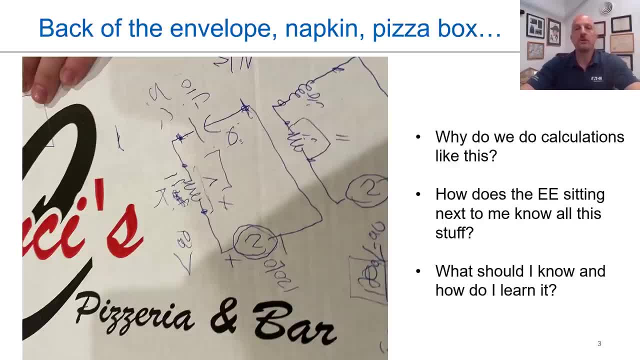 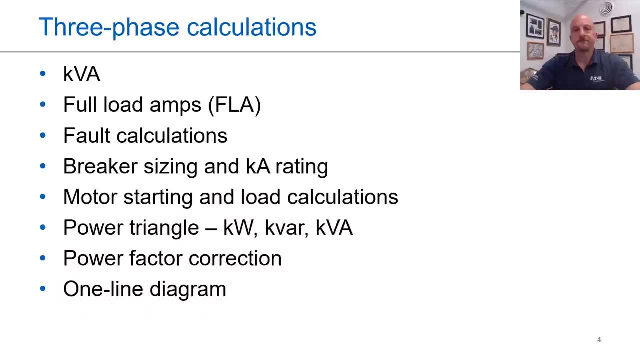 come up with those numbers on the fly is important and, as an engineer, you need to understand where those equations come from and how to use them quickly and correctly to get you the right answers. In this session we'll talk about three-phase calculations, so we're going to simplify it to 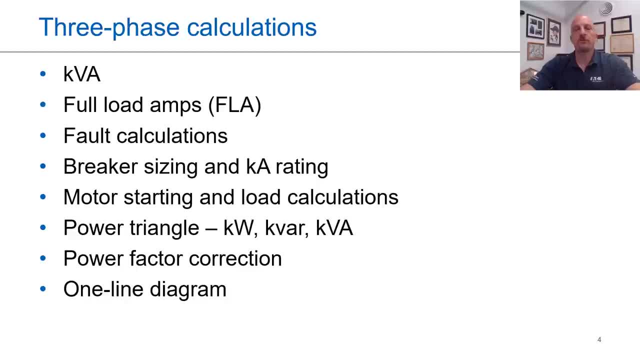 those calculations that are appropriate for three-phase. There will be one or two that are single-phase, but we'll talk about those when they come along. The one thing that's important is really kVA. That's the main equation that we're going to use. 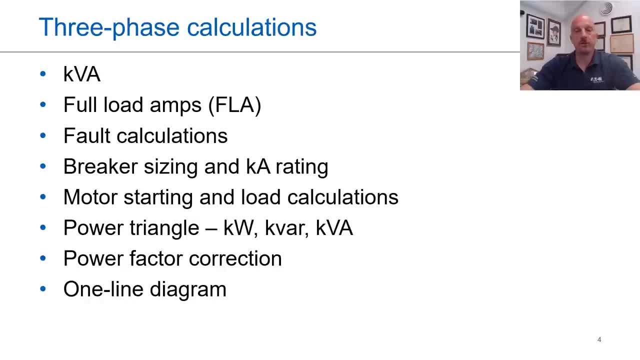 from the simple calculations of kVA, including voltage and current and the square root of three, were appropriate. We're going to talk about full load amps. How do you size the circuit breaker that comes into the circuit breaker? So the circuit breaker is a circuit breaker that goes into a transformer or goes out of. 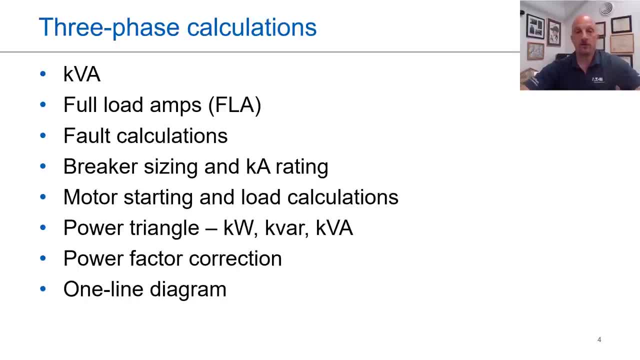 a transformer or goes into a panel board or switchboard. And then how do we calculate fault current And where do we calculate fault current, Breaker sizes and Ka ratings for that fault current? and then motor starting and load calculations, The power triangle, one of my, 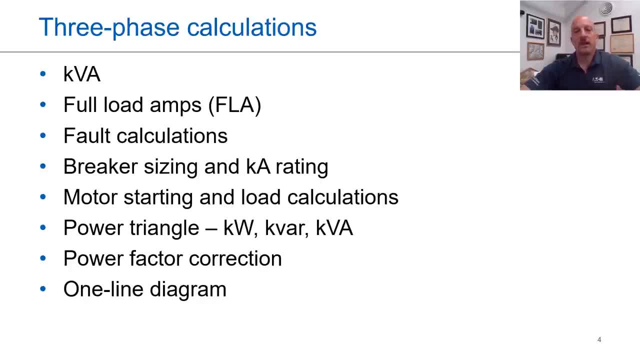 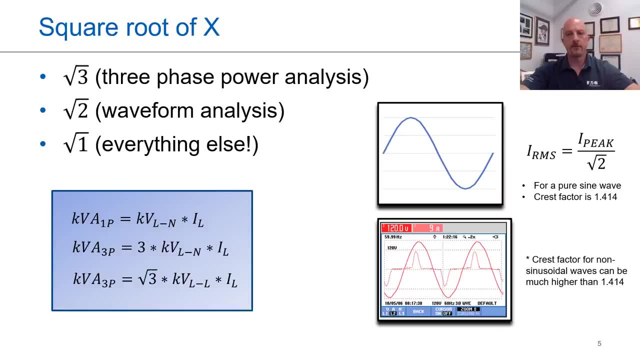 favorite things to talk about: kilowatts, kV and kVA, and then power factor correction. And how do we use a one-line diagram to get all that information and put it together Okay, so when do we use the square root of three, the square root of two or the square root of one? 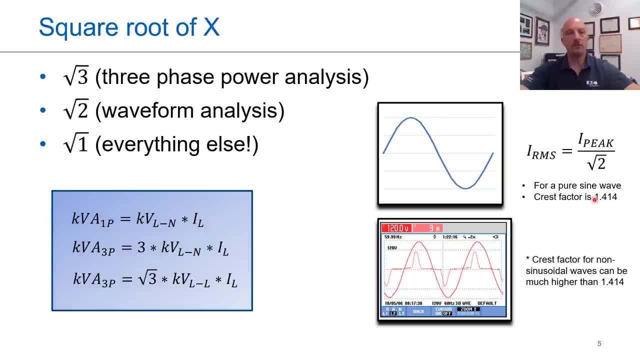 The square root of three is when we have three-phase calculations. Now most people think that volts times amps equals watts, and we know that that's not true. in AC power systems, Volts times amps equals volt amps, or kV times amps equals kVA. So when we have single-phase power, 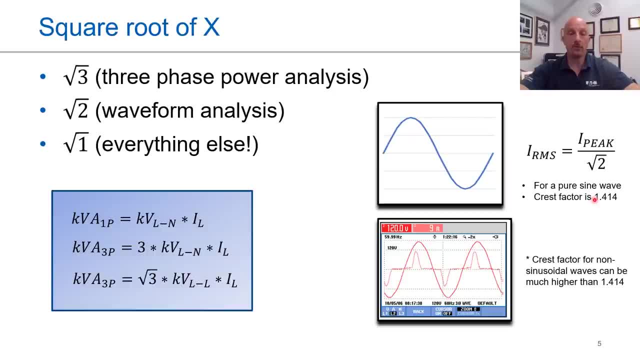 we say kV line to neutral times, I-line equals VA, kVA, single-phase. If we multiply that by three we get the three-phase equivalent for a balanced system. Now the square root of three comes into play when we have kV line to line, because kV line to line 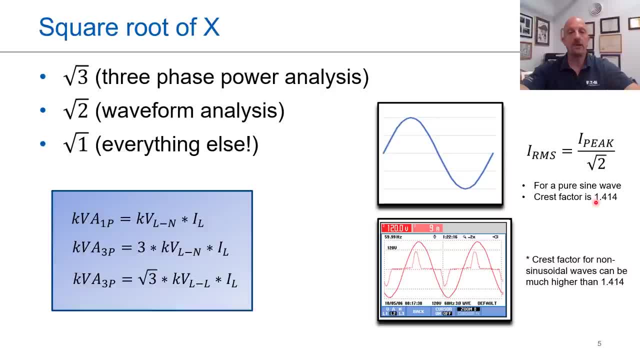 versus kV line to neutral is off by the square root of three kV line to neutral times. the square root of three is the same as kV line to line. So when we have our typical three-phase power calculation we're going to say kV, kVA. three-phase equals the square root of three times kVA. 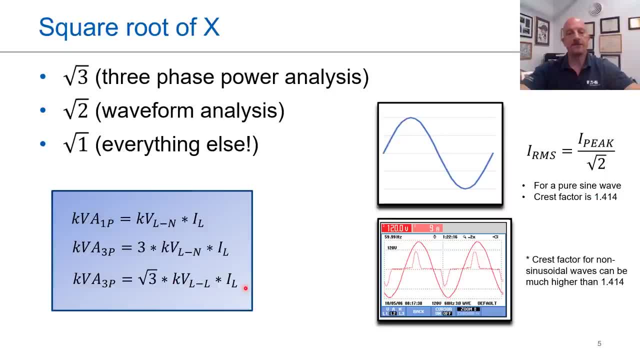 line to line times, the current, And that's going to be the equation that we're going to use a lot for the rest of the calculations for our transformers. When does the square root of two come into play? That really comes into play when we're talking about the RMS versus peak. 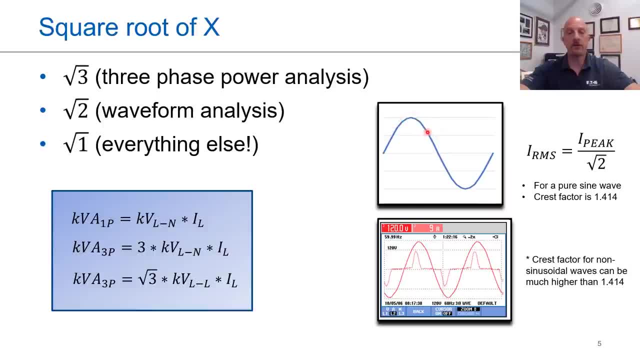 Now, if you look at the peak and you compare that to the RMS, which is more of an average value, it's typically off by the square root of two when you have a very nice sinusoidal waveform. Where that doesn't happen is when you have harmonics like the bottom picture, where the 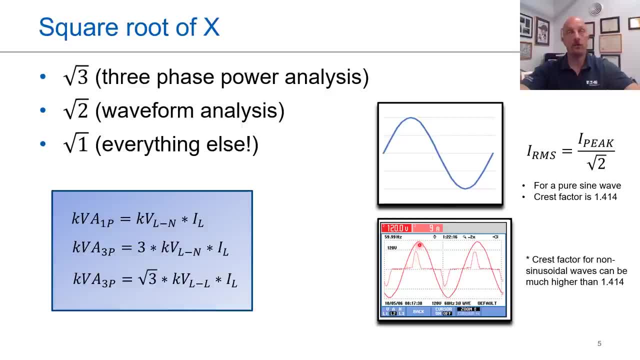 RMS has a crest factor or a peak over the square root of or a peak over the RMS of maybe three or a number considerably higher than the square root of two. So the square root of two comes into play for those kind of things, And as a consultant you might not run into that as much unless you're. 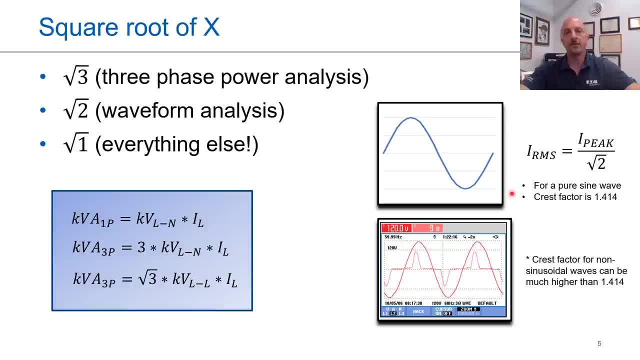 dealing with waveforms and harmonics and things like that. But the square root of three will be all around And if you understand those equations on the left, that's going to be a big deal. if you can understand the square root of three, The square root of one, you can use for everything else. 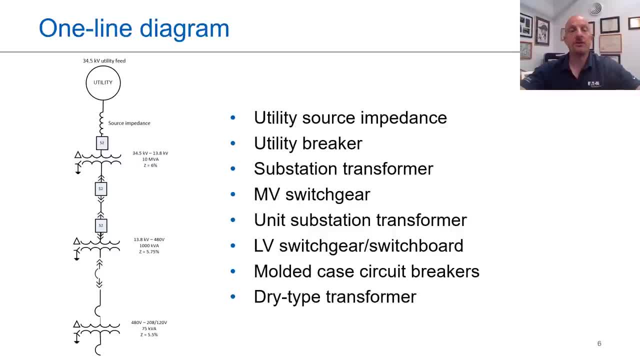 So, as a consultant, why do you need a one line diagram like this one? Well, it's really important. if you're going to try to do calculations, you really need to have a good understanding of the actual numbers of values for the equipment, And there's two things associated with that that are: 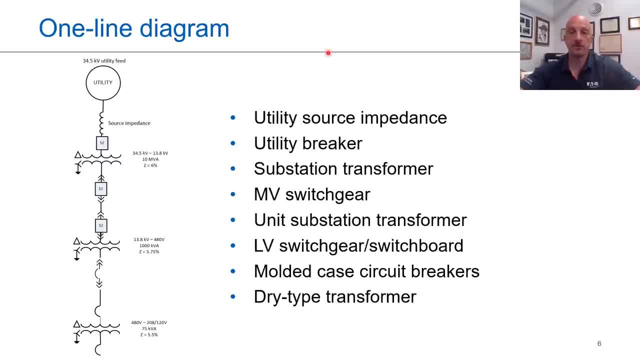 important One is you don't always immediately trust the one line. You have to make sure that it's accurate. But the second thing is really to make sure that you have all the data that's on the one line that matches up with your equipment. So sometimes you have to field verify again. 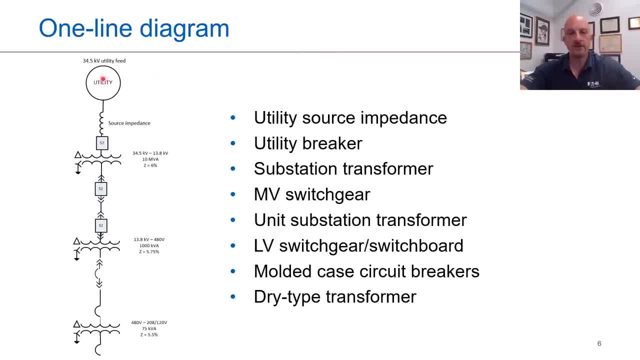 the data that's on the equipment and so forth. But if we have the one line, like in this case, we can calculate and we can use the utility source, impedance, utility, main breaker, substation, transformer, media voltage, switch gear, like we show in the middle. 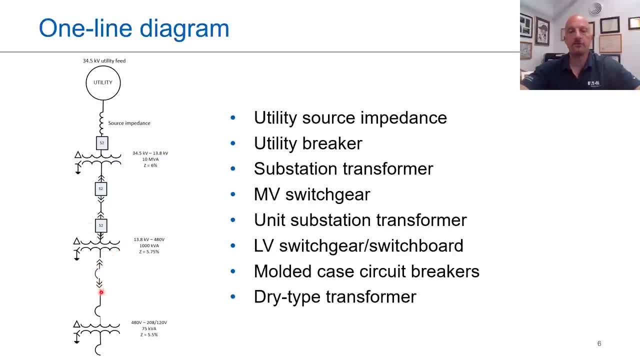 unit substation transformer, for example, and then low voltage switch gear or switchboards, then molded case breakers and dry type transformers down through the system. So all of that equipment with its proper information on the one line is going to be helpful to doing your fault analysis and your load flow calculations and all the things you'll. 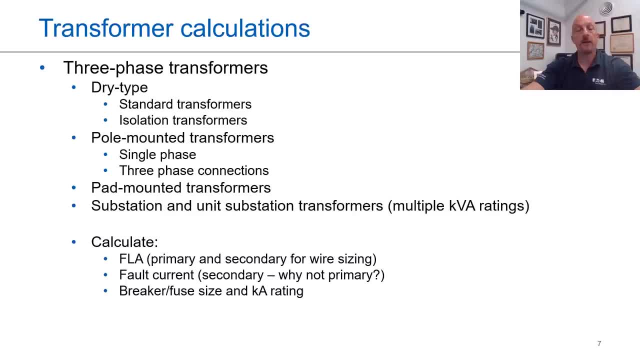 do as an engineer or consultant. Now what we're going to do is we're actually going to go through and calculate full load amps on the primary and secondary of a transformer, the fault current on the secondary and also the breaker or fuse size and the Ka rating of those breakers. We're going 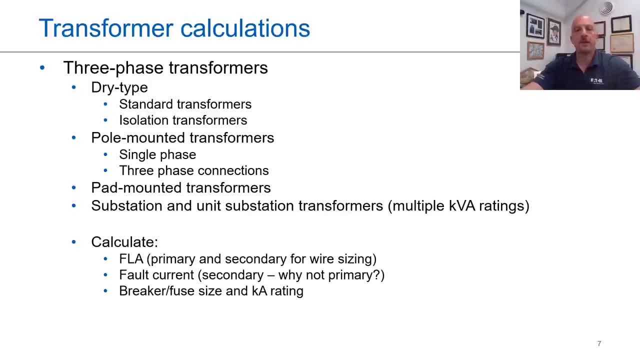 to talk about how that comes into play here. Now I'm going to actually take you for a walk and show you a couple of these transformers so you can physically see what's going on, What they look like, because they're not just squiggly lines on a piece of paper. 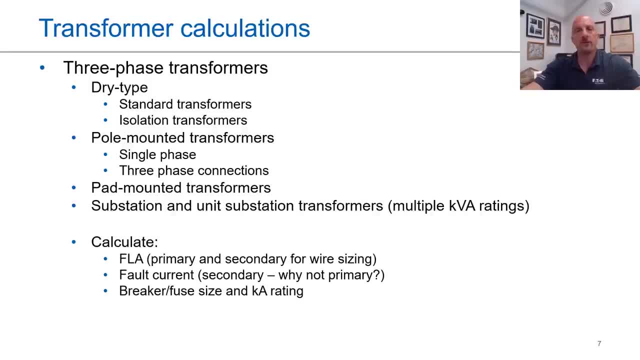 they're actually physical devices And I'll show you the difference between the liquid filled ones and the dry types and the pole mounted ones and the things you're going to have in your one line diagrams. that won't necessarily correspond to something physical you've seen before. 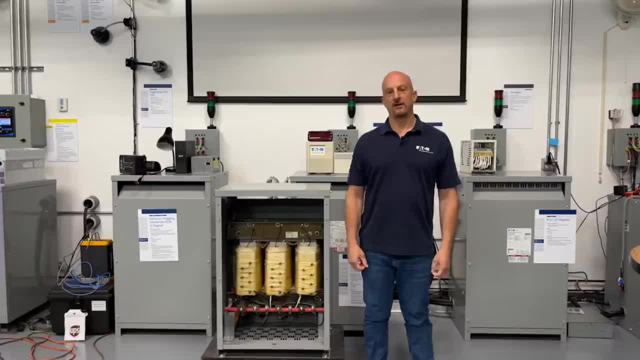 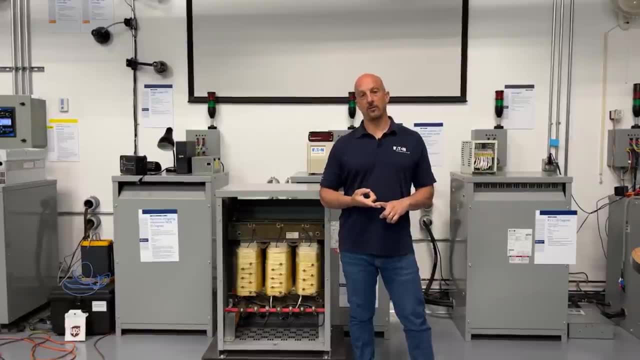 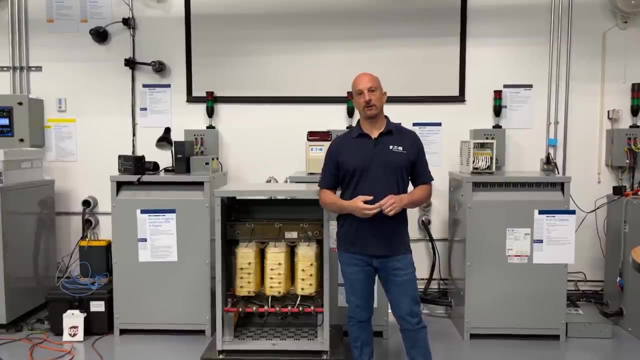 And I think that's really important to see how that all comes together. So, to get to the calculations that we need for a transformer like this, we want to think about full load amps on the primary, full load amps on the secondary breaker- primary and secondary- and then also fault current on the secondary. How are we going to get that? 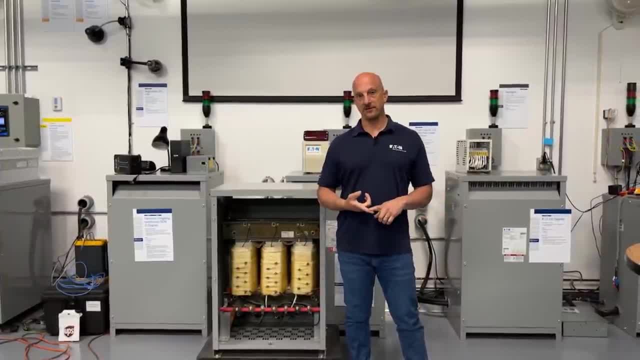 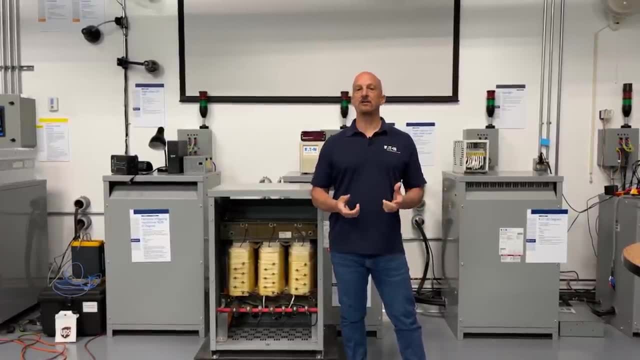 information. Well, what we're going to do is we're going to go up to the nameplates of these transformers and we're going to find out the information that we're going to need to plug into our equations to calculate those values. Let's take a look at some actual transformers. 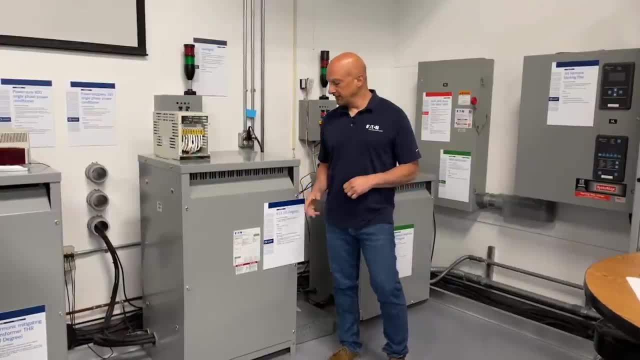 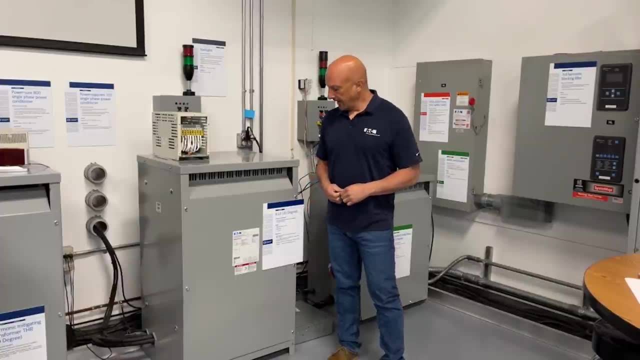 and see the ones that we're going to use in our calculations. This is the first one. This is a dry type transformer: 75 kVA, 480 volts in, 208, 120 out, and it happens to be a k13 transformer. 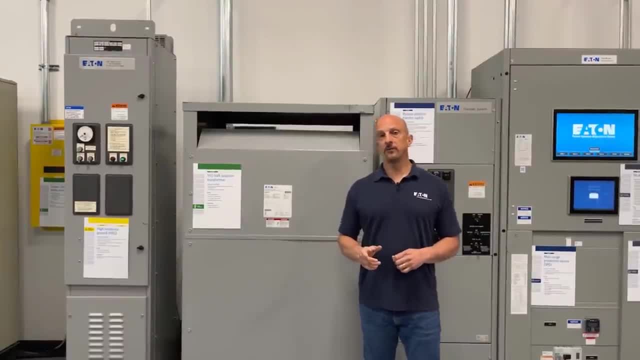 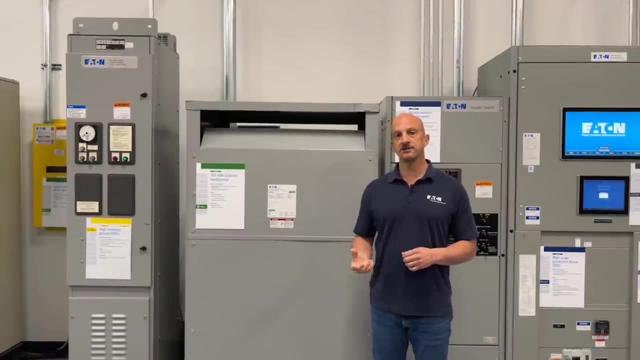 So this next transformer is a little bit unique. We call it an isolation transformer. What does that mean? That means the voltage on the input and output are the same, so we're just using it to re-establish a ground system through the delta y and the y connection on the secondary 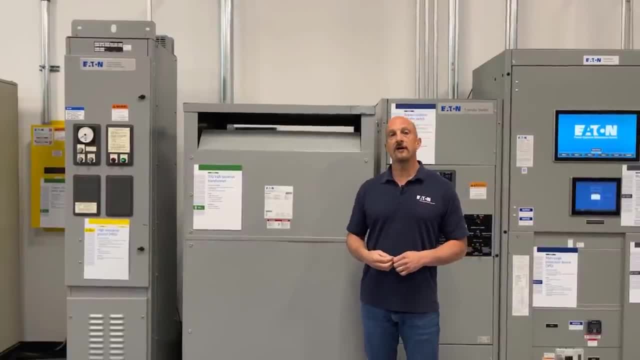 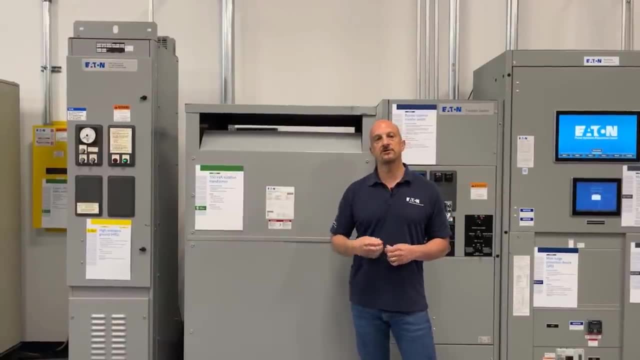 This one happens to be 460 in, 460 out, 550 kVA. It's also connected- in this case not solidly grounded, but to our high resistance ground system, which allows us to have one free ground fault and you might use that on an industrial situation for you. 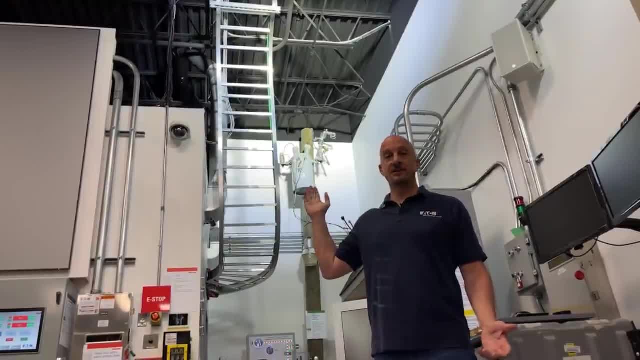 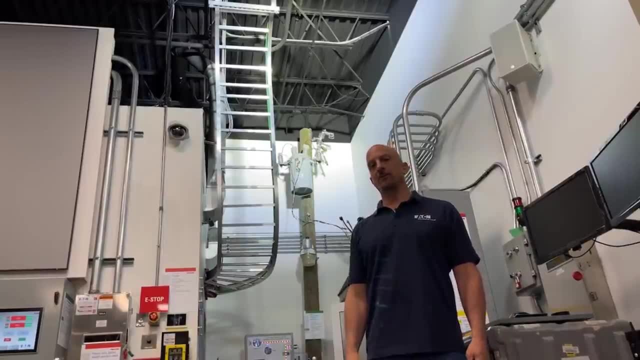 For example. now here's a transformer on a pole. We can see it's single phase. It's 13,800 volts on the input and 240, 120 coming into your house in the output. How are you going to figure out what size that one is? Well, we can see the 10 on there. What? 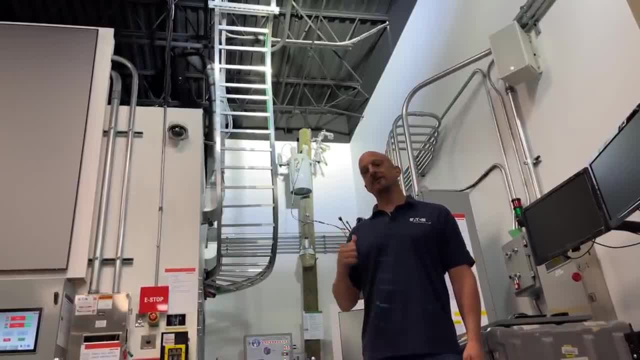 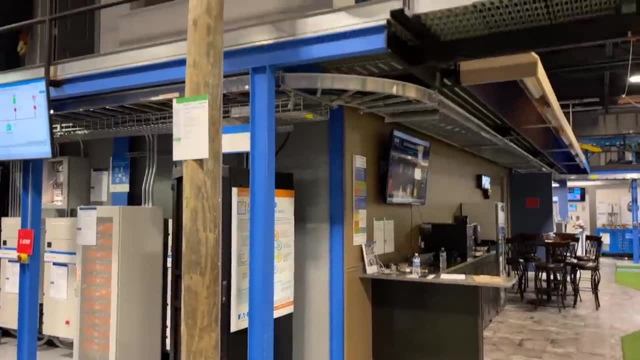 that means is 10 kVA. but the problem is, unless I climb that pole, I don't know what the transformer impedance is. so we're going to have to make some assumptions on this one. Hey, I'm up here, So these ones are a little different. Now again, don't try this at home. I just happen to be up. 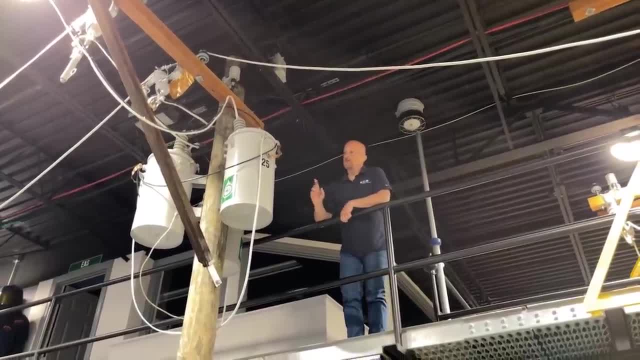 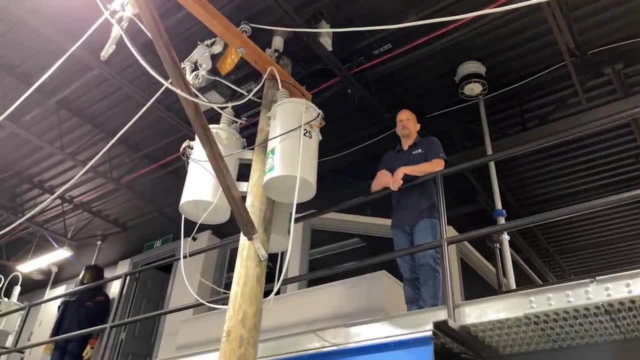 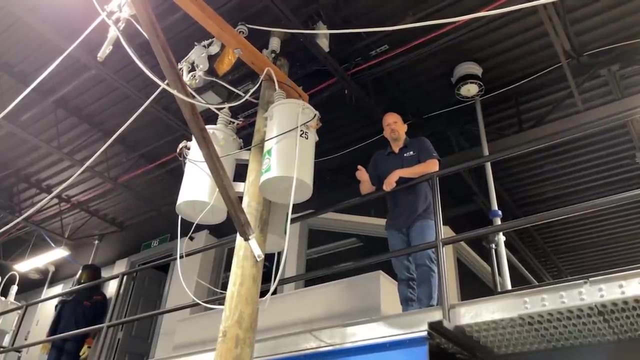 there because I know these aren't energized, but if you look at these transformers it has 25 kVA, so three of them together make a bank in a delta y configuration of 13,800 volts in this case to 480 volts y connected, so 480, 277,. 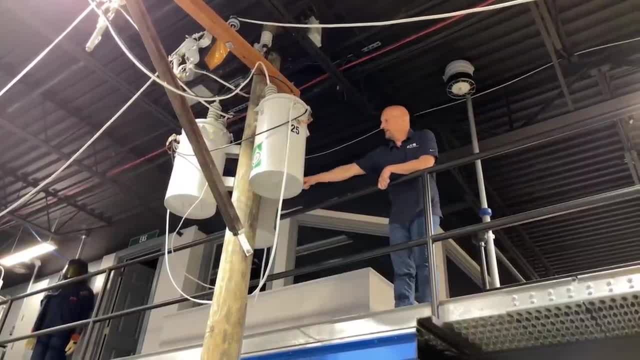 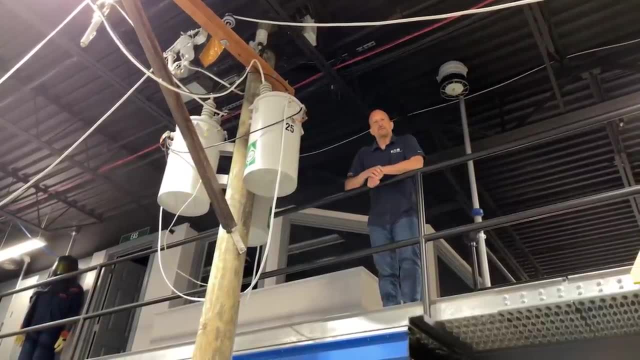 and this one's going to be solidly grounded, and I'm standing right up here next to the nameplate, so I'll show you a picture of the nameplate in the PowerPoint. but again, this is what you might see in front of like a strip mall. Now, this is a 750 kVA pad-mounted transformer. This thing's. 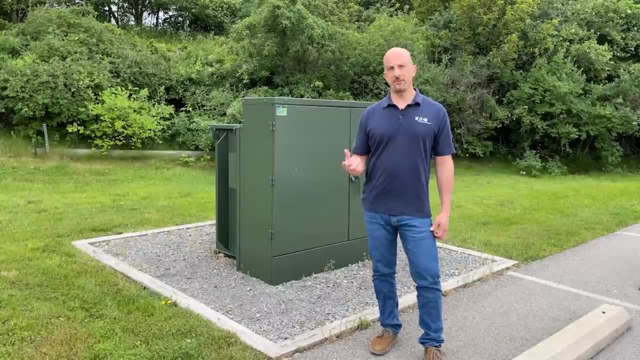 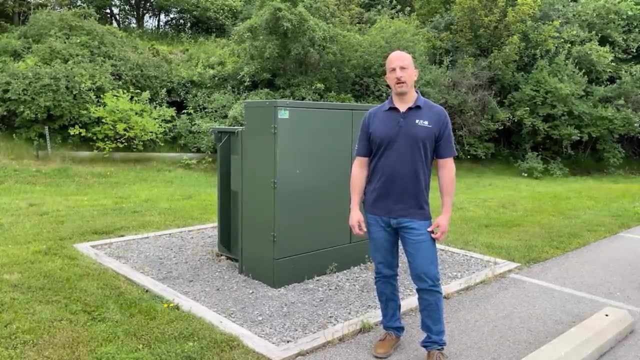 liquid-filled or oil-filled, and it's medium voltage on the input and 480- 277 on the output, for example, or it could be 208- 120 volt on the output. The interesting thing about this is, without opening the doors, a lot of times you won't be able to see the nameplate. 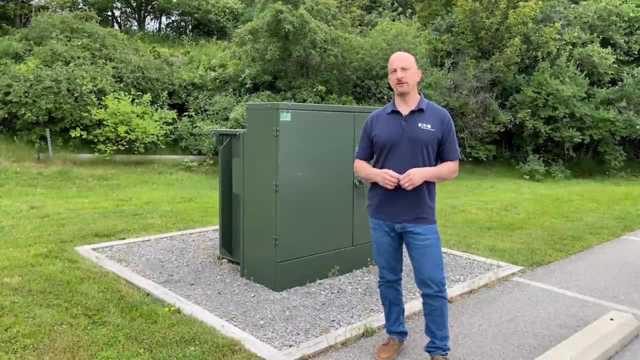 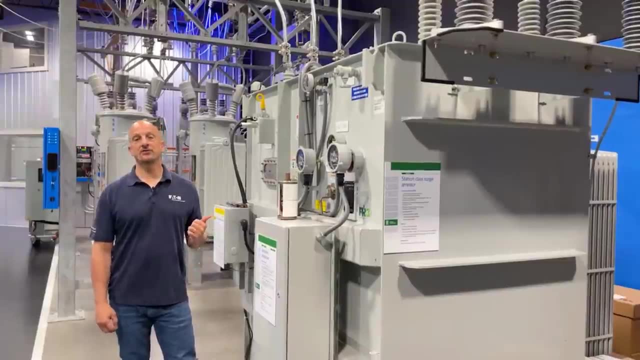 so sometimes they have written on the outside the kVA rating of these units as well from the utilities standpoint, so they know what size they are when they go to replace them if they fail. So this transformer is 5,000 kVA, but it also has a slash rating. 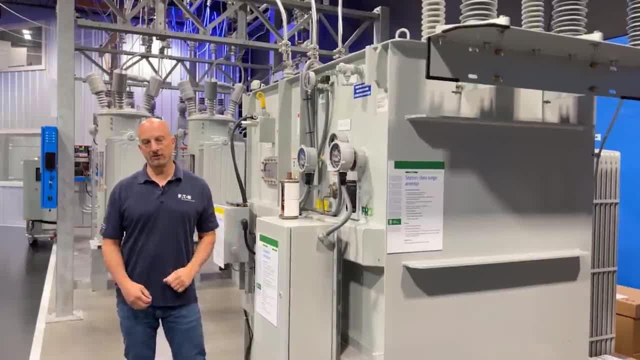 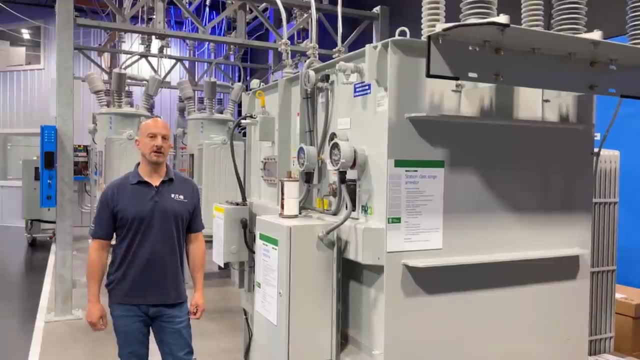 6,250, and that's because we have fans and radiators on the back to cool it down so the oil can move through those radiators and we get more kVA out of the transformer. That's going to come into our calculations for full load amps and also our fault current a little bit differently. 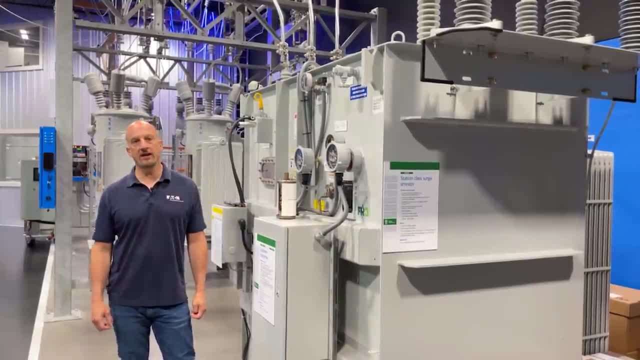 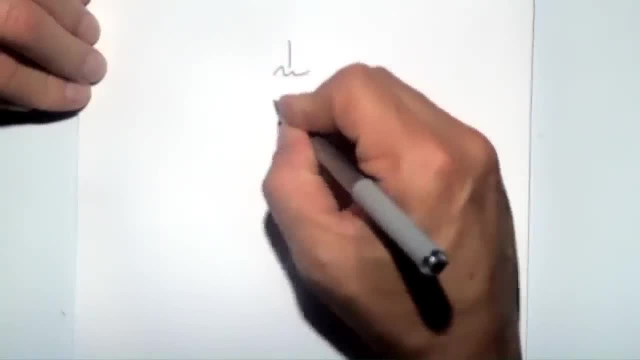 so we have to think about that. This one has 34.5 kV in, 13.8 kV out. Okay, so let's get into the fun stuff. Let's calculate full load amps on the primary and secondary of the transformer. Here I full load. on the primary. I full load on the secondary. Three-phase fault current. I fault three-phase here and that's going to help us determine the wire sizes on the primary and secondary, as well as perhaps the breaker sizes here on the secondary and there on the primary. 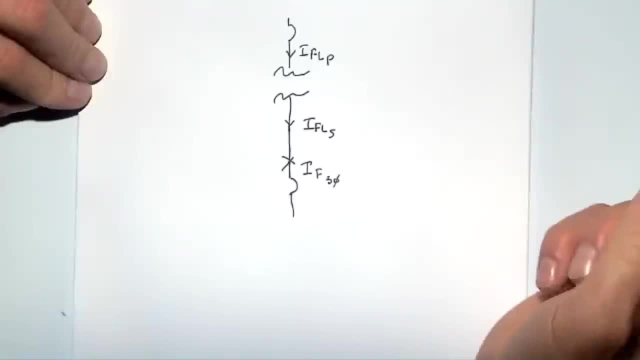 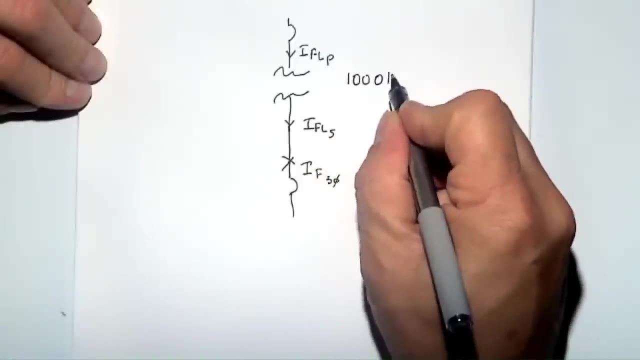 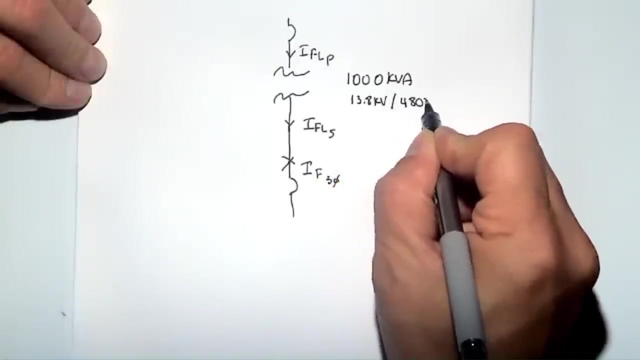 Now we're going to use the information from the transformer. So again we're gathering information from the transformer's nameplate. Let's just use this as a very simple: 1,000 kVA- 13.8 kV- primary to 480 volts secondary impedance: 5%. 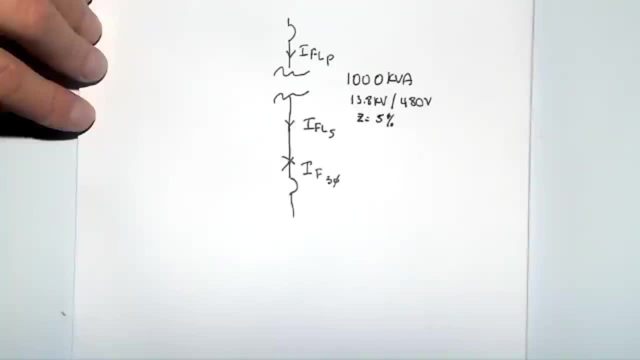 So we're going to go back to the equation that we started with and we talked about for three-phase power, which is kVA. So we have kVA- a 3-phase voltage. that stands for current kV a 3 phase. 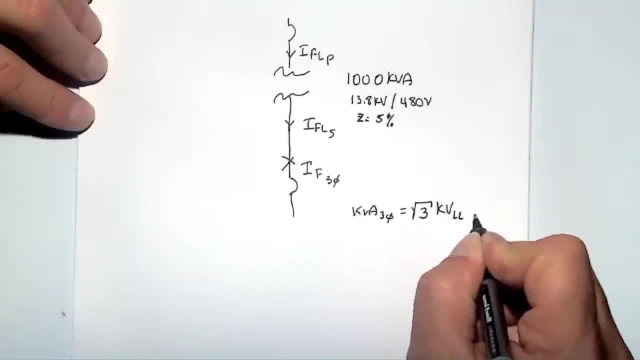 equals square root of 3.. There's that square root of 3 kV line to line times Iline. So if we solve for the current Iline equals kVA 3-phase divided by square root of 3, divided by kV. 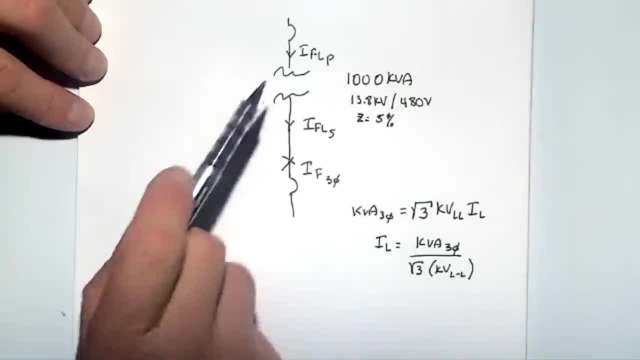 line to line, then we just substitute in if we're on the primary or the secondary, to count the kV and line to line. our current, so for example, current I full load on the primary is a thousand kVA divided by the square root of three, divided by thirteen point eight KB and. 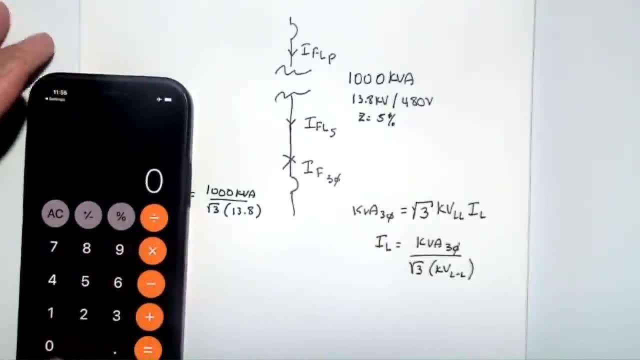 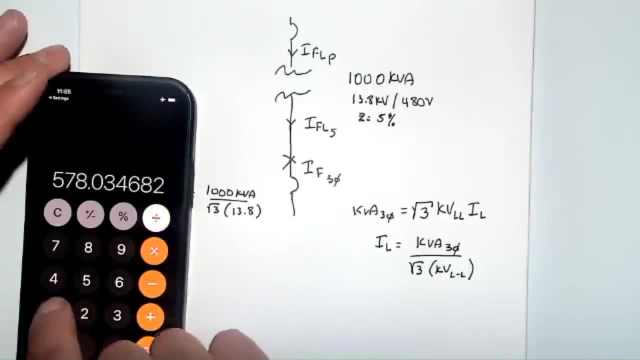 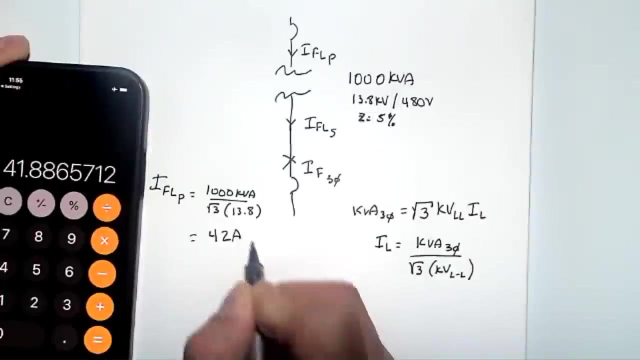 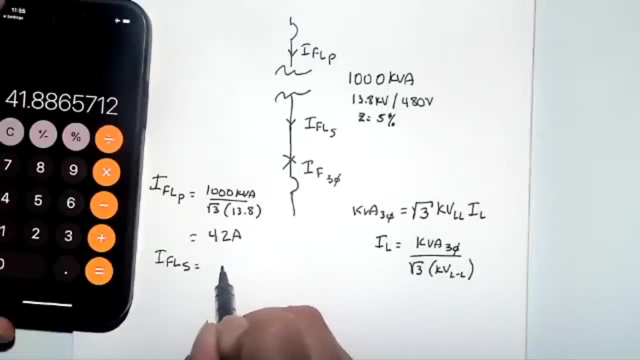 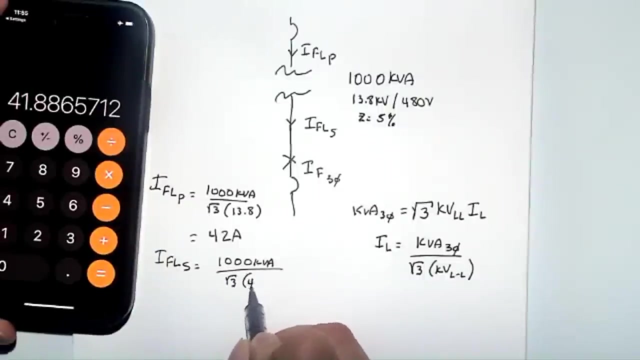 so let's calculate that out: thousand kVA divided by one point seven, three divided by thirteen point eight, that works out to be 40, about 42 amps. okay, now, if we want to look at the secondary current- I full load secondary- we would take a thousand kVA divided by the square root of three divided by 480, right well, 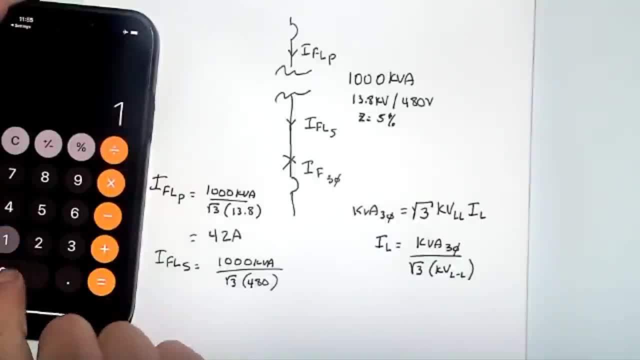 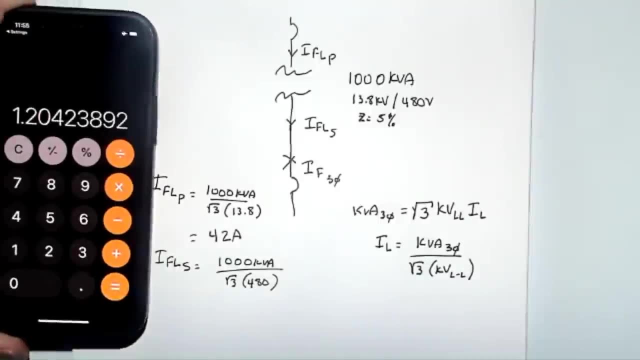 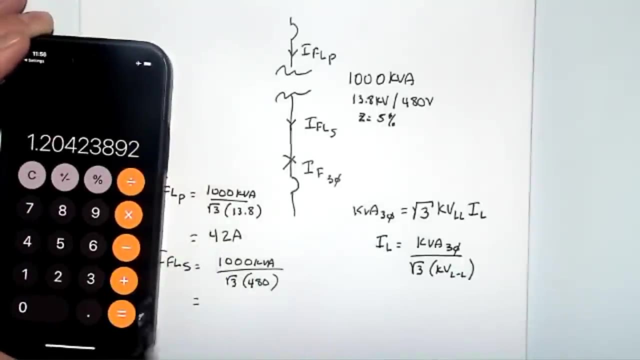 here's what's going to get you in trouble. if you do that, thousand divided by one point seven, three divided by 480, your current is 1.2 amps. and if you have 1.2 amps on the secondary and 42 amps on the primary, you should know that something's wrong. 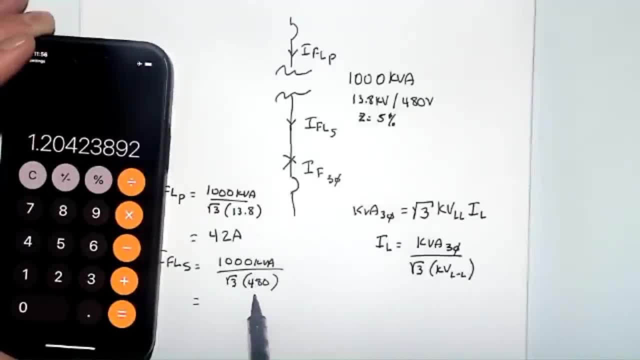 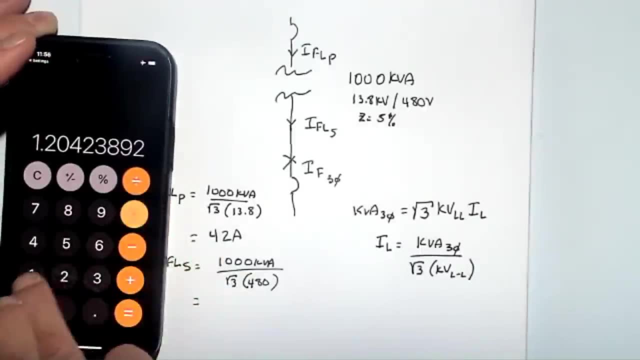 and in fact what you forgot is this is KV on the bottom, KV line to line on the bottom. so we have to do 0.48. so if we divide that or multiply that by a thousand, we end up with the correct answer, which is 1204 amps and one. 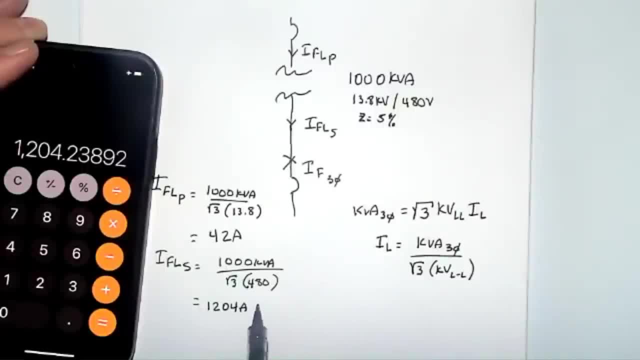 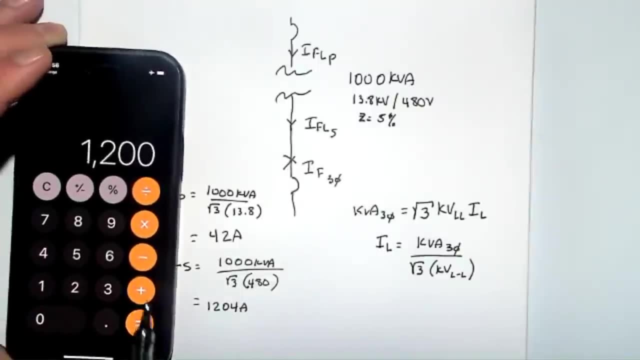 really cool thing about 480 volt systems is that if you take a thousand kVA, a thousand, multiply it by 1.2- guess what- 1200 amps, 1204. so there's a good rule of thumb that basically says: if you have full load amps on the secondary of 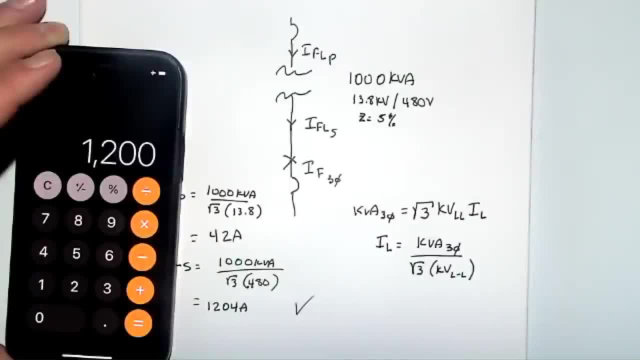 a. if you have full load amps on a 480 volt system, it's about 1.2 times the kVA rating of the transformer. now let's look at the KVA rating of the transformer. now let's look at the KVA rating of the transformer. now let's. 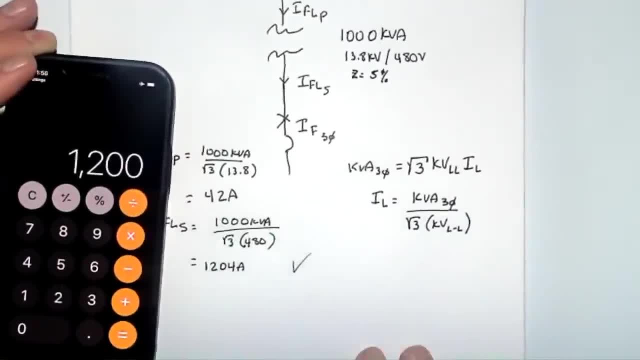 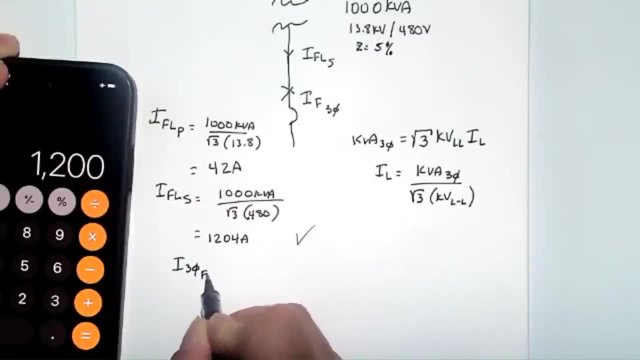 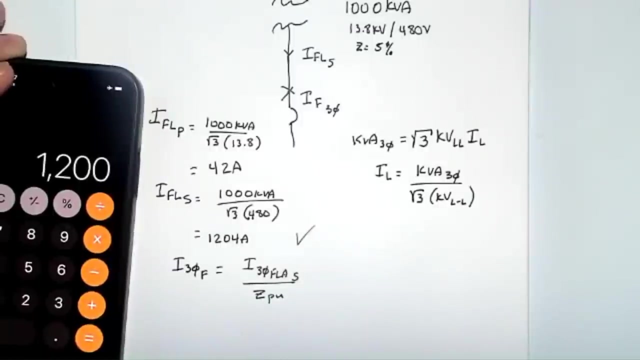 take this to the next step, which is: how do I calculate my fault current? so if I want to calculate my fault current- I three phase fault- it's actually very simple. all we do is we take I three phase full load, full load amps secondary, divided by the impedance in per unit, and we'll talk about what. 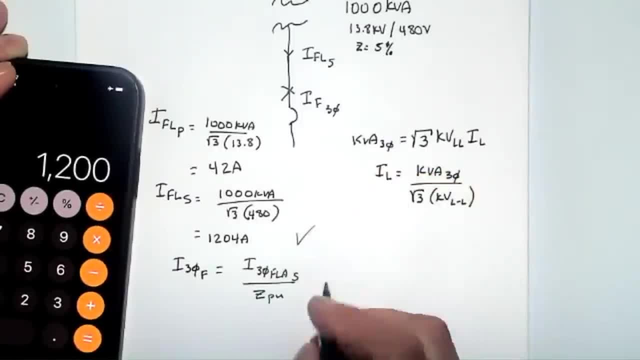 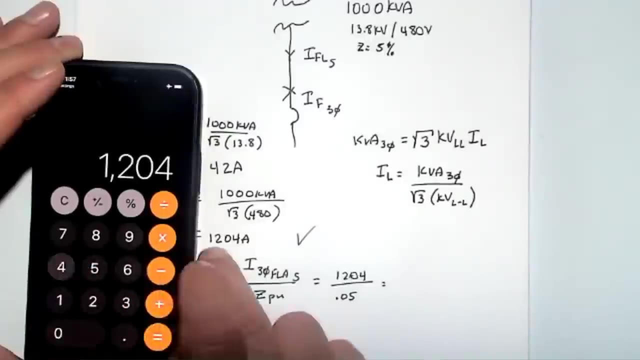 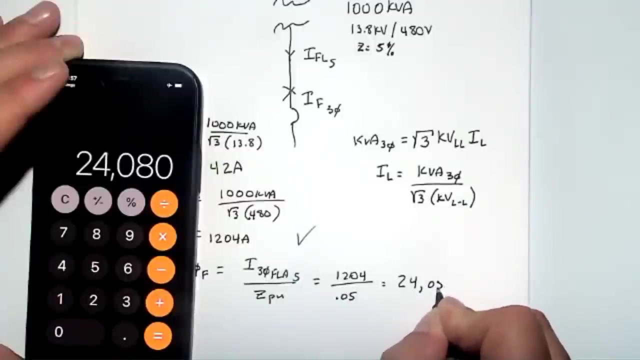 that means basically per unit at five percent. per unit is point zero five. so we take 1204 divided by point zero five and we get 1204. 1204 divided by a point zero five and we get 24, about 24,000 880 amps or 24k a. that's our. 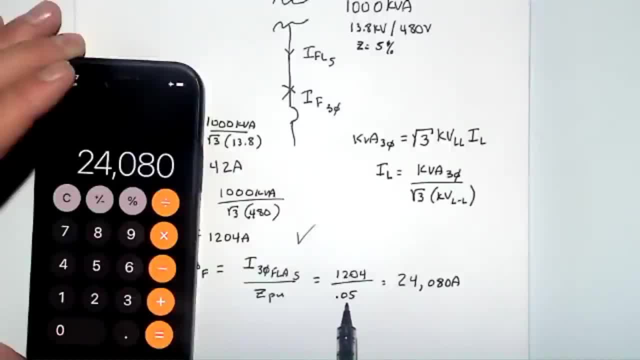 fault current this number, since the impedance is 5% or point zero five. this number is 20 times the full load amps. again interesting things to think about when you think about the impedance. 1 over 0.05 is about a ratio of 1 to 20. 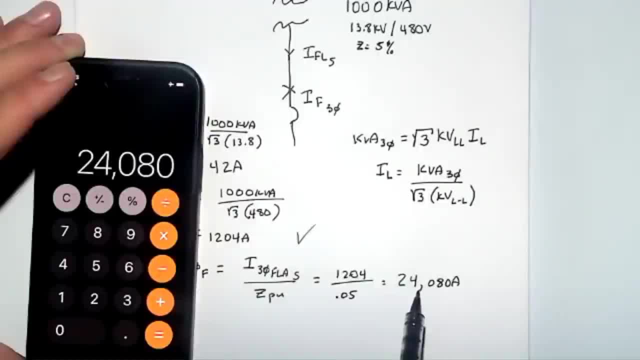 so the ratio of the full load amps to the fault current is 20 times, and that's how we're going to size our K rating for our breakers. so those are just a few of the things that we want to think about now. on the next page we're going to talk. 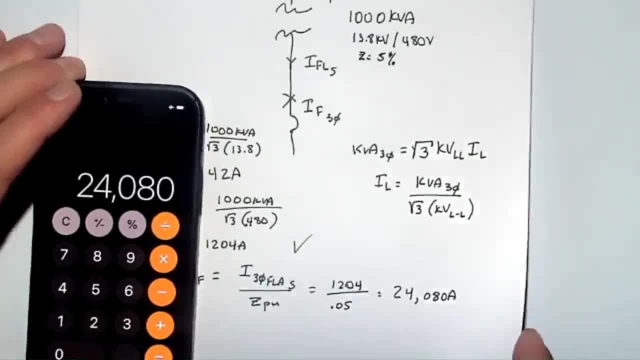 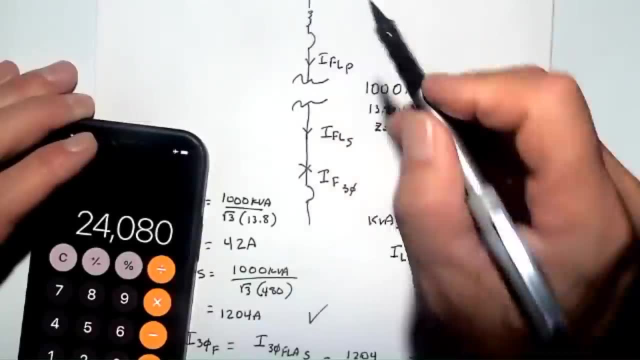 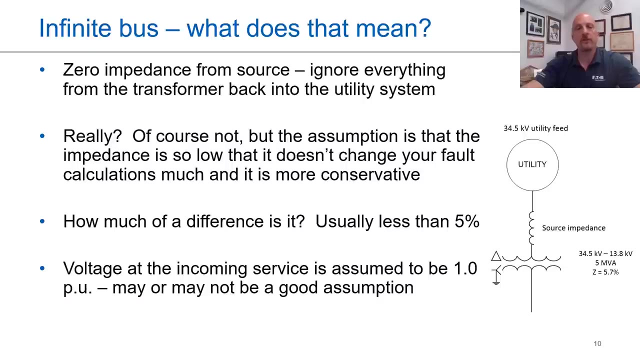 about the infinite bus, and why do we not calculate the fault current on the primary side? the reason we can't is we don't know what the impedance back here is, so let's talk a little bit about that. so what does an infinite bus mean? an infinite bus basically says that we have zero impedance all the way looking. 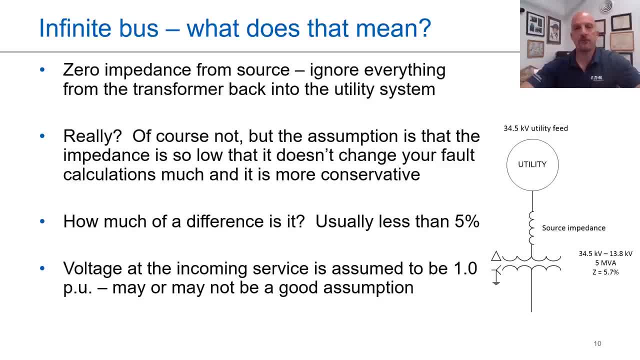 back to the source and we know that's not exactly true. of course it's not true, but if it's low enough, the calculations work out so that we can actually ignore the fault or the ignore the impedance of the transformer and we can just use the nearest upstream transformers and 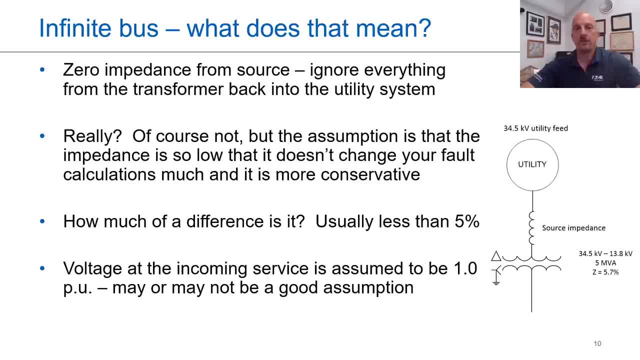 cables and everything else and just use the nearest upstream transformer as our main source impedance. that becomes especially important when you're doing things like fault calculations and even harmonic analysis, really to be honest with you- for resonance and things like that. so if you can understand transformer impedance and you can calculate all that, then you can figure out. you know how. 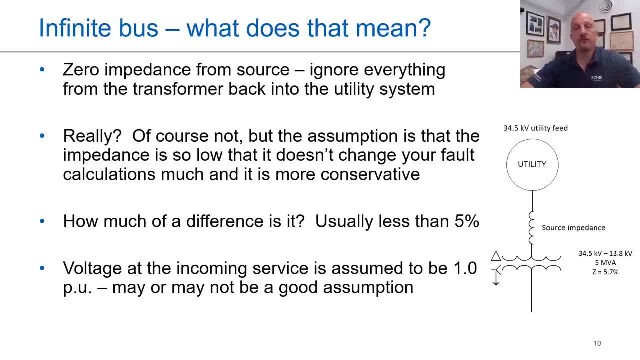 that comes together. how much of a difference is that? it's usually less than the conservative side. so if we ignore that impedance, what are we doing? we're making the impedance lower. if the impedance is lower, our fault current is going to be higher. so actually it makes you know for a better or more. 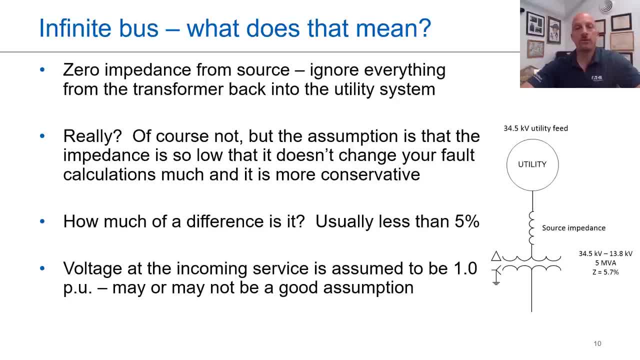 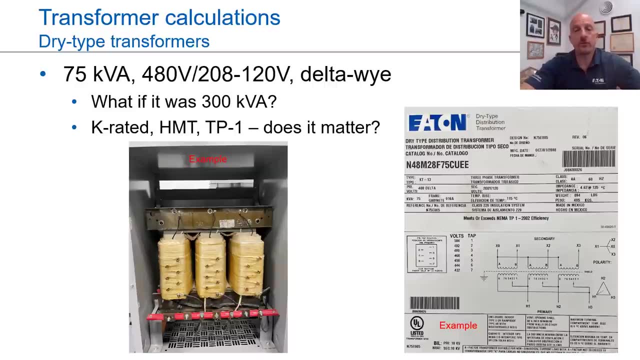 conservative calculation. now what if our per unit voltage is not 480 or 13.8 kV, but maybe five percent high again? we have to think about that, so we may actually add in a little bit of full current into our final calculations. okay, so I showed you a few transformers earlier. 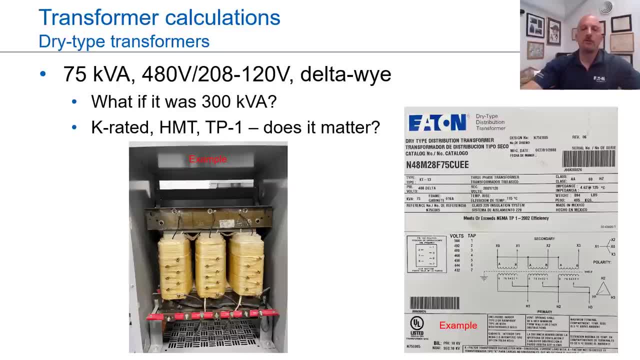 let's start to do some of those calculations that we talked about. so, again, we're going to try to look for primary and secondary full load amps and secondary fault current. now, here's the transformer, here's the inside of it, and typically you're not going to get to see it with a name plate with the cover off of it. so what we usually do is we: 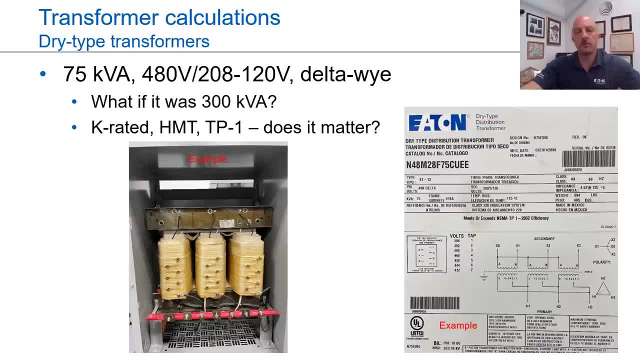 walk up to the name plate and we start to gather the information that's on the name plate. what are we looking for? kva rating, we're looking for primary voltage, secondary voltage. sometimes we worry about the configuration of its Delta Y or Delta Delta, for example, but for these calculations that we're 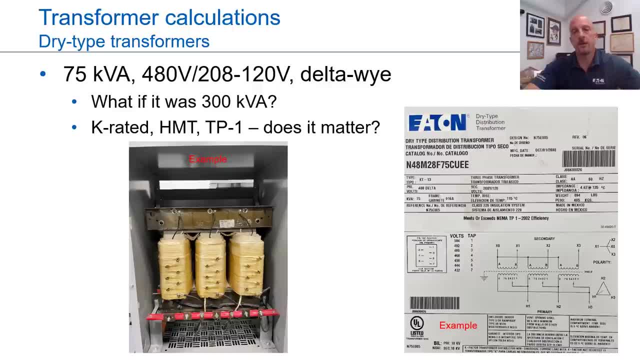 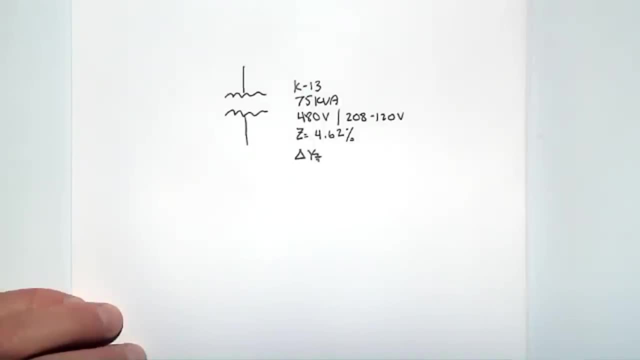 going to do it honestly, it doesn't matter for that particular part. and then we also look for impedance, and that's the Z in the Z value. that's on the transformer. okay, so let's start in with fun stuff, with the actual transformers that we saw on the pq lab. 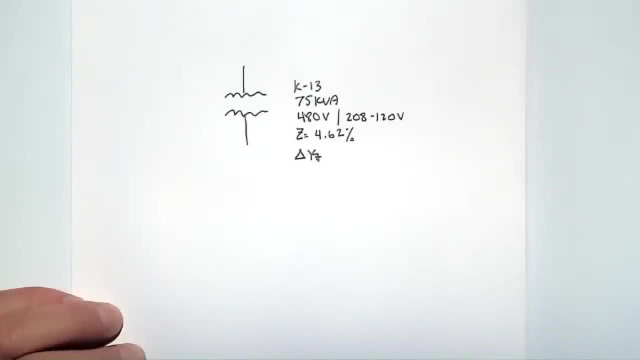 here. this is one of my favorites and you'll see why in a minute. it's 75 kva, k13, which, by the way, we have an X dos. so now you could probably buy a switch to plug aril and do the same thing. but if you can't find out why, you 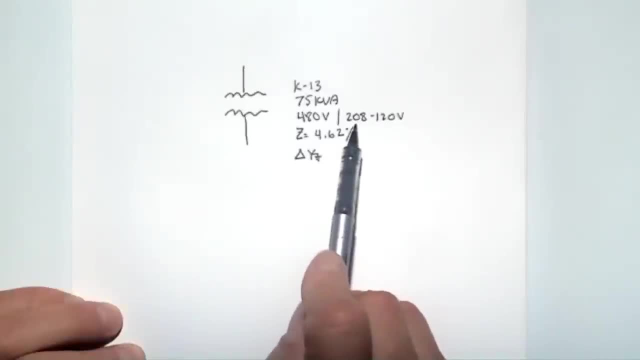 should look for the power, or, quickly, you can use a dual brush like this, which is probably going to help you, and we're going to be right in here for flat levels and we're going to be laying WrestleMania and then we're going to have the positive voltage that we need. so we're going to have the, you know. 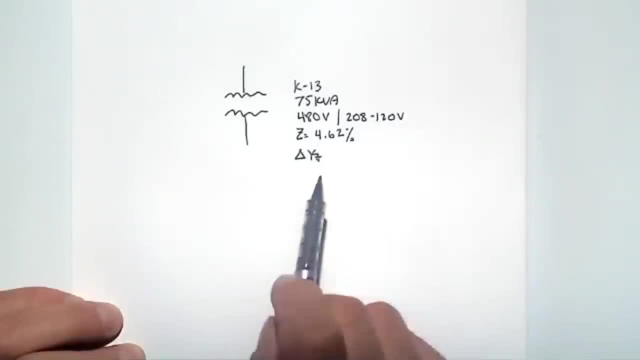 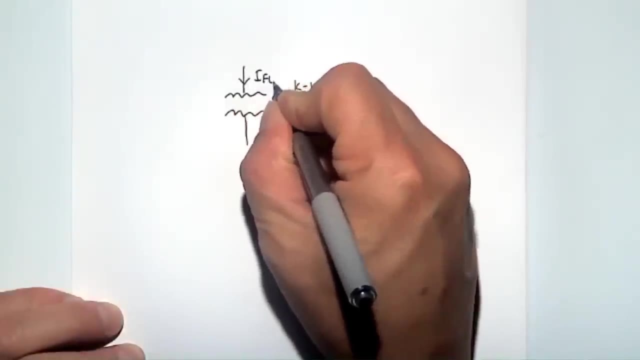 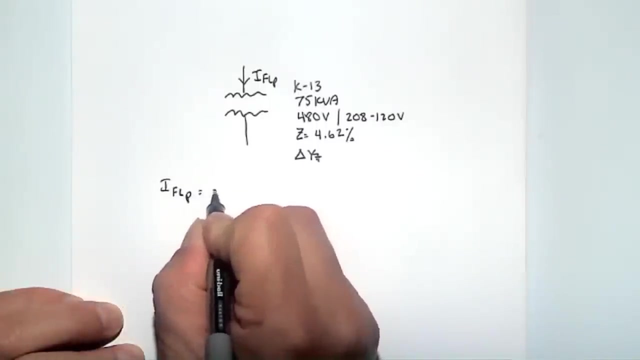 connected in a Y, so 120 line to neutral and the impedance is 4.2, 62 percent. so let's calculate I full load primary. all right, so we go back to our equation we had before. I full load primary is going to be in this case against 75 k VA. so 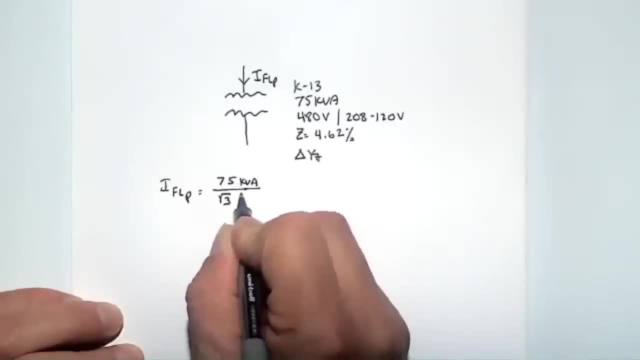 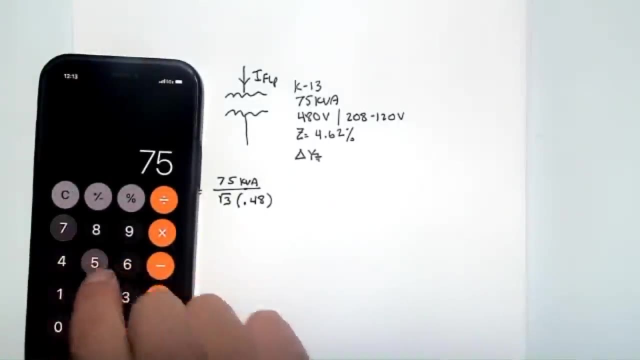 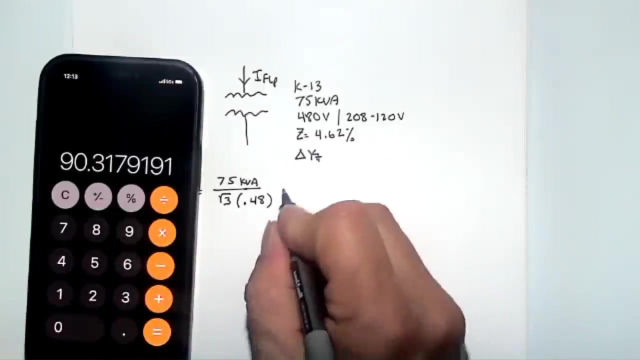 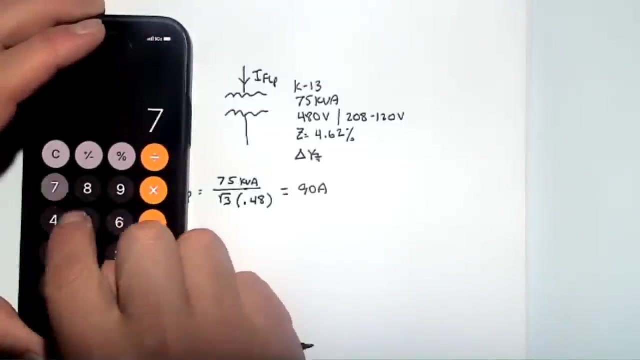 it's k VA divided by the square root of 3, divided by k V, and again we got to make sure we use 0.48 here. so we take 75 divided by 1.73, divided by 0.48 and we get 90 amps. remember what I told you earlier: 75 times 1.2. 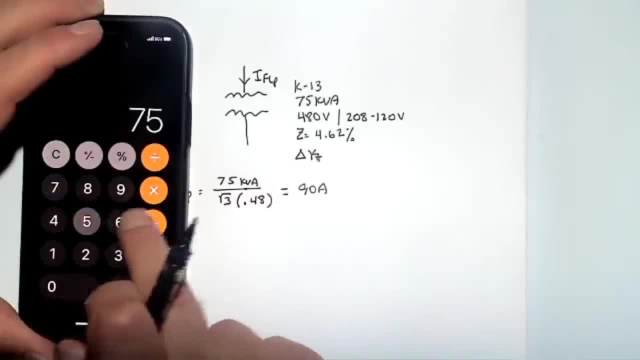 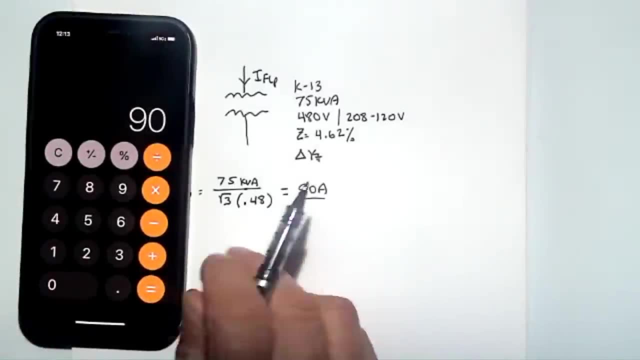 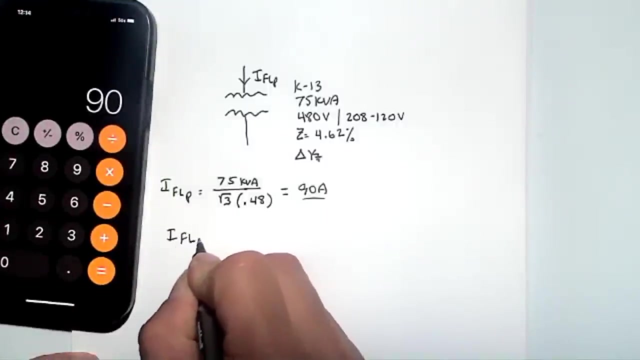 oops, divided by 75 times 1.2 is 90 amps, so we end up with 90 amps, which is that 1.2 multiplier when you have a 480 volt system. now here's the cool thing: if I want to calculate, I full load secondary. I know. 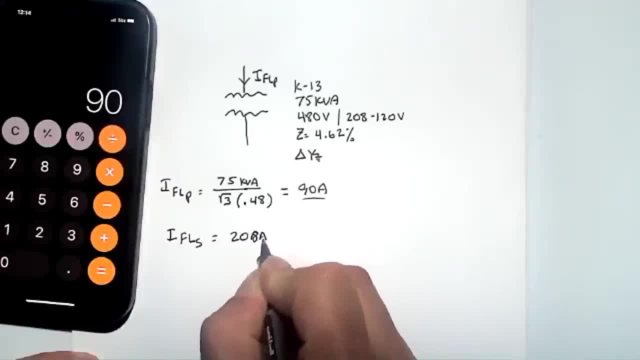 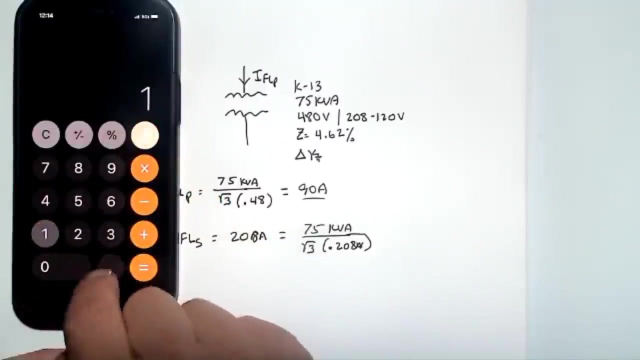 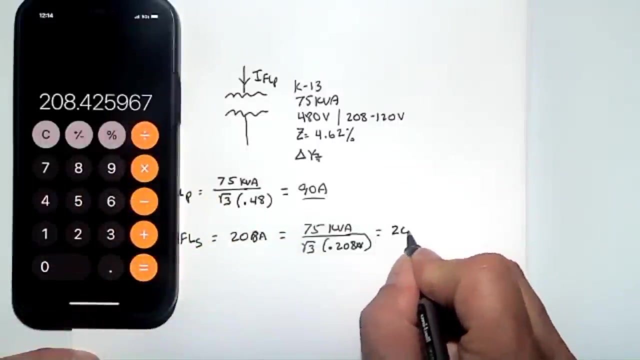 it's 208 amps. how do I know that? well, let's go ahead and multiply it out: 75 k VA divided by the square root of 3, divided by 0.208 volts, or KB, because it's 0.2, and we get 75 divided by 1.73, divided by 0.208, and that works out to be 208 amps. 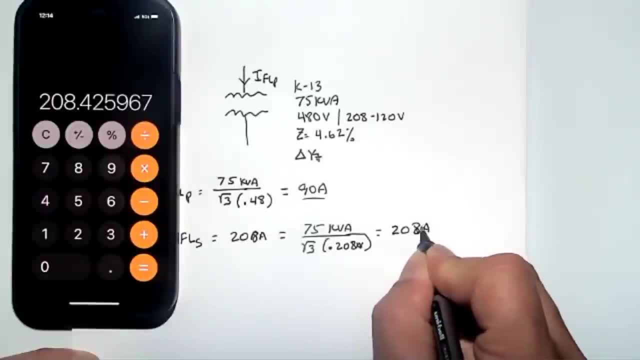 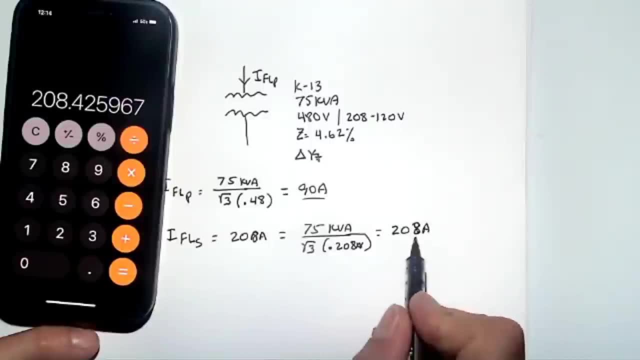 if you can remember that a 75 k VA, 208 Volt transformer gives you 208 amps. so 208 volts and 208 amps, what would be as 750 k VA transformer? well then you just- it's up to you- 208 times 10, or 2080 amps. And again, that's just a side note, Again, rule of thumb, something to 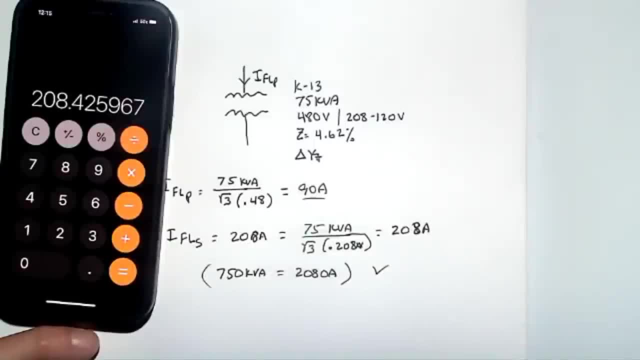 think about something to remember in the back of your mind. And, as I said in the previous page, what if it was 300 kVA? Well, if it was 300 kVA, it's four times this number, So an easy. 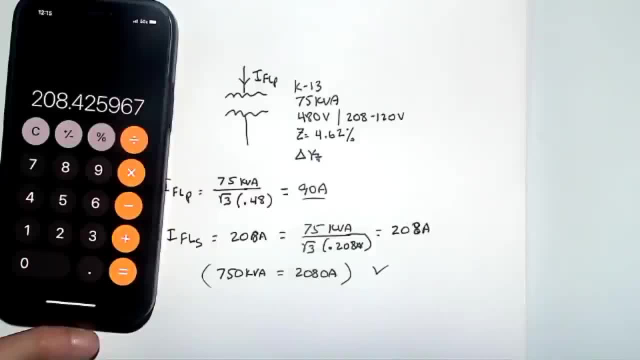 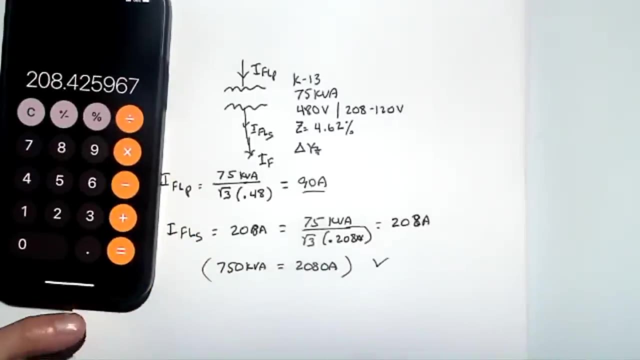 calculation for you to remember to do that Now. so that's full load amps, primary and secondary. What if I want to calculate my fault, current here I fault. So then, earlier I mentioned we just divide the full load amps by the impedance. But really what we're doing is we're calculating. 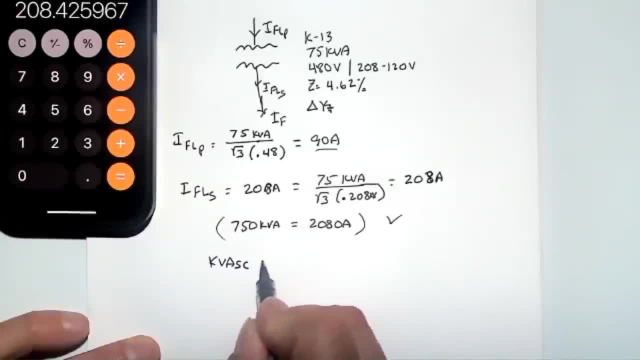 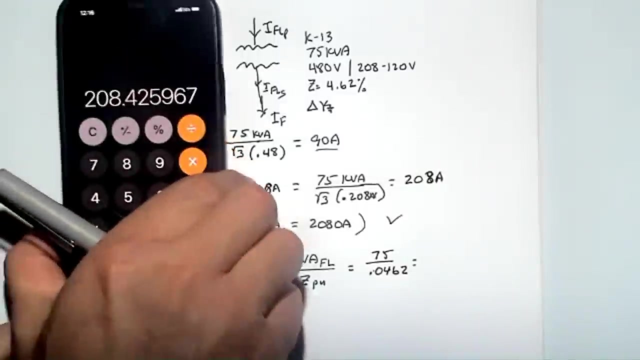 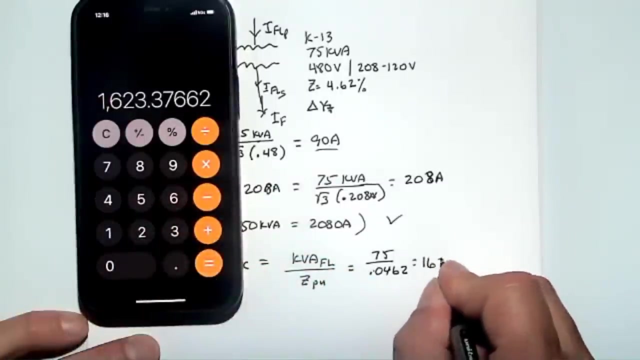 kVA short circuit, And kVA short circuit is kVA full load, which is our rating or rated, divided by the impedance in per unit, And in this case it's 75 divided by 0.0462, which is 75 divided by 0.0462.. That's 1623 kVA. 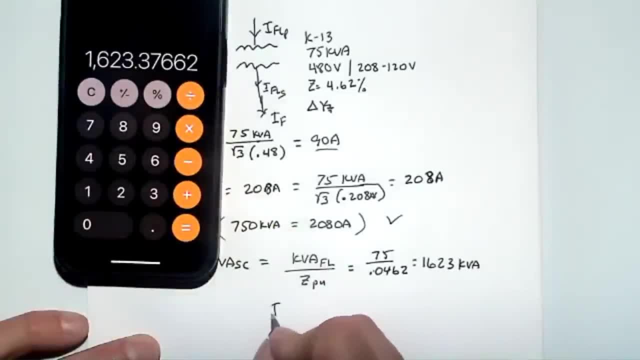 And then that number, if we use our I fault three phase, we're going to take our short circuit and we're going to get a kVA. And we're going to get a kVA And what we're going? KVA, which is 1623, KVA divided by our square root of 3, and divided by our 0.208 volts. 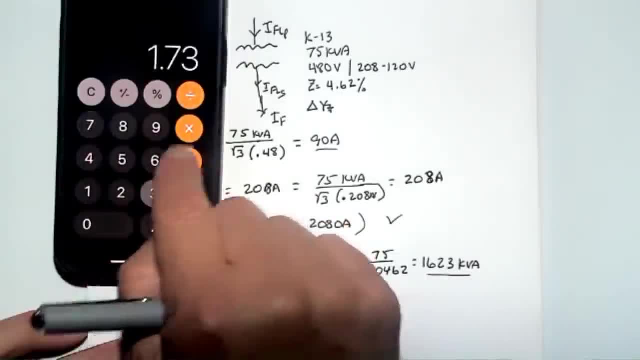 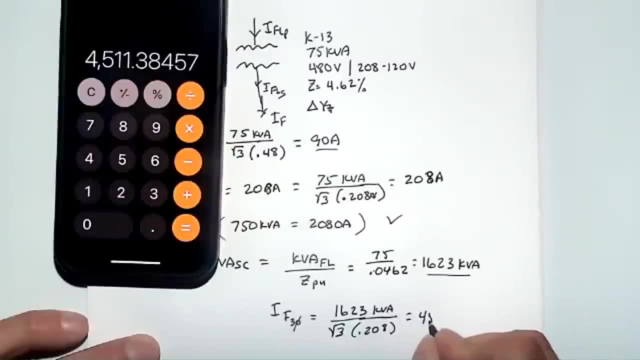 which is 208, and we end up with about 4511 amps of fault current. If I took my number here, that was 208 amps. if I take 208, divide it by 0.0462, I end up with 4502 amps, which is very close to that number. 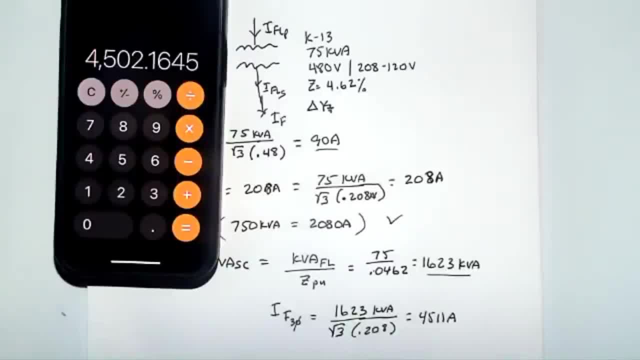 I just was off by basically the square root of 3 factor that works out in there. But anyway, this number, our full load amps and our fault KVA are important, And so you can see that we're using the same equation, you know. 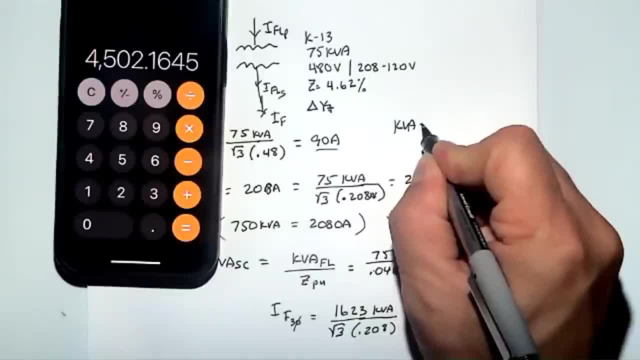 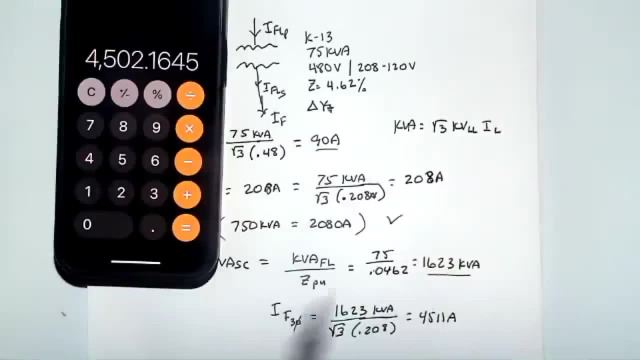 We're using that same equation, which is: KVA equals square root of 3 KV line to line times I line, And if that KVA is our fault- KVA which is what we used here- we can then calculate the fault current here. 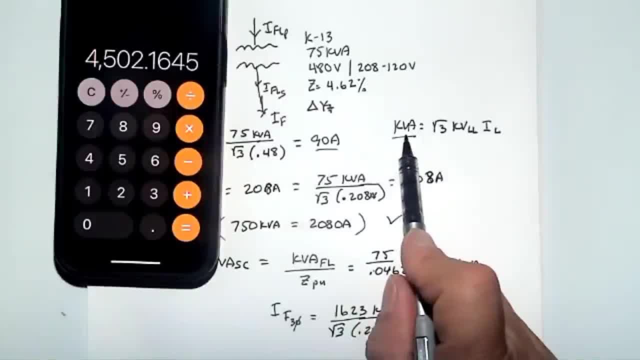 So the equations are all the same. It's either KVA full load or rated, or KVA fault. And the way you get KVA fault is by doing this. KVA fault is divided by the impedance. But again, if you can remember that 208 volt and 208 amps, that's going to come in really. 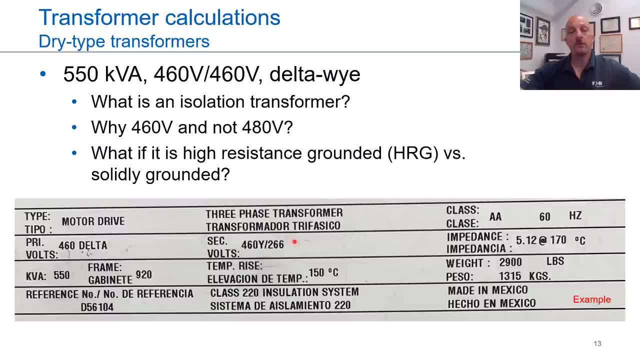 handy. Now this transformer is a little bit unique. This is called an isolation transformer, and again, isolation transformers might be used in front of a motor drive, as is shown here. The interesting thing about isolation is, again, it goes 480 in, or 460 in in this case. 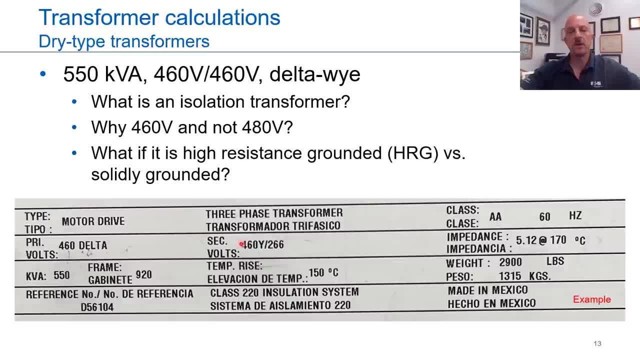 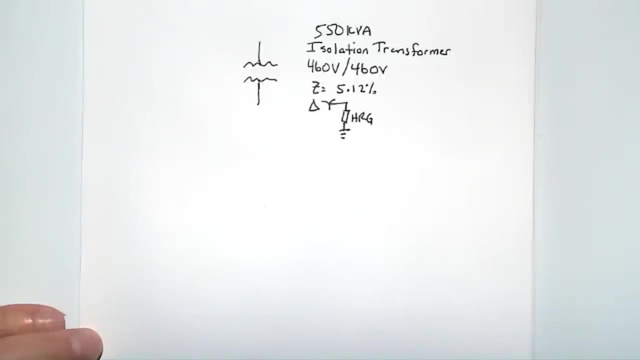 and 460 out. So it's a little bit different. But again it's a little bit different. So it's a little bit different. OK, For the next transformer, we have this unique isolation transformer And again it's 550 KVA, 460 volt rated in, 460 volt rated out. 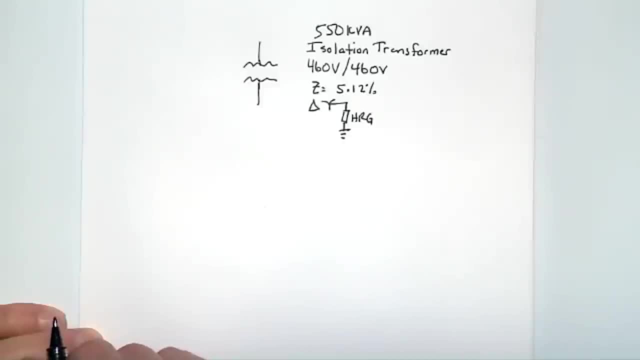 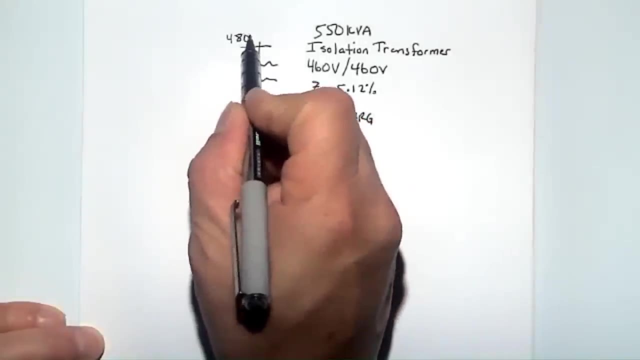 And this is a 550 KVA. So it's a 550 KVA, So it's 5.12% impedance. Now we're probably going to apply this on a 480 volt system. So the bus voltage here is 480 volt and the bus voltage here is 480 volt line to line. 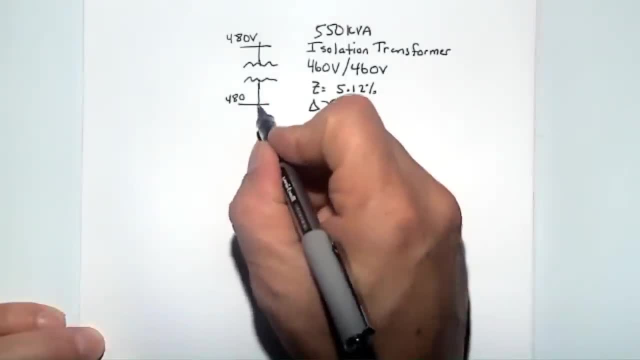 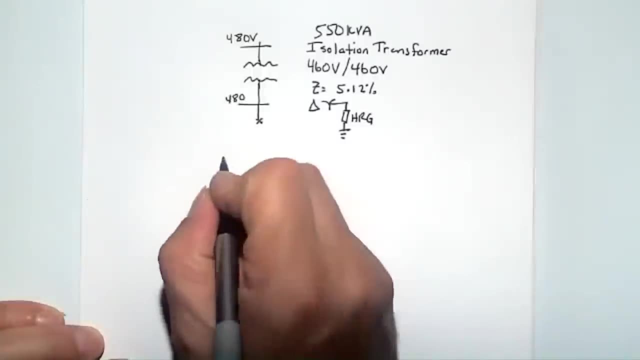 But how are we going to calculate the full load amps on primary and secondary and calculate our fault current? So again, we'll start with our same equation we've been using the whole time here, which we're going to do i full load primary. In this case it's going to be the same as secondary, coincidentally because the voltage is the same. 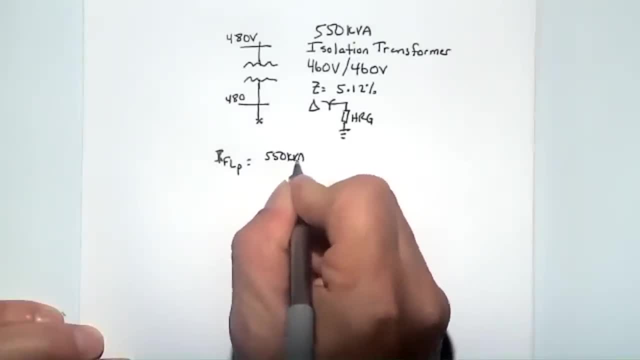 It's going to be 550 kVA divided by square root of 3 kV line to line. Now the tricky part is: do we use the rated value or do we use the actual applied voltage? And what I'm going to tell you here is: let's do it both ways. 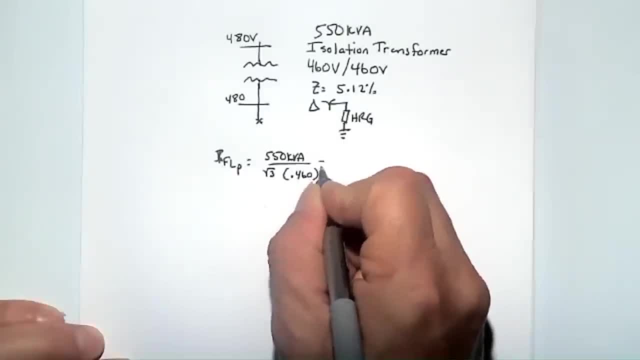 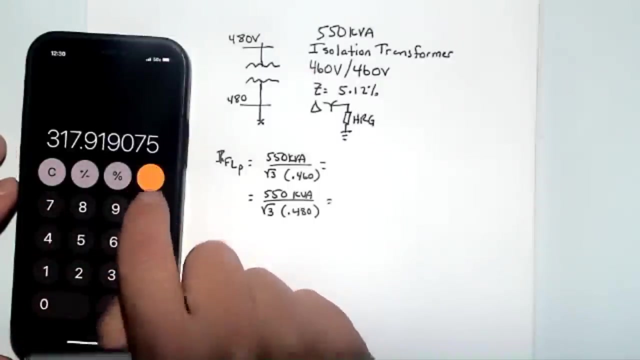 Let's do 460, and then we're going to do the same thing: 550 kVA divided by square root of 3.48.. And let's just see what the difference is there. So 550 divided by 1.73, divided by 0.460.. 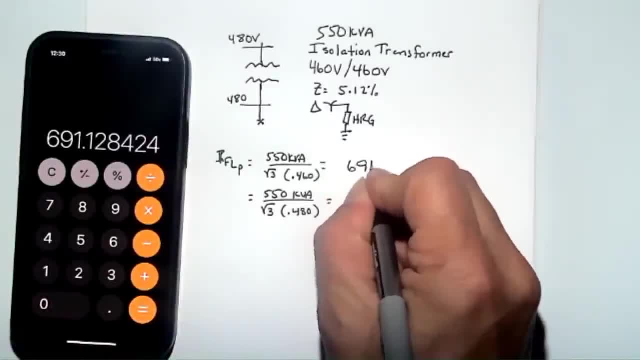 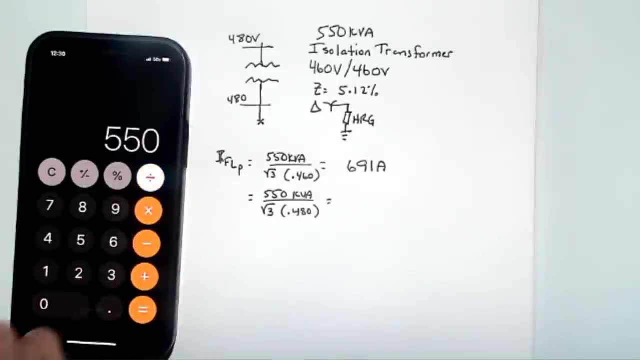 Now that gives us our 691.. If we do the same thing, 550 divided by square root of 3 divided by 480, we get 662 amps. The windings and the actual transformer are designed to handle 691 amps. 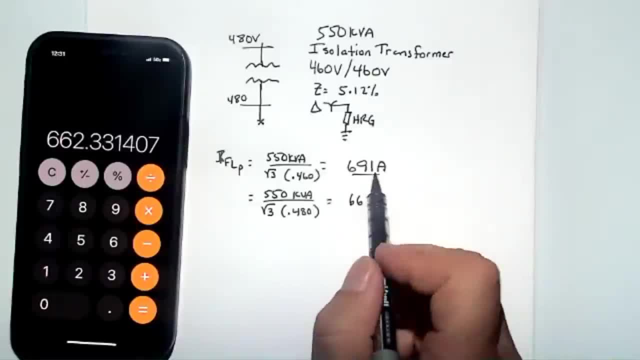 But what you have to remember is kVA is a capacity thing. It's volts and amps together. So if we run at a lower voltage we could go up to that amp Amp Capacity rating. If we run at a higher voltage we're likely going to only want to put up to that many amps through it. 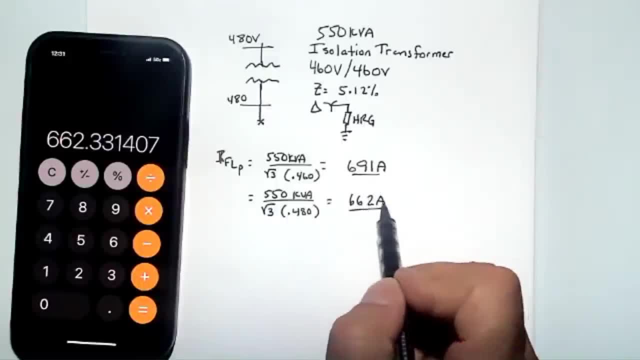 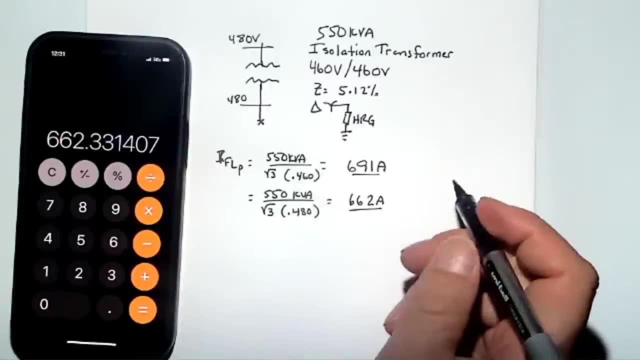 Otherwise we're going to exceed the kVA rating of the transformer. So that's why these two numbers are important to understand. Most of the times you'll see motors rated at 460.. You'll see transformers rated at 460.. A lot of times that's because they're down in the system, where you expect the voltage to run somewhere near that level. 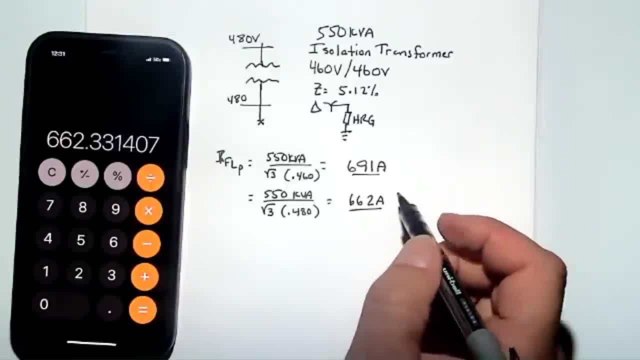 And so to get the full load capacity out of them you can use that 460 volt level. So anyway, Um, you know, again, sizing the breaker, here we might size it for 660.. Well, it's not going to be exactly. that's going to be something less or a factor of that, even a little bit more, depending on how our protection scheme is done. 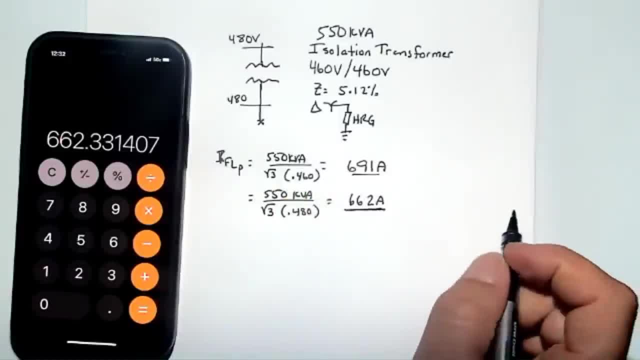 But we're going to typically base it on that because we know we're applying it at 480 volts. Now the fault current I'm going to use that I fault is I'm going to use the short circuit kVA for this one. And the reason I'm going to use the short circuit kVA is because 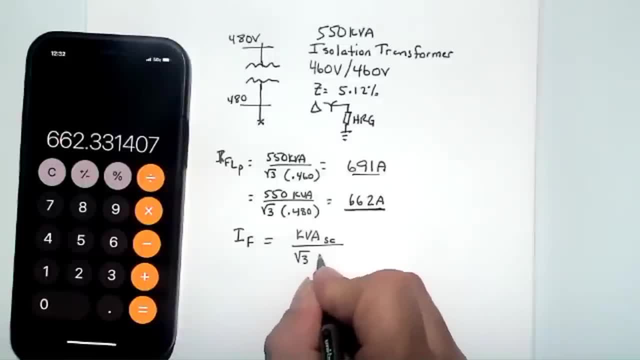 That's based on the rating. So, And then the KV line. Sorry, we're going to divide that by the impedance, So we're going to do 550. But a bit squirted three, but about 0.46. And then that, that's our short circuit kVA divided by our impedance, which is 0.0512.. 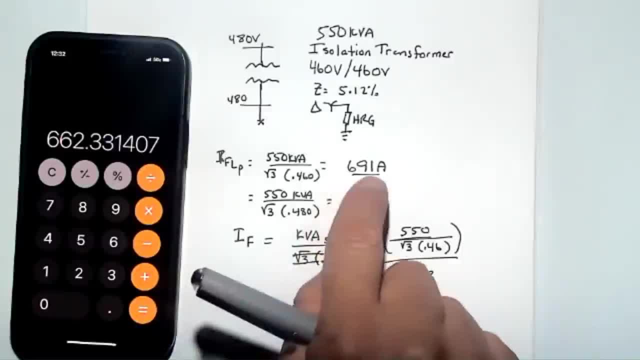 So we get 550 divided by that, That's going to be that number: 690.. 1 divided by 0.0512, and that's going to work out to be 13,496 amps. That's our fault, current And honestly again, these are estimated values. 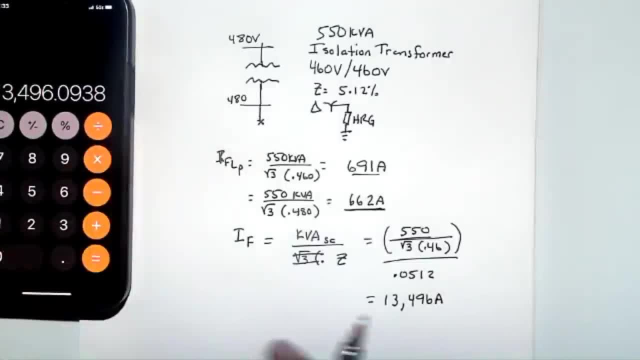 So let's talk about that for a minute. If we have an estimated value of 13,496 amps, is it going to be that? No, absolutely not. It's going to be probably less than that. Why is it going to be less? 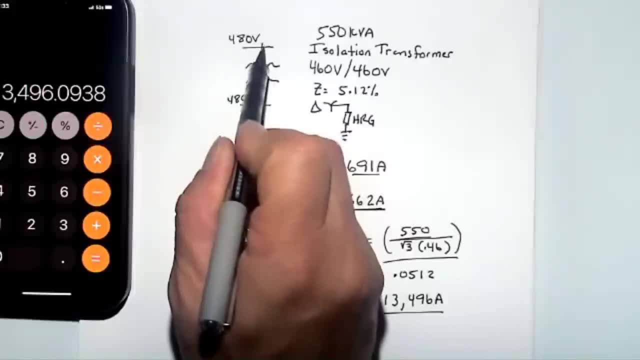 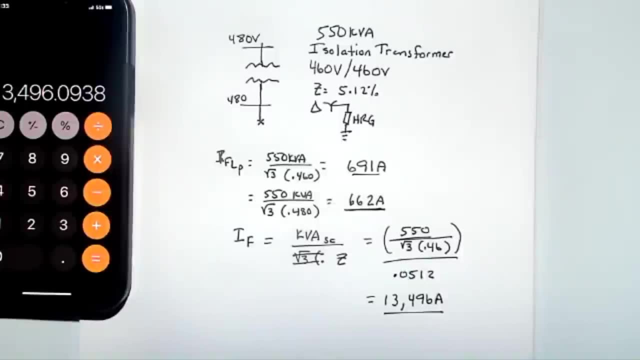 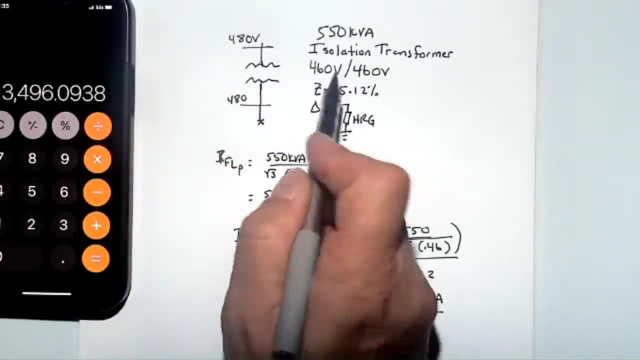 Because, remember, we Ignored our primary impedance of our source above that. So in a lot of times in this case, especially where you use an isolation transformer, the transformer upstream of this might not be very small or very big. In fact, it might be closer to the range of this transformer. 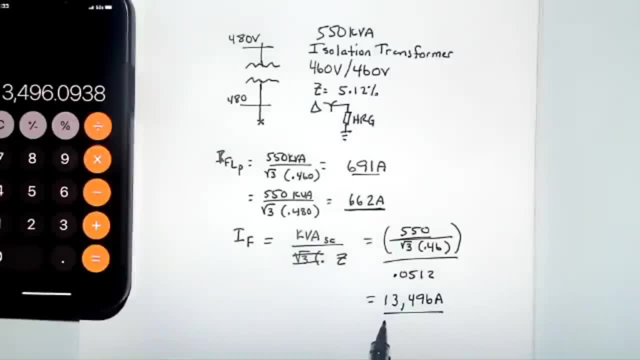 So we do have to take that into account, sometimes in a more formal study. But again it's going to knock that number down. Also, if we have motor contribution here, That motor contribution Could increase the fault current for a short period of time during fault conditions. 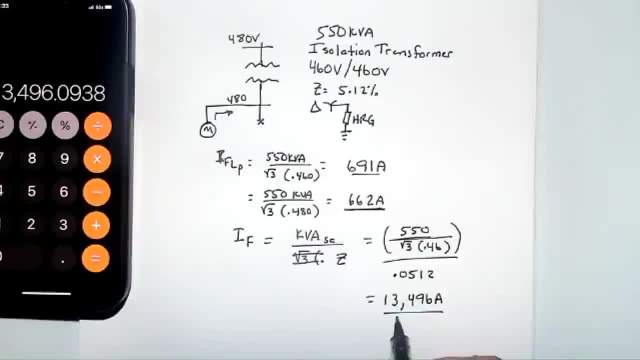 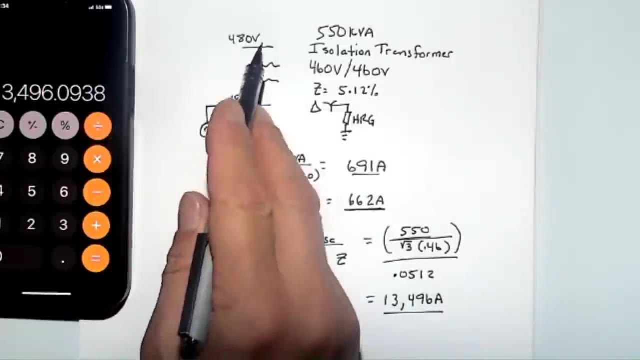 So again, these numbers are estimates. If that number was, you know, 13,500 amps and you were putting 35 K a breakers in on this system, it's not going to matter there. It's so different that it doesn't matter. if this number was 34,000 amps and we weren't exactly sure what the impedance up here was going to do and the motor contribution was going to do, I would be much more concerned. 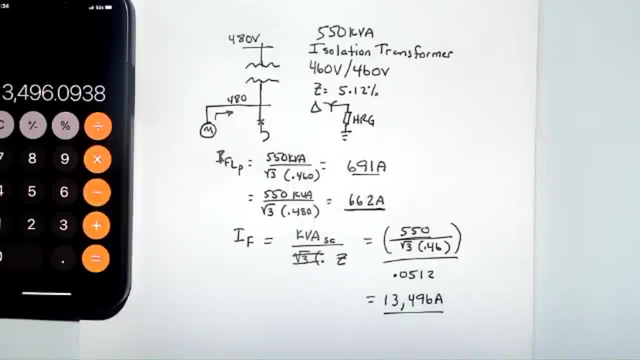 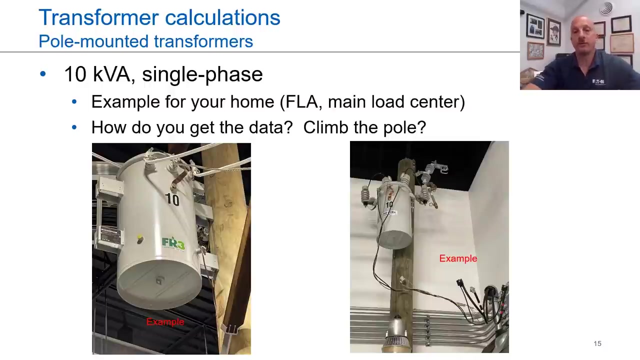 So, again using These estimated calculations, we can go through that and figure it out. Okay, now, moving on to a different type of transformer. These are pole mounted transformers, and this is actually the kind of transformer that's going to be out in front of your house. 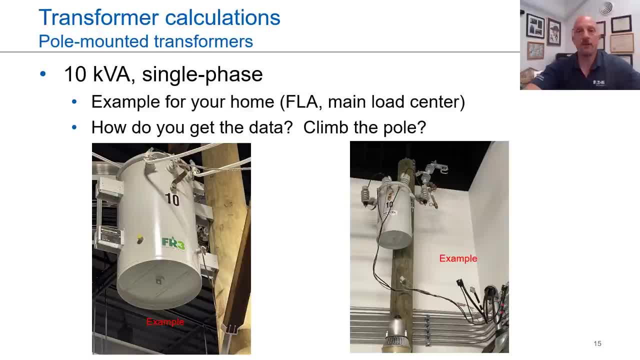 For example, you either have this type of transformer or you have one that's pad mounted, but in the case of of the size, it's usually 10 KVA, 25 KVA, and that's what we see on this one: 10 KVA. 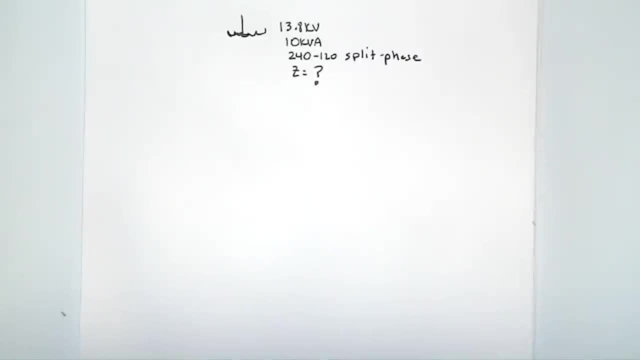 That's the number that's written on the side of the transformer. Okay, now, this is a fun one, because This is what's outside of your house and you want to think a little bit about what's the full load amps on the primary and secondary on this transformer. 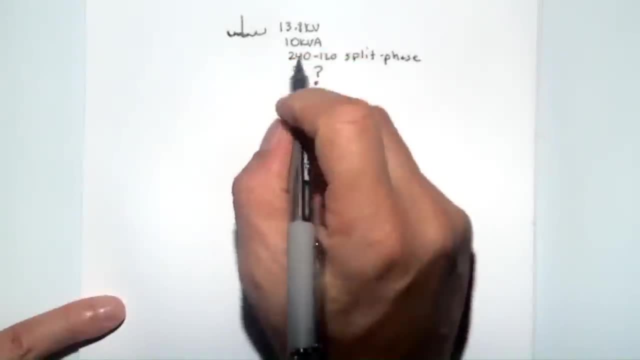 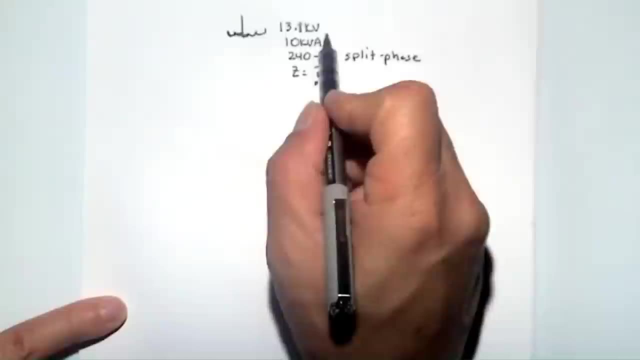 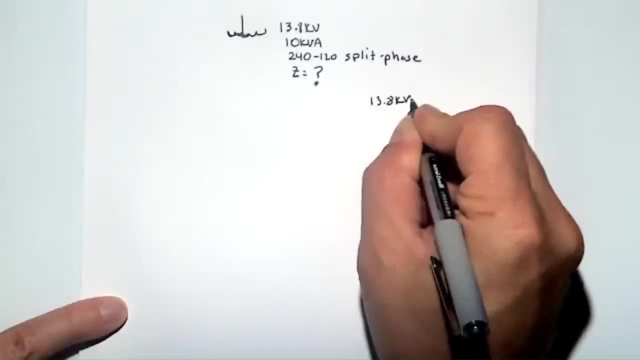 I didn't draw the secondary here because I want to show you something. This is 13.8, typically line to line, or it could be line to neutral, which is this number divided by the square root of three. And so if we knew the primary voltage, let's say 13.8 KV, and we divide by the square root of three, we would get 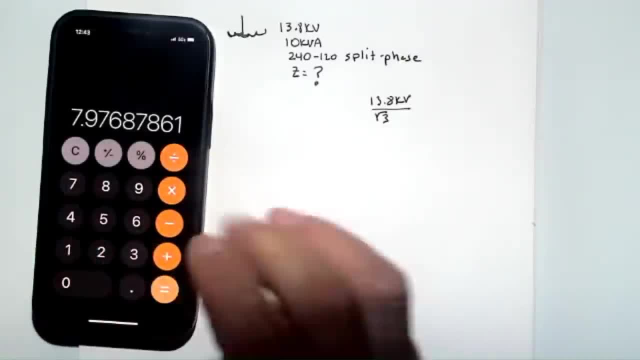 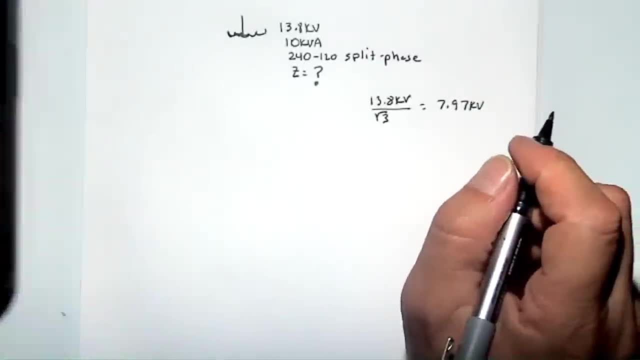 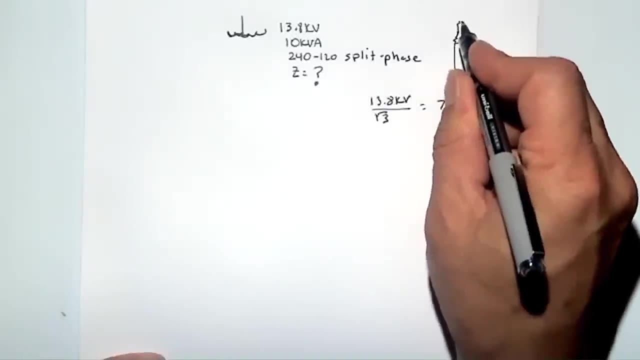 13.8, 7.97, so that would be our KV on the on the primary side. Okay, but the way you can tell that is if you look at the transformer, and the transformer has two bushings that are about the same size. typically they feed them line to line. 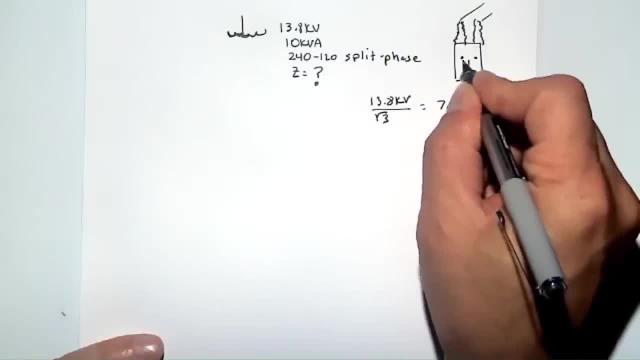 You'll see your secondary bushings coming out of the secondary here and the 240 volt and the center tap. Okay, You'll see your secondary bushings coming out of the secondary here and the 240 volt and the center tap filtration taking about neutral grounded. 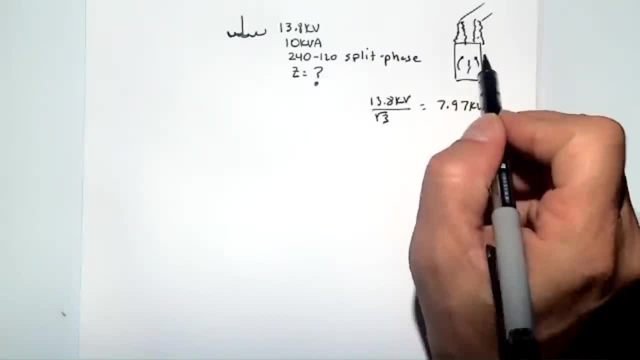 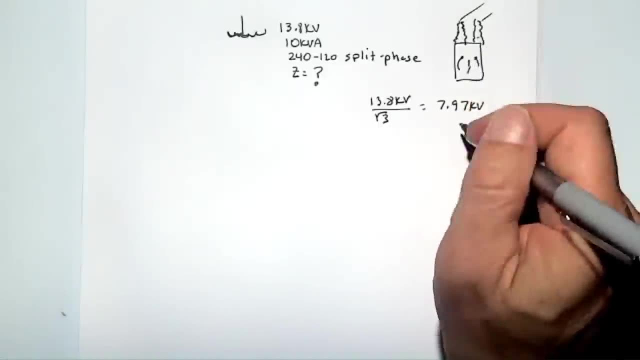 Neutral is coming off there. If there's only one tall bushing and one short bushing, then a lot of times just line to neutral. They do that because of the cost. of the bushing obviously adds to the many, many, many transformers that are out there. 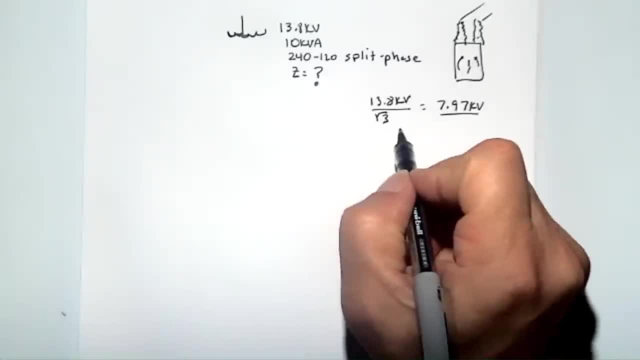 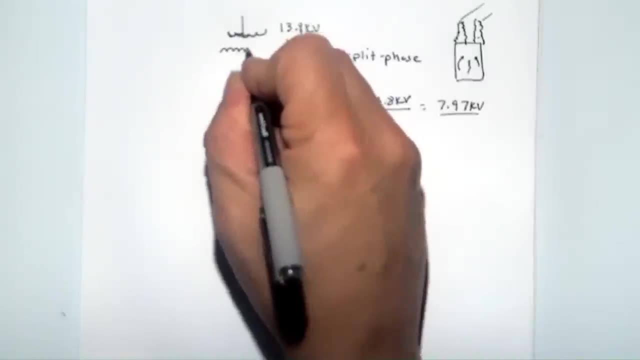 So sometimes they apply on that line to neutral rating or, in this case, line ground, and sometimes apply that line to line. But we're gonna just say it's line to line. for the secondary, The transformer looks like this This: two windings coming off of there. 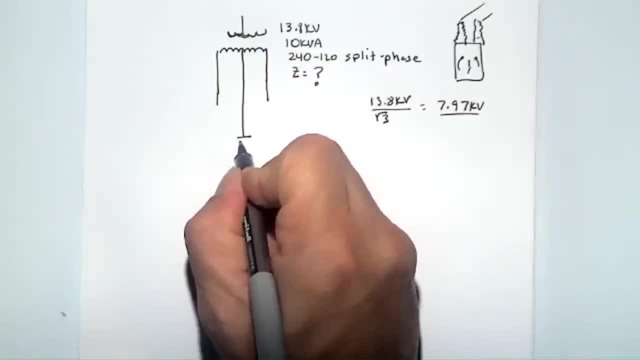 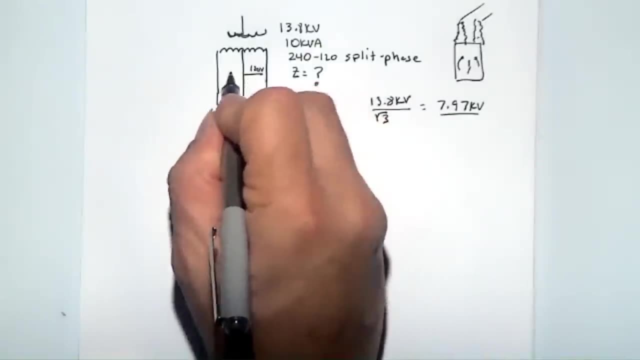 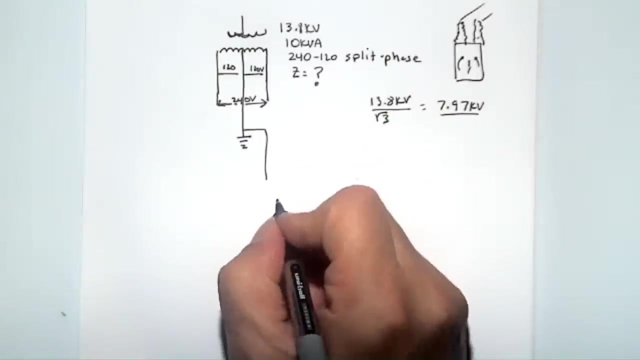 120 volt to a grounded neutral. so the neutral is grounded, it's brought into your home and so it's 120 volt here, 120 volt here and then 240 volt from here to here. so what are we going to calculate? the breaker that's in your home typically is a two pole breaker that's connected on that 240 volt. 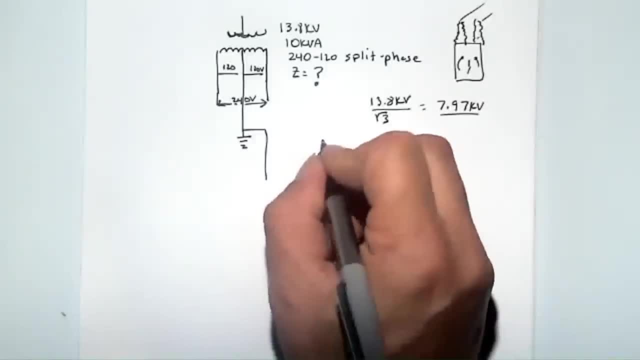 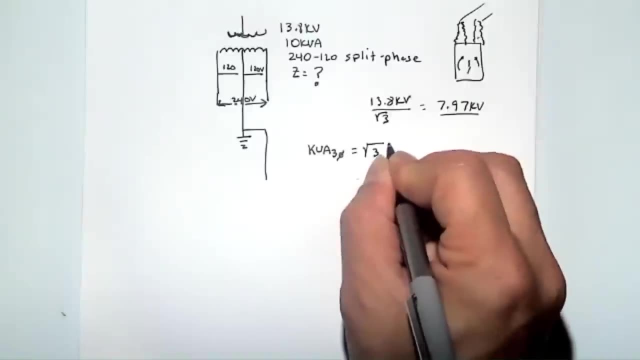 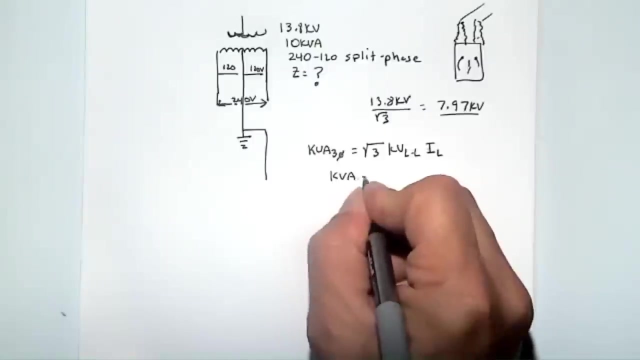 so we're going to calculate based on the 240 volt. so instead of using that, KVA 3 phase is equal to square root of 3 AV by the line times I line, we're just going to say KVA equals KV times current. in this case we know the KVA which is written on the side of the transformer is 10 KVA and then 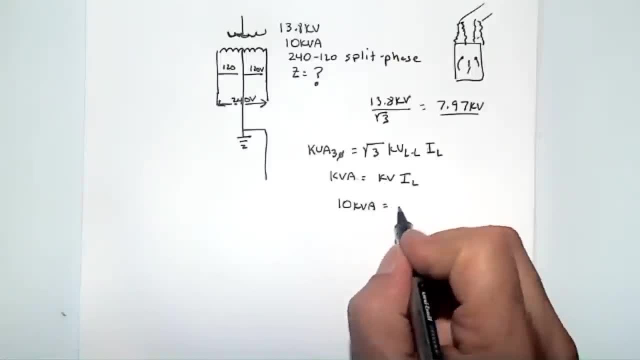 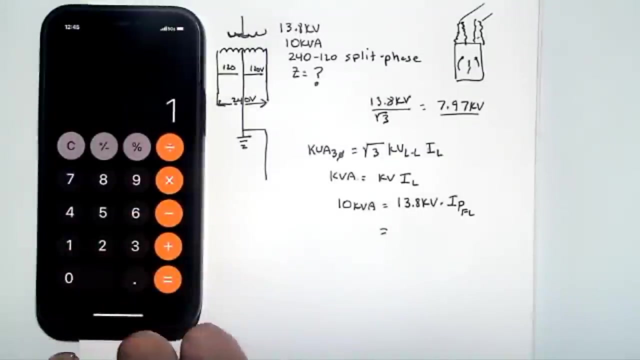 the voltage is either going to be 13.8, we said on the primary, that'll give us our I primary full load, or- and so let's just calculate that out- um. third, so we'd have 10 KVA. so I equals 10 divided by um. 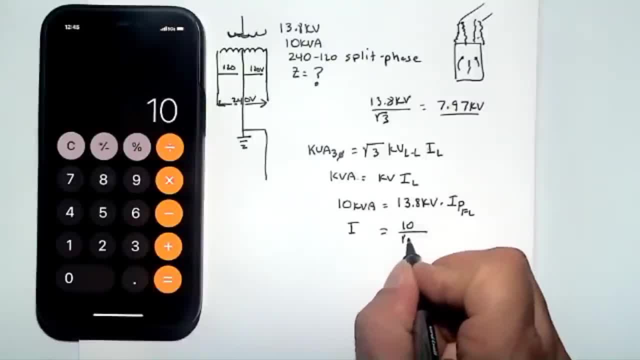 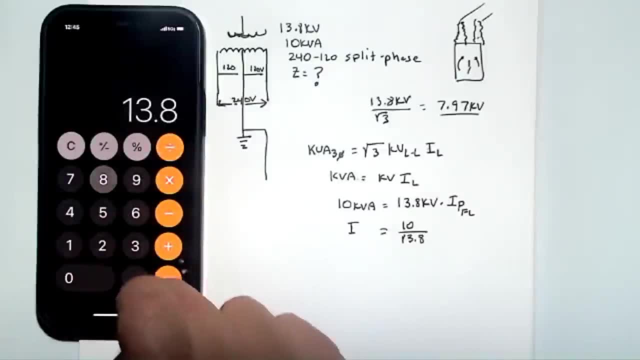 yeah, I want to use my square root of three in there. um, I divided by 13.8, so 13.8, so 10 divided by 13.8 and really right away we can see that's less than one amp, so 0.725 amps. so that's what's kind of cool. if you think about it, they could use almost like an. 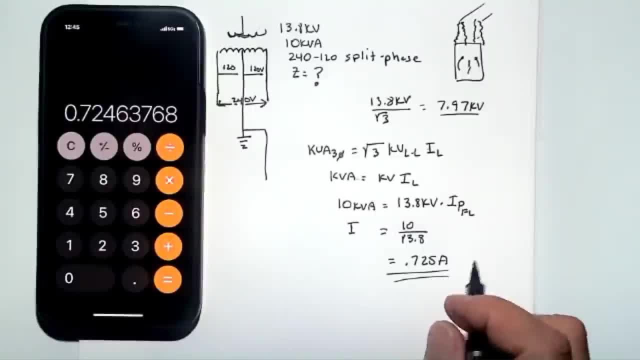 Ethernet cable to feed your house. it's very, very low gauge wire, but that's why they can use like a 10 or 12 gauge wire, uninsulated in the air, just feeding the primary, and you're going to see that that wire is small. it doesn't even need to be as big as it is. 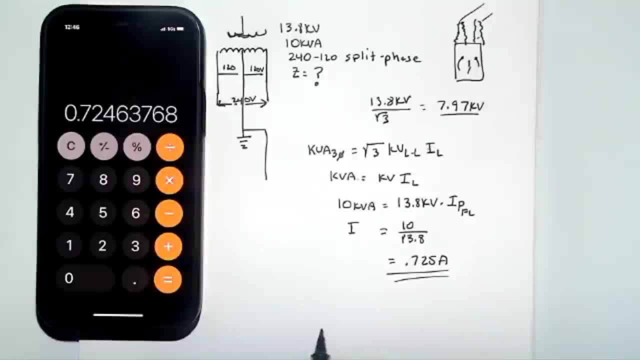 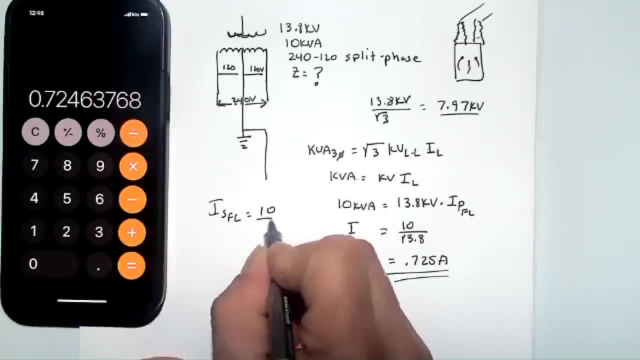 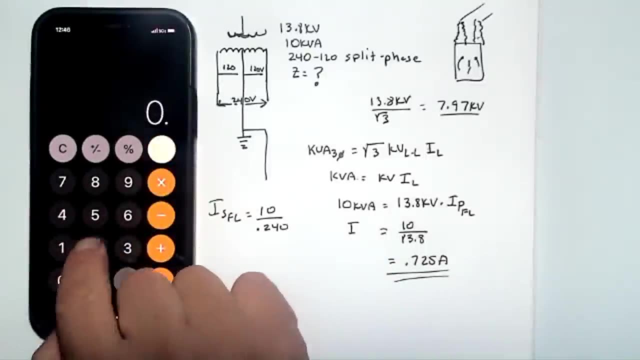 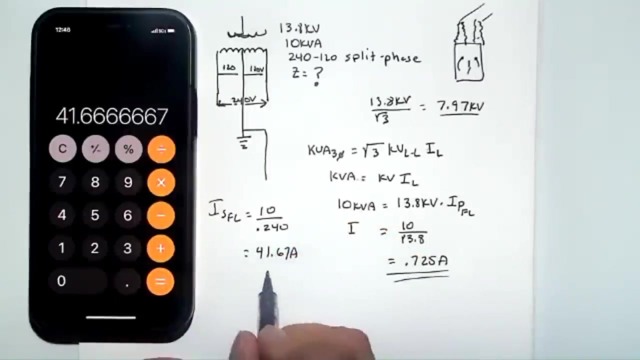 because you have less than an amp on the primary. the other part about this is cool is if you look at the secondary is secondary full load. we have 10KVA divided by 240, so divided by 0.24, then we get about 42 amps, 41.67 amps, so for obvious reasons then we put 200 amp. panels in, or we put multiple 200 amp panels in. then we're going to need to have towel towels in, and then we put another three, which is probably less than so. this are only heavy and more expensive. so 41 more. now here's our recommentary problem. I imagine somebody said: oh, we need to build one O cucumbers to first extract the� 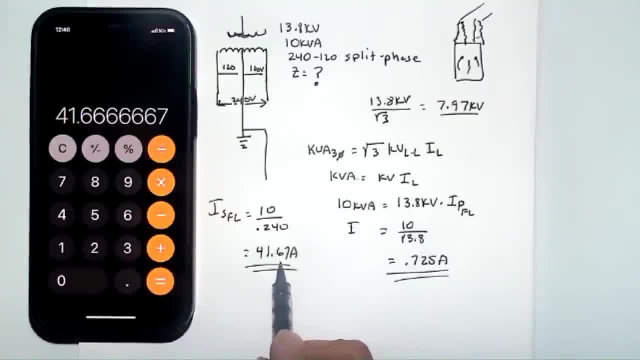 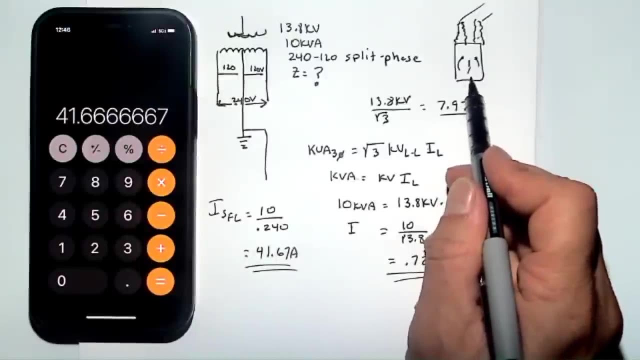 in our house. right, what's cool about this thing? you think about it. our panel in our house is 200 amp, but we can only supply 41 amps or 42 amps from the utility transformer, based on its capacity. but the utilities actually will push these. push these transformers up even more and they'll let you draw. 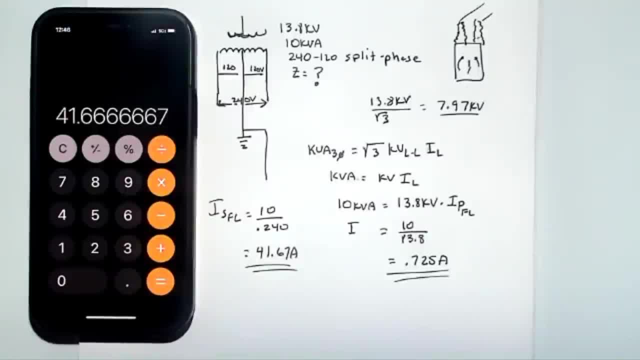 through maybe almost two times the normal KVA, because they'll just let them blow off the poles. but reality of it is you're never going to approach the 200 amp panel that's in your house, so why do we put 200 amp services in? well, we 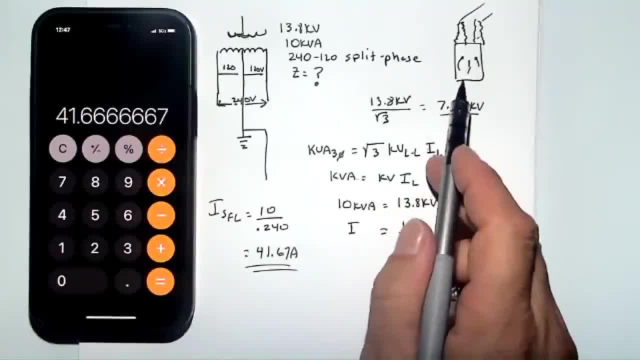 don't know. if they have a 10 kVA Transformer, they may upgrade that to a- you know, 25 kVA transformer, or maybe 50 kVA, so we don't know. and so the capacity of the service coming into your house is what really dictates your. 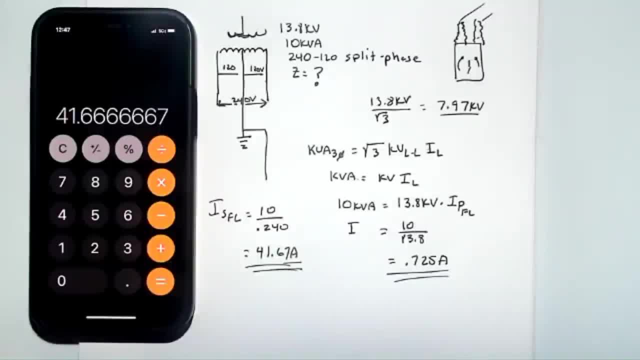 breaker and not necessarily the full load amps in this case. now, as far as the bulk current, let's just take that number, 42 amps, and div eternal that by our impedance. What is our impedance for this kind of transformer? Said it earlier, it's going to be between 2 and 3 percent. 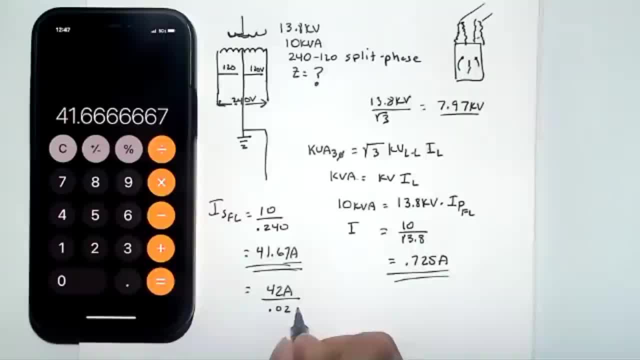 so let's just use 0.0.. I think the one we showed was 2.4 percent. so take that number, divide it by 0.024, and we get 1,736 amps. Typically in our homes we're using 10kA breakers. 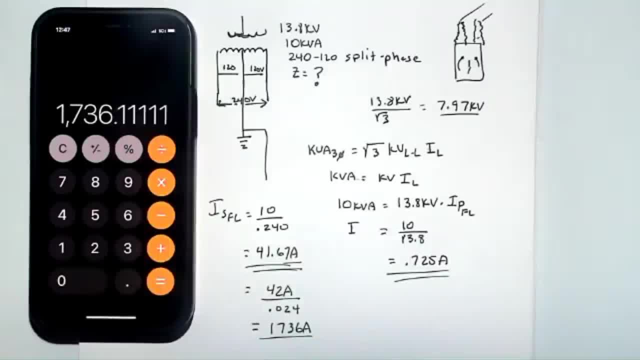 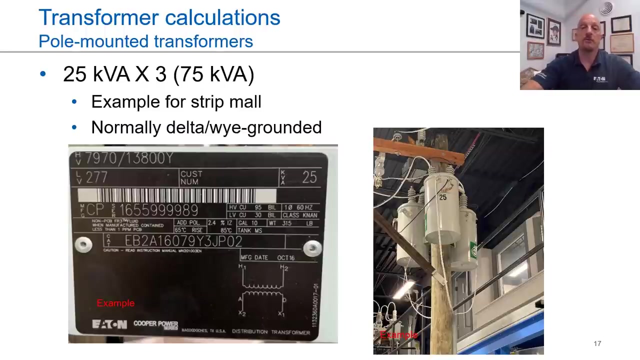 so this is well within that range. Now, let's take a look at this transformer or the sets that we are going to take. So let's take a look at this transformer or the sets that we are going to take. 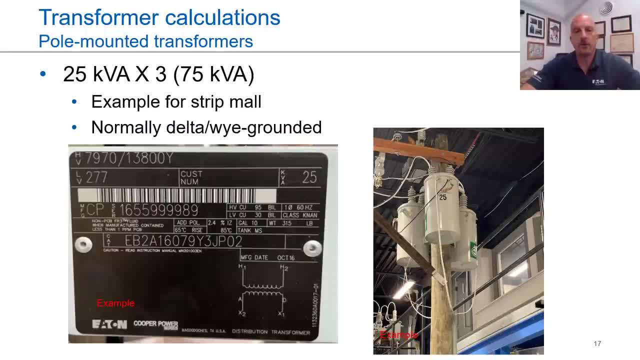 So let's take a look at this transformer of transformers. These are three pole-mounted transformers, Again oil-filled or liquid-filled. These ones happen to have FR3 in them, 25 kVA, that's what the 25 is on there And actually, 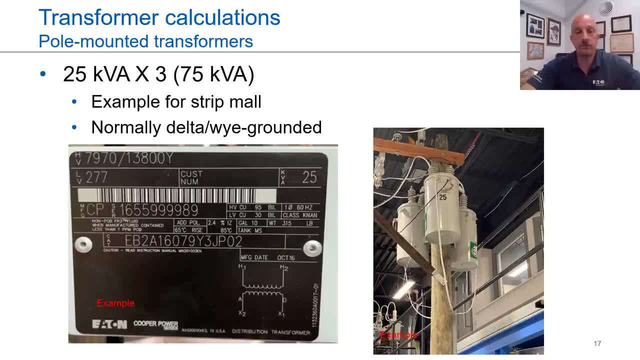 if you get up close and again, if I you know up earlier I was showing you on from the bridge there. If I looked at that nameplate, I could actually see the nameplate and the impedance of this transformer. In this case it's 2.4%. What's interesting about pole-mounted transformers is 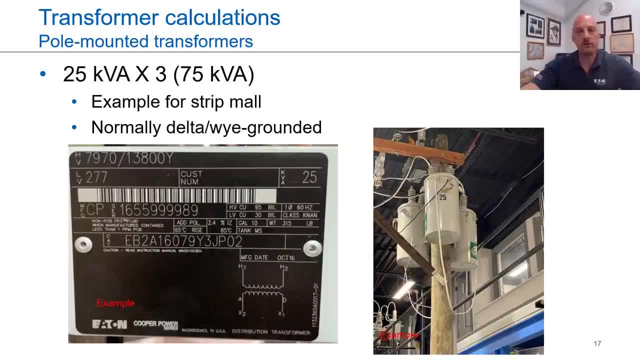 they do have a lower impedance. So we made an assumption earlier. if you didn't know the transformer impedance, you could say 5.75%. But in this case, if you don't know the impedance of a pole-mounted transformer and you guess that high, guess what you're going to do. You're going. 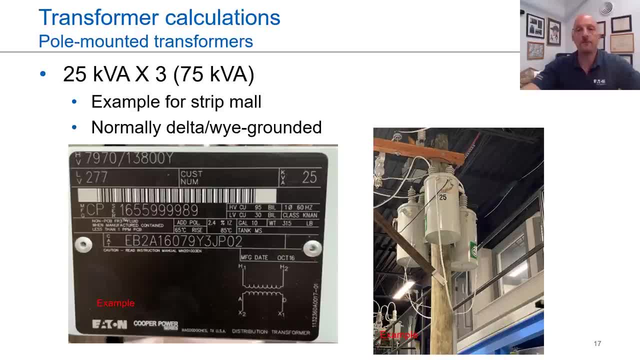 to influence your fault current calculation. So it's important that you don't overestimate the impedance of a pole-top transformer, And so, if I don't know the value, I might even guess 2% for that one. So 2 to 3% is a typical number. Okay, now that we're getting pretty comfortable. 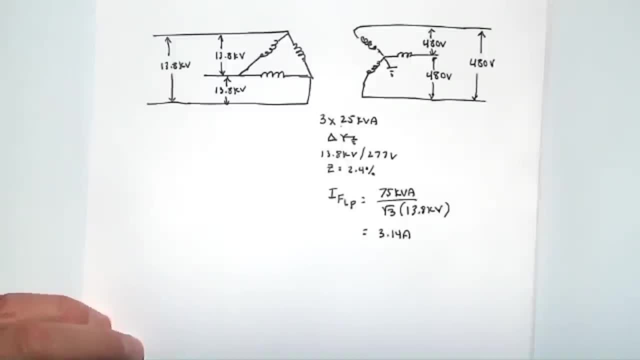 with these calculations, let's move on to the next one. So we're going to look at the another little wrench in the plans. We're going to say there's three single-phase transformers, pole-mounted, and those transformers are connected in delta Y as shown here, delta Y. So this: 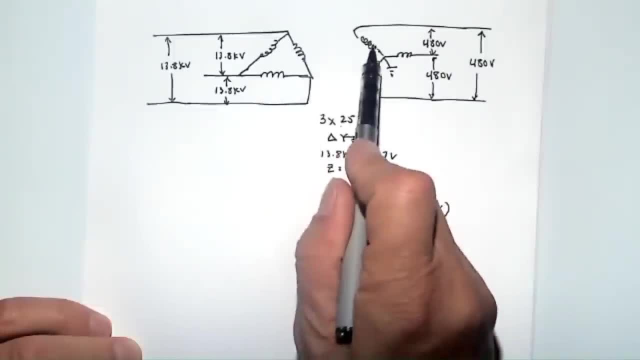 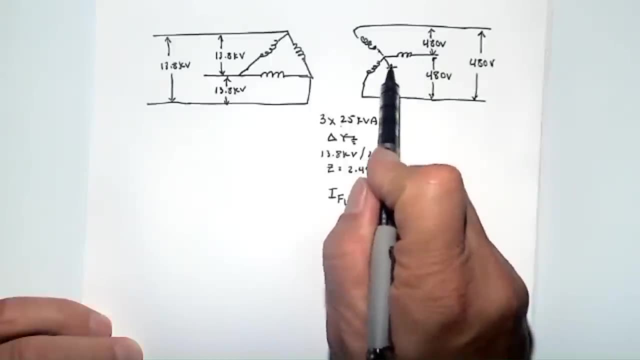 winding corresponds to that one, this one to this one and this one to that one. Each winding, each transformer is rated 13.8 kV line-to-line. 277 volt line-to-neutral. So here's our neutral point on the secondary of the transformer: 480 volt line-to-line. on the secondary. 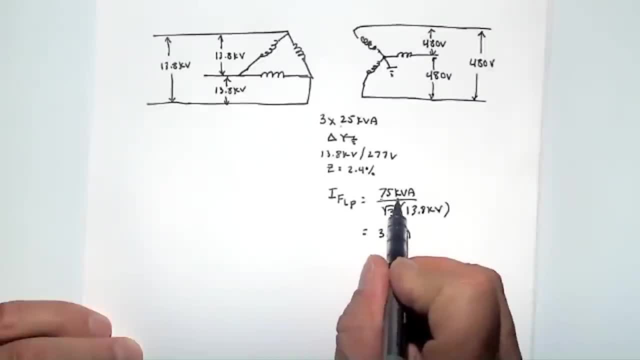 So our difference in our calculation really is: we're going to take this 3 times 25 kVA and make it a 75 kVA transformer. There's our square root of 3 and 13.8 kV. That works out to be about 3. 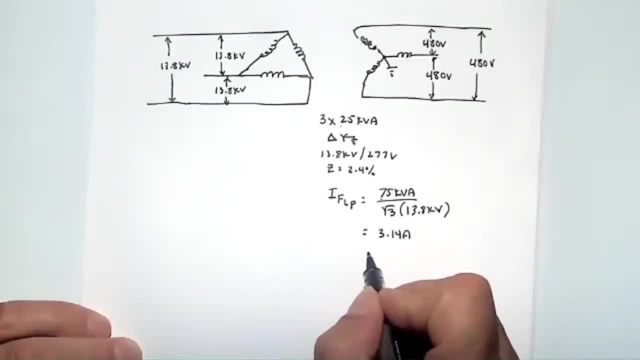 amps. So again, even though the wire size could be very, very small, in this case we only need about 3 amps on the secondary, on the primary And on the secondary. again, we already know what that's going to be: It's going to be 75 times 1.2, or about 98. 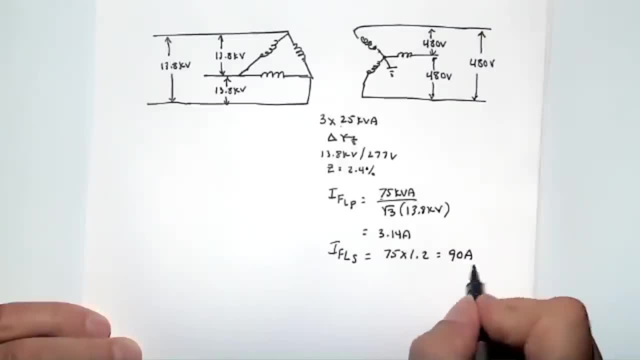 So, again, we're starting to become more and more comfortable with that. Why is that? Because we're a 480 volt system. Our multiplier on our kVA is about 1.2, so we're at about 90 amps. 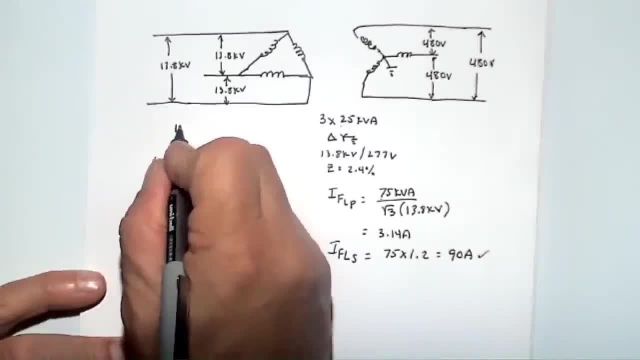 Okay now why am I using 13.8 kV? I could use 12.47 kV for medium voltage. I could use 13.2 kV, I could use 13.8.. I may even go as high as 34.5 kV for medium voltage, and I might go as low as. 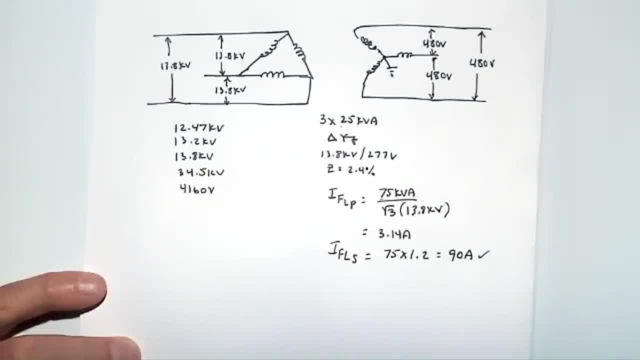 4.60 volts or 4.16 kV, But anyway, or even 2.4 kV. But the point is, I'm trying to be consistent, so I'm using the 13.8 for this calculation. So again you can see what our. 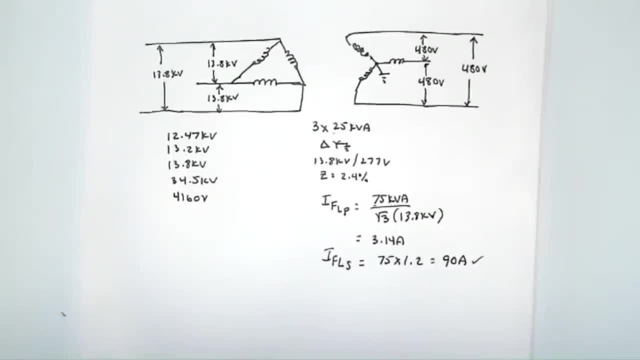 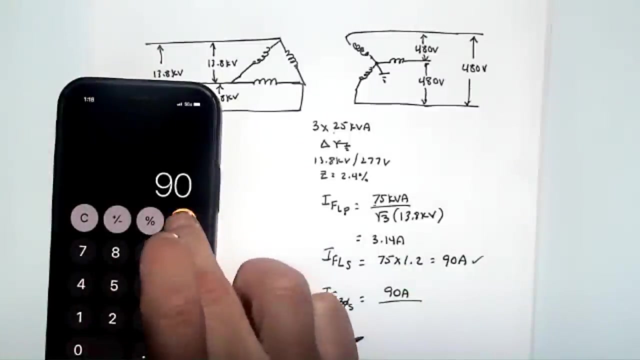 load currents are going to be primary and secondary. Now let's calculate our fault current. So I fault three phase on. the secondary is going to be 90 amps divided by our impedance, And again, the impedance for these guys is typically pretty small, So we're going to use, you know, the number on the nameplate in. 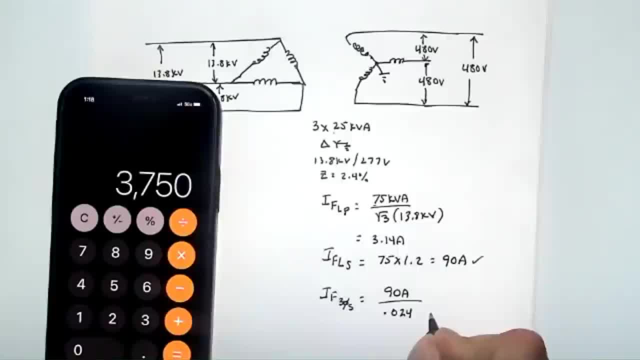 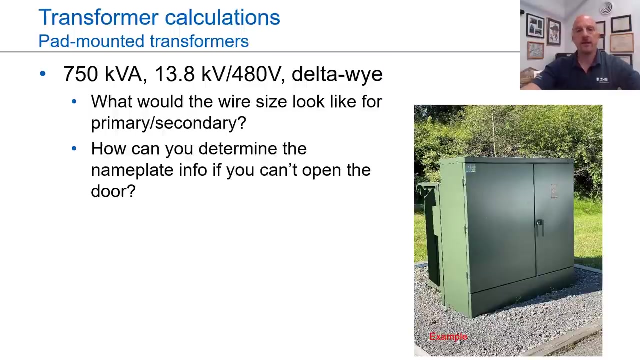 this one, 024 per unit, or 2.4 percent, and that works out to 3750 amps of fault current. So this transformer is 750 kVA delta Y, 13.8 kV to 480 volts. Now, what's unique about these? 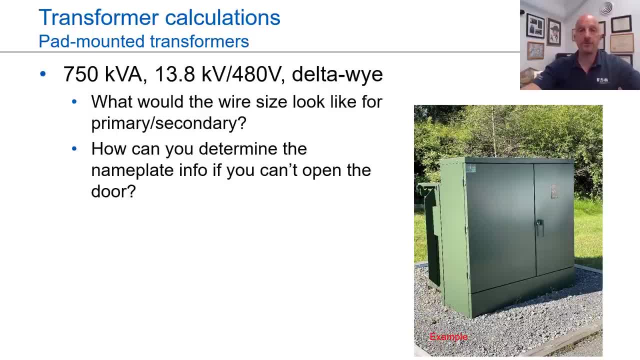 pad-mounted transformers that you might find out in front of a building, just like the one I'm in today here, is that you can't really tell a lot of times what size they are and you don't usually get to access the nameplate because the nameplate might be behind one of those two doors. So you 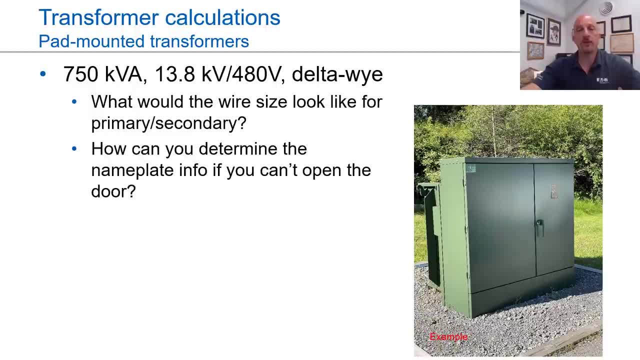 might have to rely on numbers that are on the outside of the transformer and you might have to rely on numbers that are on the inside of the transformer, But most likely you want to talk to the utility company and get that information from them, especially as it relates to impedance. 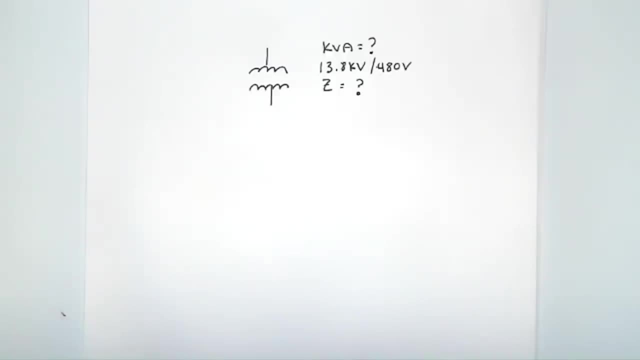 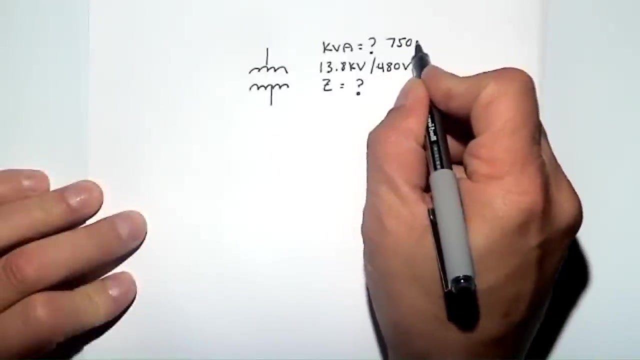 and kVA size. So if you have a pad-mounted transformer like this one, how do we know what the ratings are for it? As I mentioned, you can't get inside the door. So a lot of times we'll talk to the utility company and let's say we determine that the kVA rating either with some numbers. 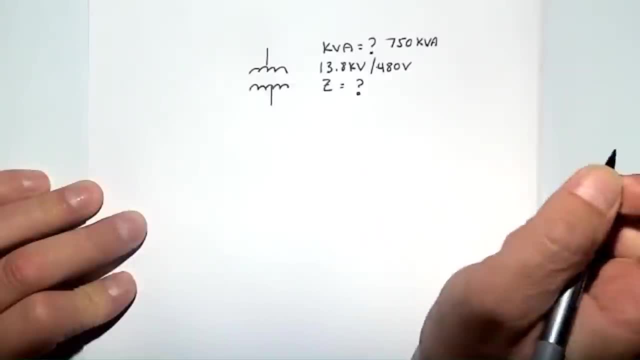 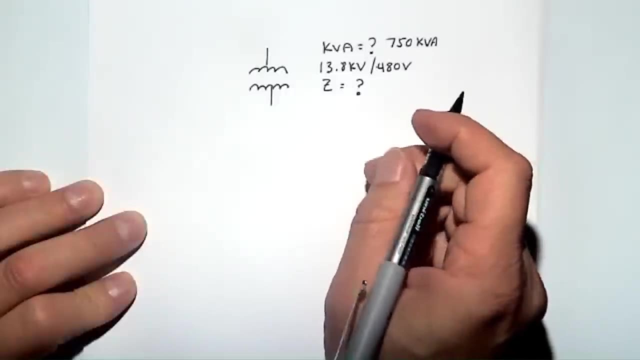 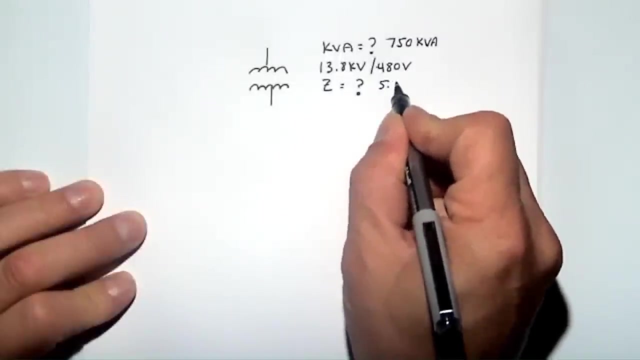 written on the transformer was 750 kVA and we couldn't get a hold of the number on the transformer or we couldn't get a hold of the utility company. So what are we going to guess? Well, honestly, it's difficult to guess at transformer impedances, but in many cases, if we don't know the answer, 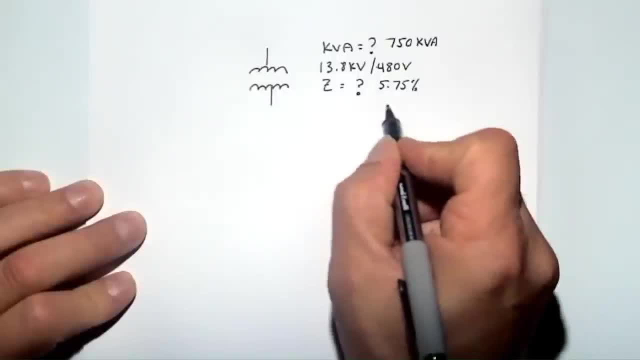 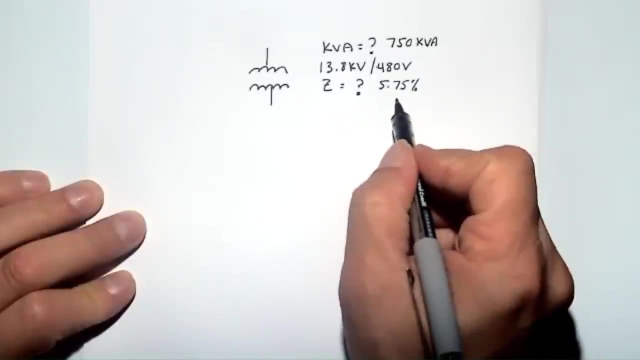 the traditional impedance to use is 5.75%. I will tell you, though, that, depending on the size of the transformer, this is not a great number. for much larger transformers- And again we mentioned pole-mounted transformers- is not appropriate So for kind of medium size and smaller dry-type. 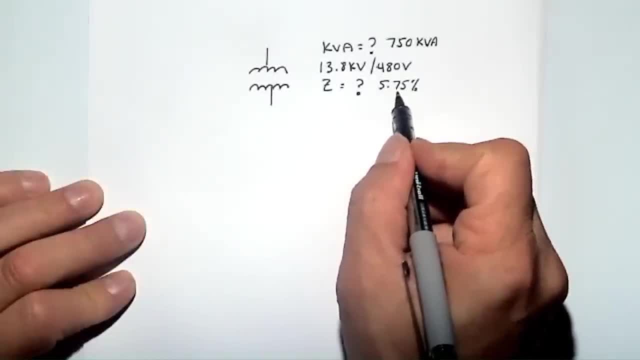 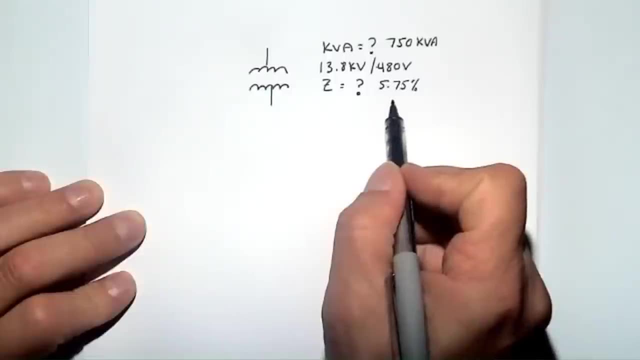 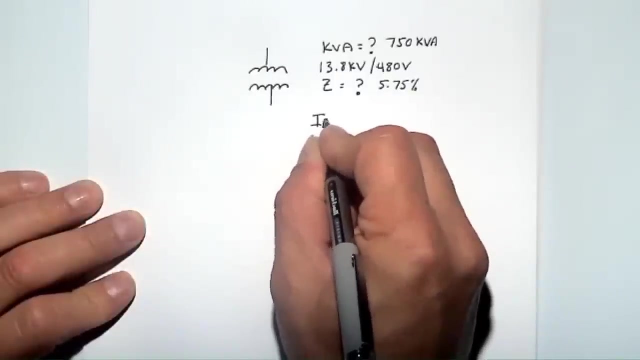 transformers. if you don't know, you can use that number. But again, using a bigger number gives you less fault current. So we want to be careful we're not overestimating impedance For this liquid-filled transformer. we're going to use 5.75.. But anyway, so let's say we figure out. I full load on the primary. 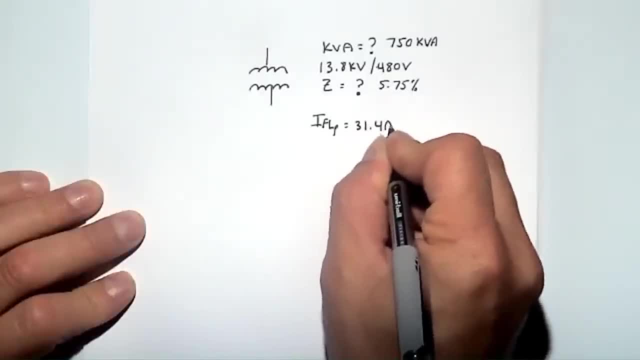 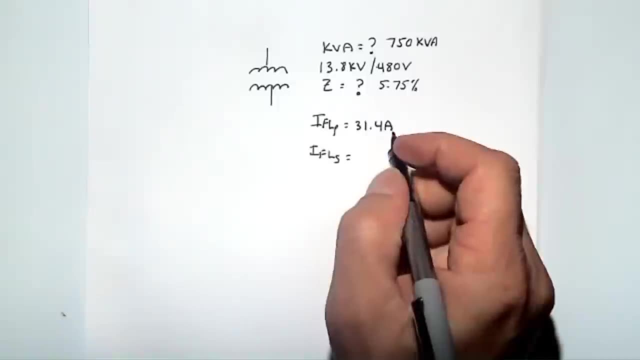 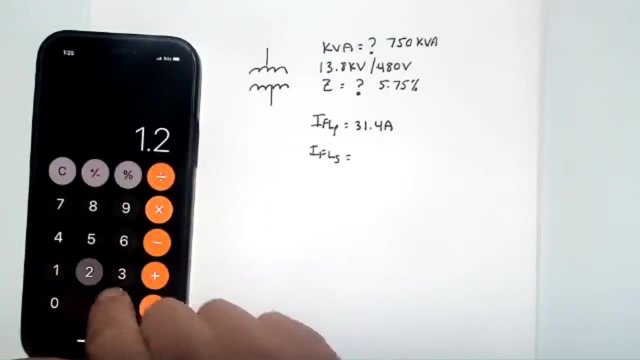 is about 31.4 amps and I full load on the secondary and I know what you're going to do. You're going to take that 750. And do what You're going to take that 750 and say 750 times 1.2, and you come up with 900 amps, right? 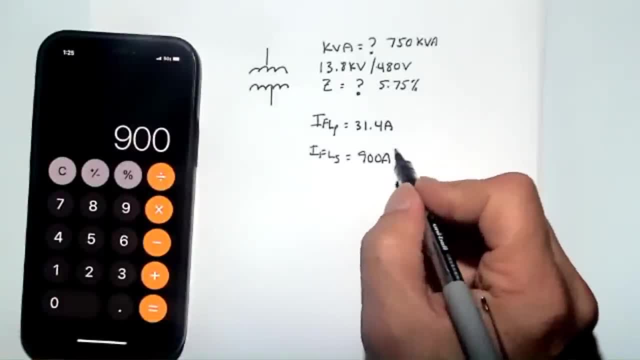 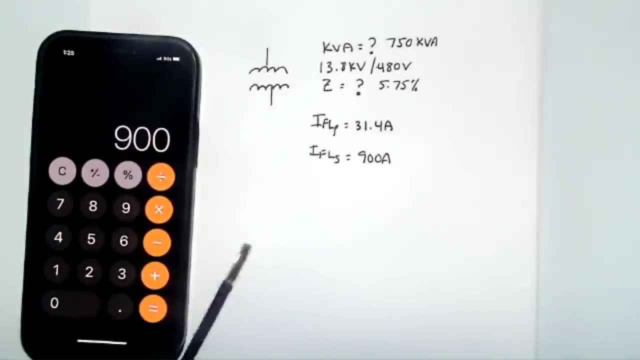 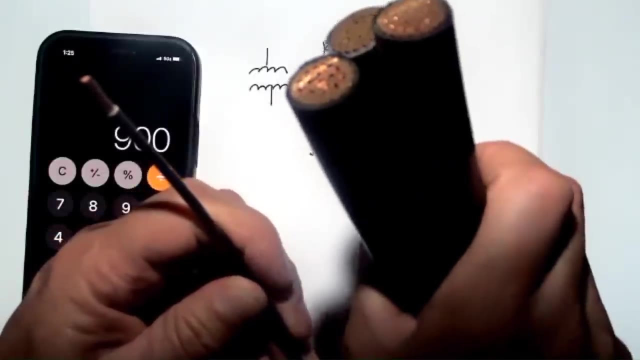 So now that you came up with 900 amps and we did the calculation to calculate the primary amps, it's kind of interesting If you take the wire that would be used for the primary and secondary and look at it. I'm going to try to hold this at the right angle here, but you can see that you'd need three of these conductors on my 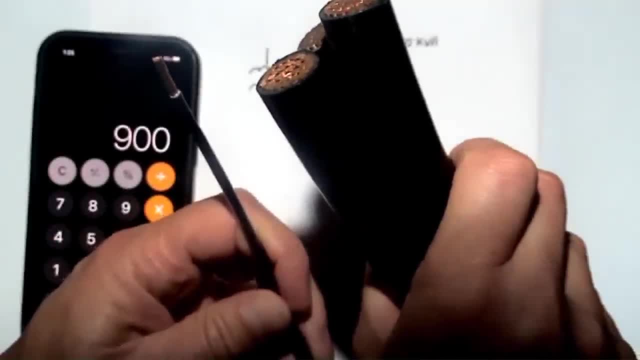 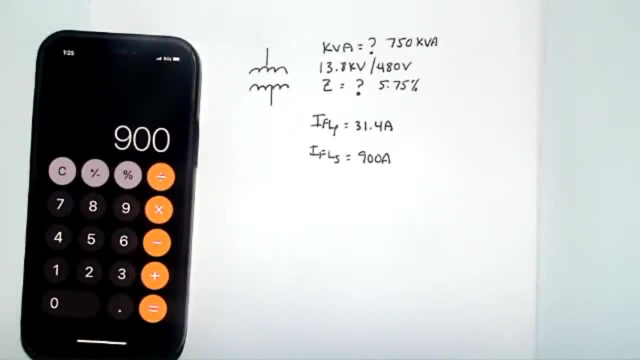 right hand And compared to the one conductor on my left hand, this would be your primary voltage wire and your secondary voltage wire. And so, as you can imagine, why do we use transformers? Because small currents, a little bit of copper. 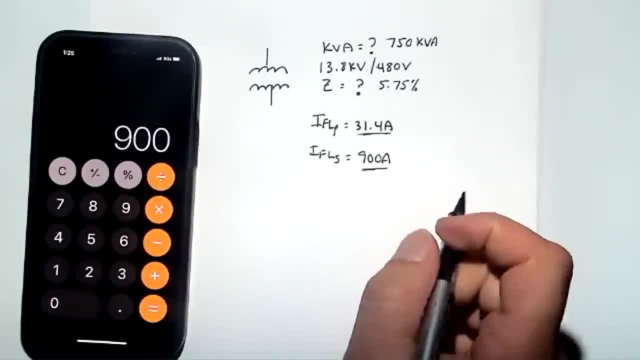 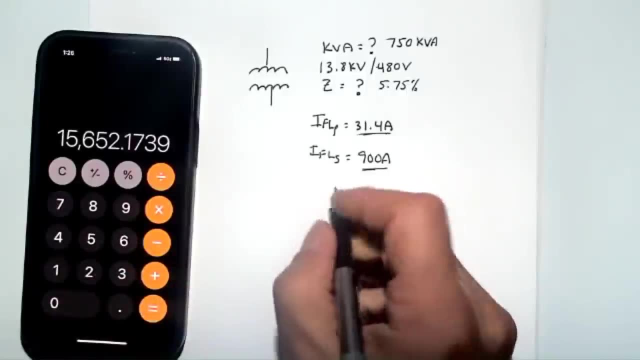 Large currents, much copper and any more. It's super expensive to do that. So let's calculate our fault current. Divide that number by 0.0575.. And we're at about 15,650.. 152 amps of fault current. 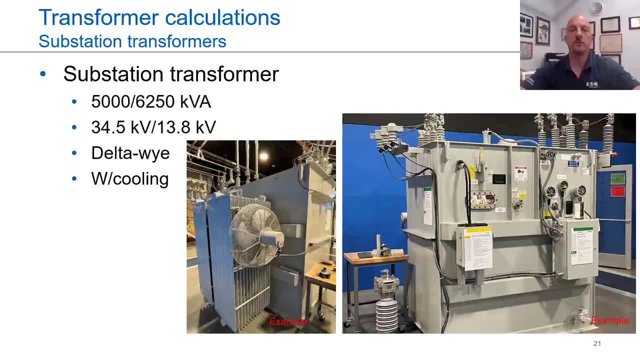 Finally, we'll talk about this transformer. This is a substation transformer, And what you see on this one is a couple of interesting things. One is, if you look on the back side of it, it has those radiators and fans. 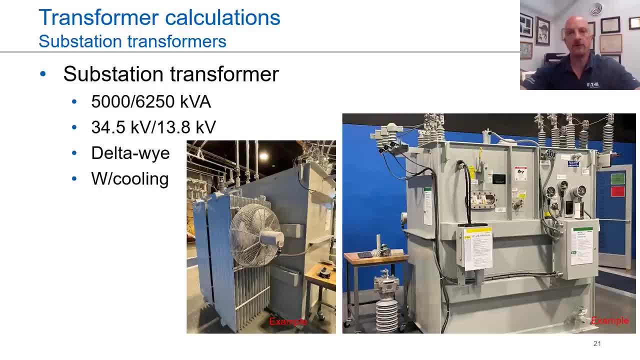 What that allows you to do is get multiple ratings, In this case, two ratings. It's 5,000 kVA base rating And then it has a 60 to 50 rating with the fans and the coolant going through the system. 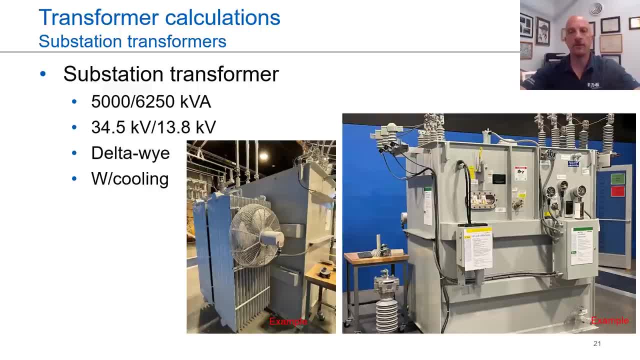 So what that allows you to do is run more power through it. in terms of kVA, That also is going to come into play when we talk about our calculations for this transformer. This one in particular is 34.5 kVA input and 13.8 kVA output. 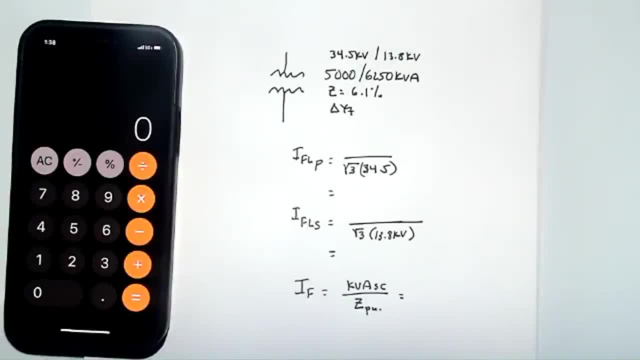 Okay, now so for this last transformer. this one adds a little bit more complication in a different regard, And that is that it has a slash rating. It has two ratings: It's 5 mVA, but it's also 60 to 50 kVA. 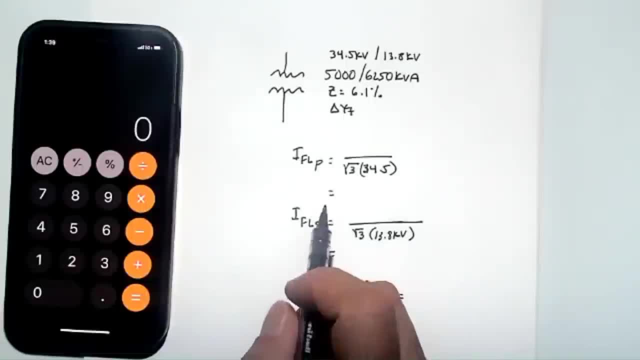 How do we determine what the full load amps are on the primary and secondary of the fault current? How do we determine that If we have two different ratings for that, We have two different ratings for kVA. Which kVA do we use for which? 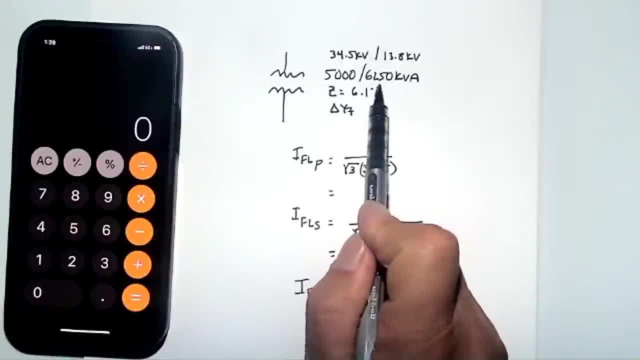 If you think about it, the kVA rating, the slash rating, really indicates that if we have cooling we can run up to that level, the 60 to 50. So when we calculate our primary and secondary full load amps, we want to use 60 to 50 kVA. 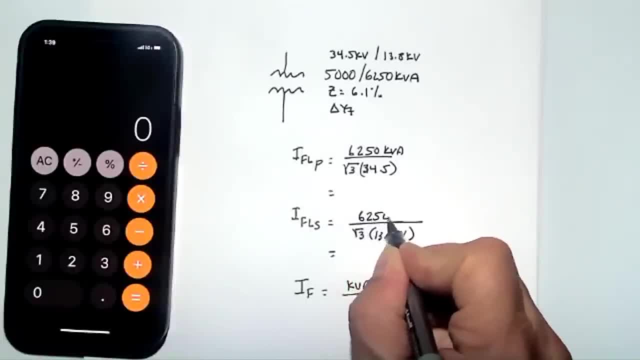 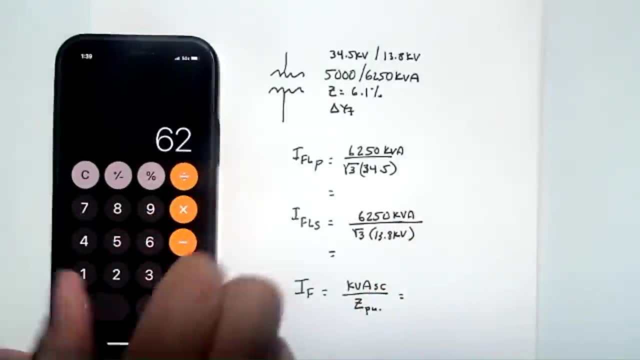 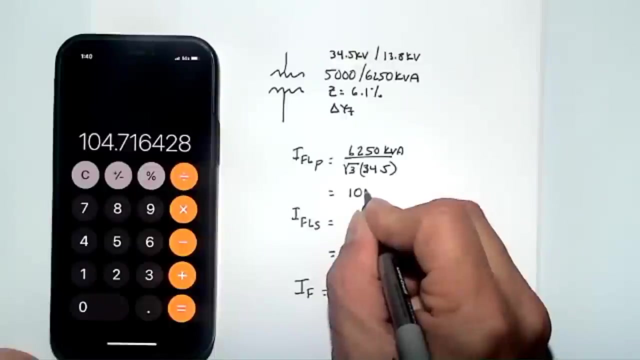 That means that's the most we can get out of that transformer. So our current has to be rated based on that. If we take 60 to 50, divided by 34.5, divided by the square root of 3, we end up with 104 amps- about 105 amps, 104.7 amps. 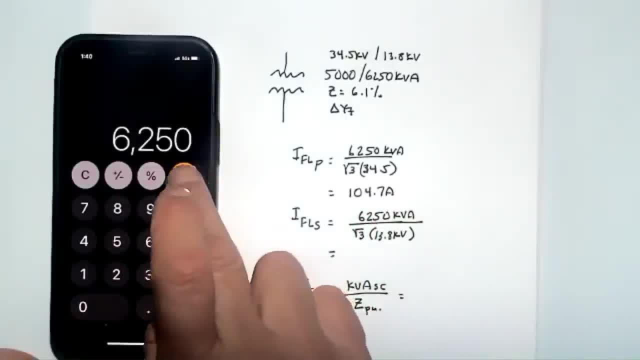 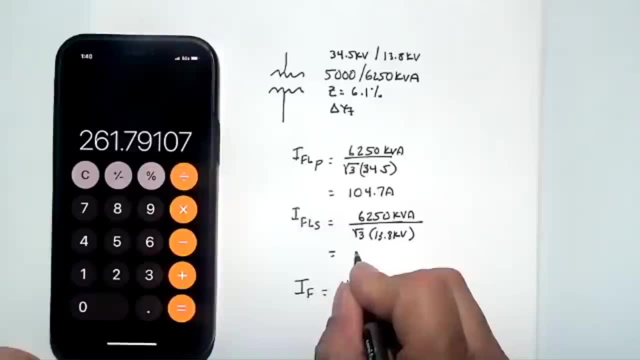 If we look at our secondary, we take 60 to 50 divided by the square root of 3, divided by 13.8 kVA, We end up with 260 kVA. We end up with 261.8 amps. So that's our secondary current and our primary current. 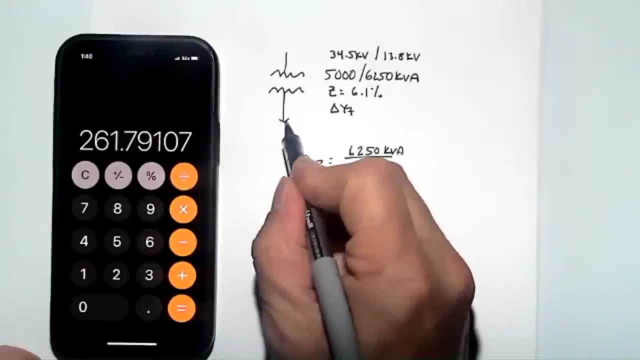 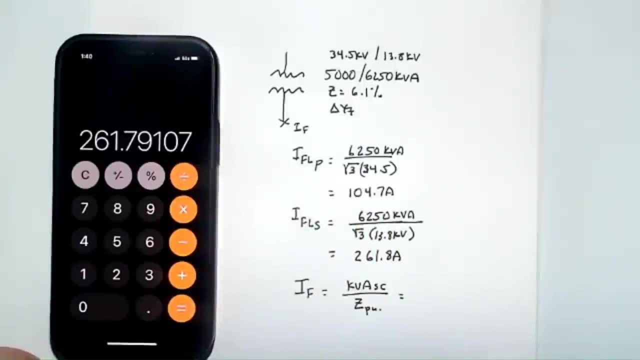 Now, in a normal situation, if we were just calculating the fault current, here I fault. we would just say: you know, take this number divided by the impedance, which we know is 6.1%. However, this 6.1% is not based on this 60 to 50.. 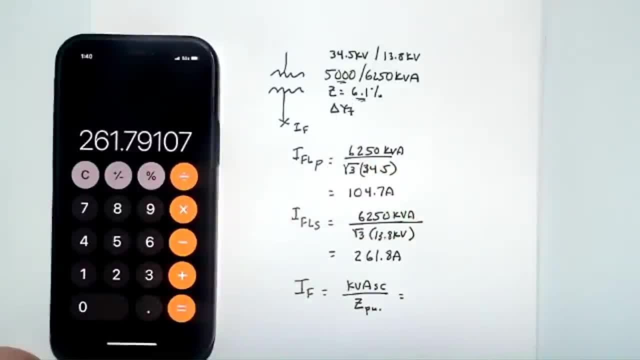 This 6.1% is based on the base rating. There may be two or three ratings for kVA. This 6.1% is only based on this value, So we need to go back to our short-circuit kVA rating, which is going to be 5,000 divided by the square root of 3, divided by 13.8 kVA. 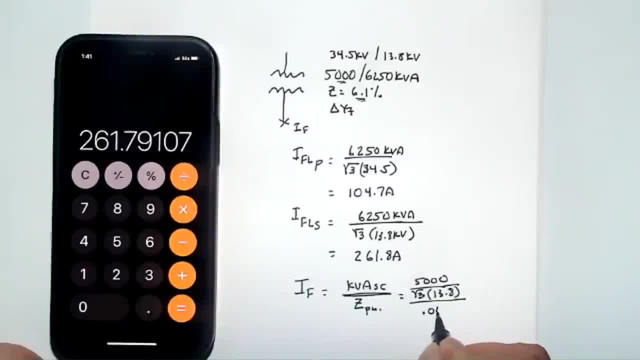 And then divide that by the impedance, which is 0.61.. And that number would be 5,000.. 5,000 divided by 1.73, divided by 13.8.. So that number is 209 instead of 261.. 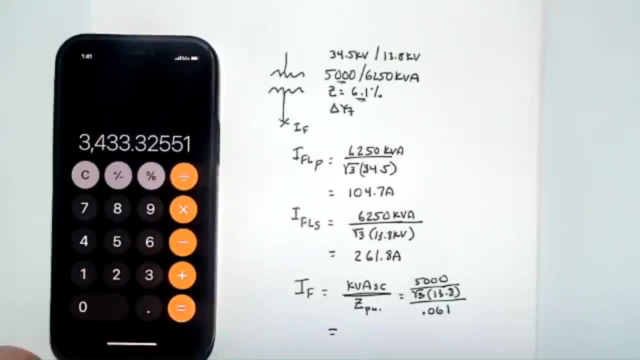 Then we divide that by 0.61.. Otherwise, our fault current would be higher: 34, 33.. Otherwise, our fault current would be higher than it would be if we used the other number. It would be higher than it would be in reality based on the impedance of that transfer. 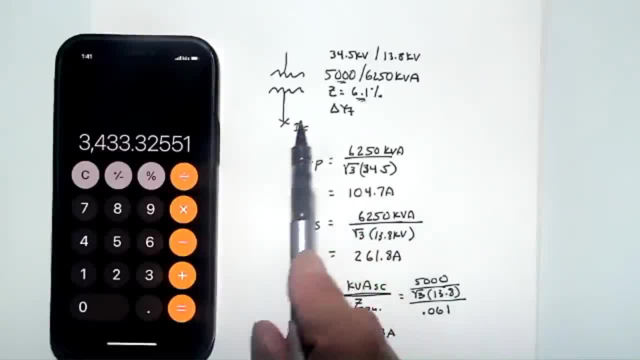 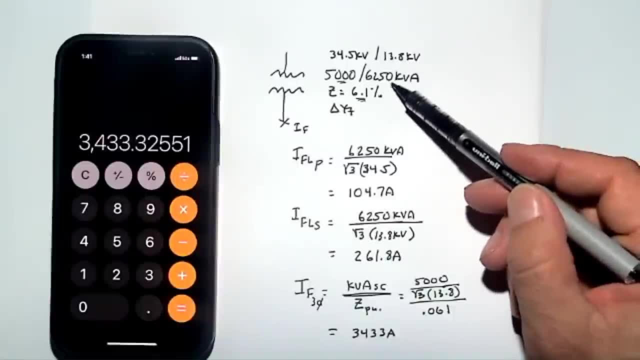 And again we're starting to get into that situation where we may want to look at what the actual source impedance above there is. So those are the key things here. 60 to 50 is the most kVA we can get through it. 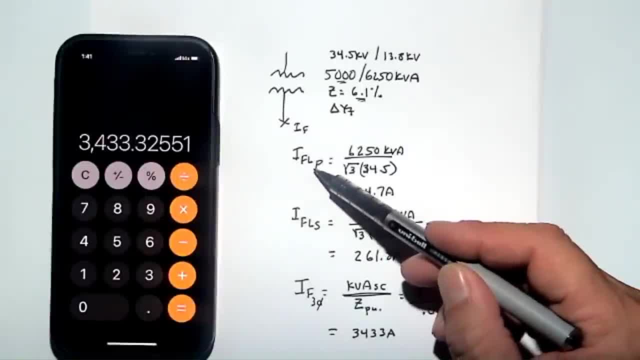 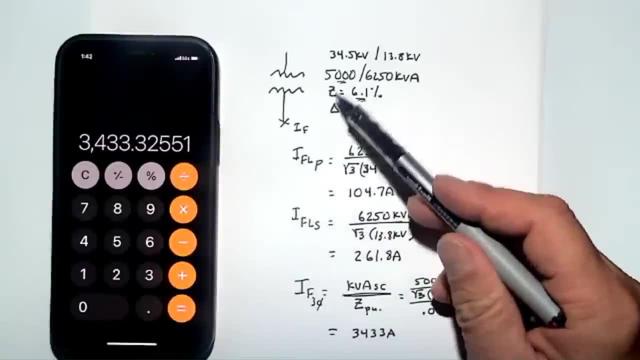 So the most kVA means the most. In other words, in order to use the full capacity, we want to base our primary current based on that- 60 to 50. If you base it on this one, you're just limiting the capacity of the transformer artificially by putting a breaker or something ahead of it and limiting the capacity of the load. 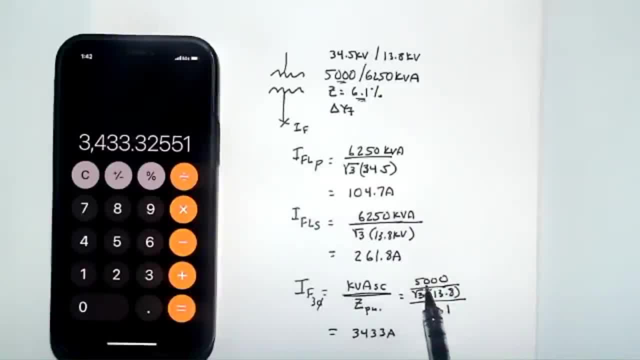 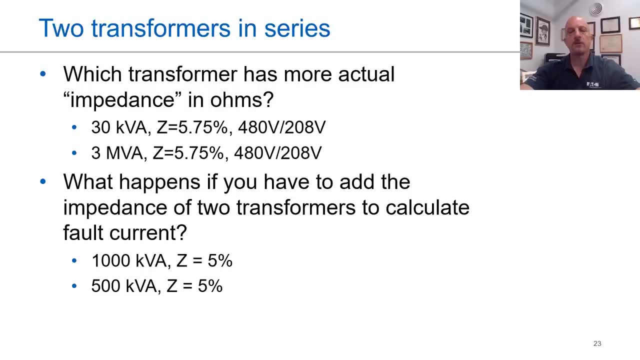 And then for the fault current we use the 5000 or we use the base rating in the base impedance. So a lot of questions come in when we're doing this class in person about the impedance of the transformers being the same and the kVA being different and how that affects your system and really what that means. 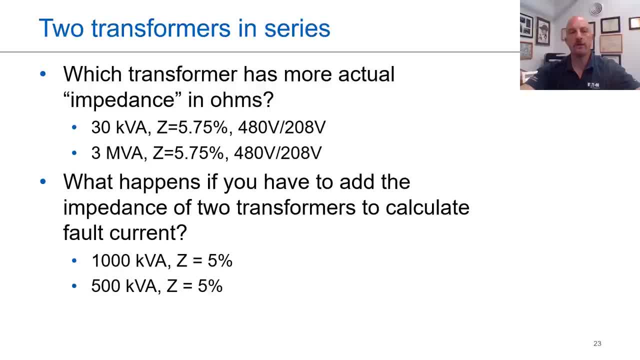 So, if you think about it from a very simple example, a 30 kVA transformer versus a 3 MVA transformer, which one of them is going to provide more fault current, And I think we would all kind of agree with that. 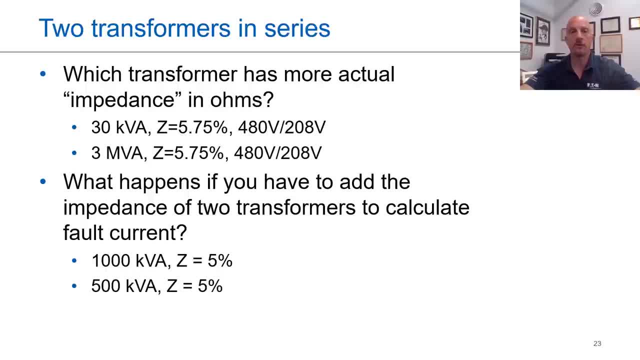 We would all come to the conclusion that the 3 MVA transformer would provide more fault current at the same voltage level. What happens if you have two transformers in series? How do you add them together? And so let me show you that as a quick calculation. 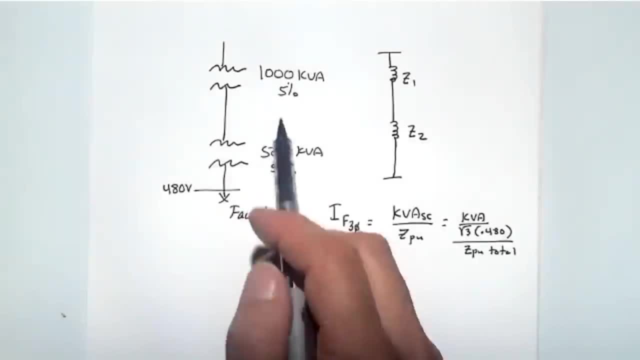 Okay, Now here's a situation that you also have to understand. What if I have two transformers in series and the ratio of those transformer kVAs is not 10 to 1, as we've been assuming? So we can just say it's an infinite bus above the downstream transformer. 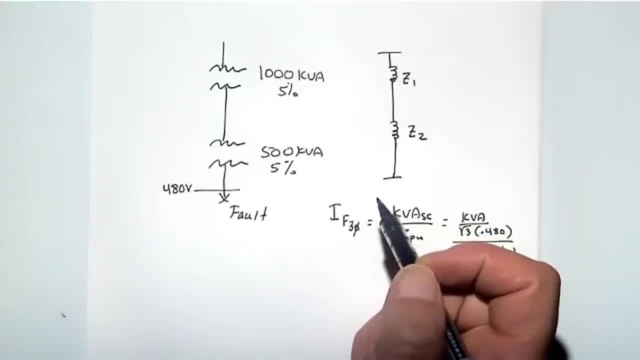 In this case, these two transformers are the same. These two transformers are actually relatively similar in size. We want to add them in series to create that series impedance so that we can figure out our total fault current at this point on the system. Now the nice thing of it is, if we calculate the fault current here, the only thing we need to know is which kVA to use. 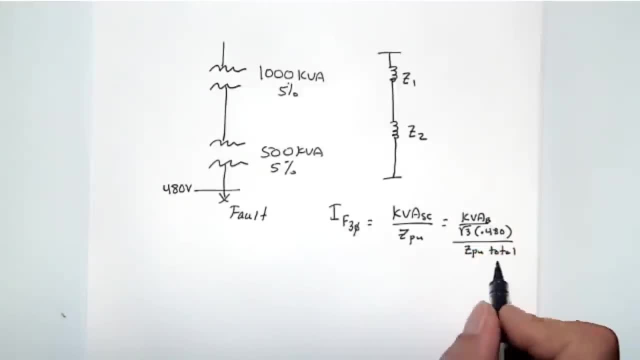 And we're going to use kVA base, one or the other of those kVAs, And then we're going to use a Z per unit total, which is the series sum of those impedances. But we can't just take 5%, 5% and call it 10%. 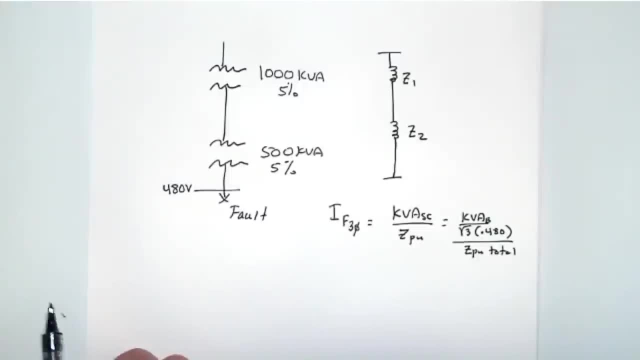 We have to combine those on a common base. So what I like to think of is if you take this transformer and this transformer and you say which one delivers more fault current, And I would say the 1,000 kVA delivers more fault current. 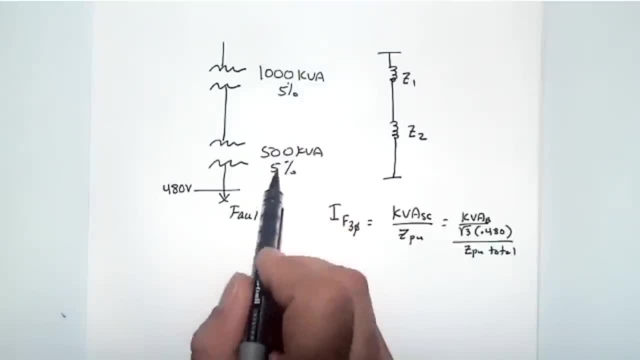 So if I put those side by side, this one has a higher impedance. The 500 kVA has a higher actual impedance in ohms compared to this one. So if I want to take my KVA base, KVA base. 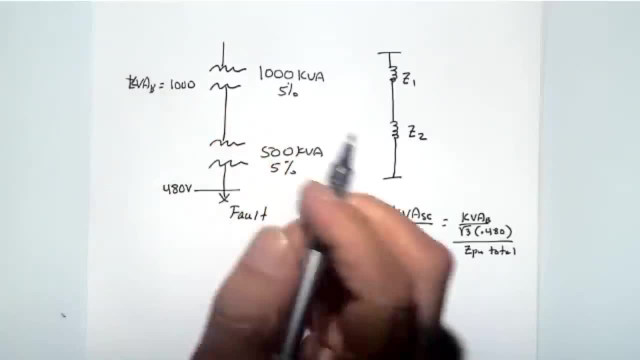 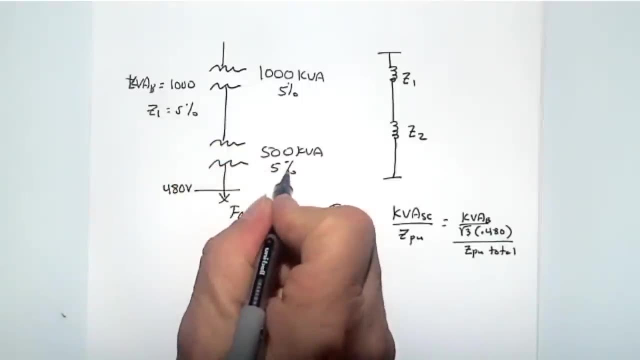 And make it 1,000. Then my Z for this one: Z1 is 5%. And then my Z for this one: is it going to be bigger or smaller? And, as we said, it's more impedance at that base. 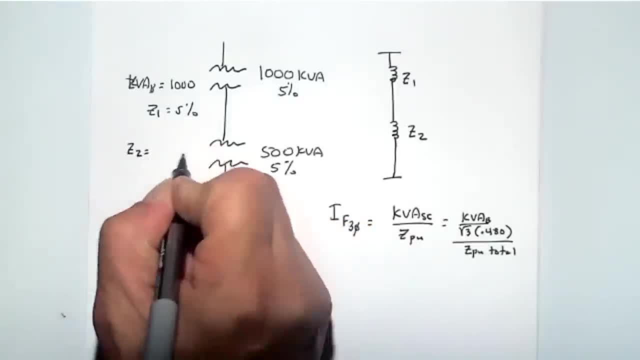 So we're actually going to say: Z2 is the new base, which is 1,000.. Divided by the rated, which is 500. Times Z here, so 5%, That gives us the total impedance of 10% for that one. 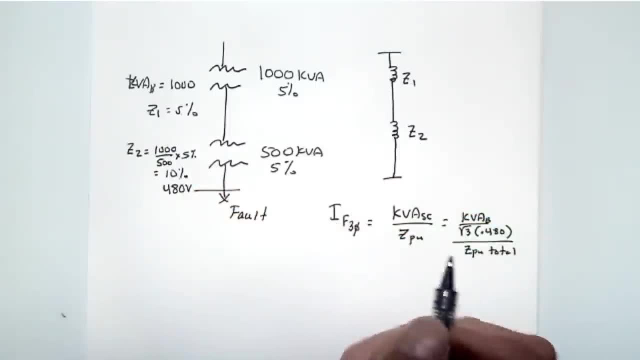 So Z1 plus Z2 in that case is 5 plus 10. And I would end up with: I would end up with KVA base 1,000.. Divided by the square root of 3.. Divided by 480.. 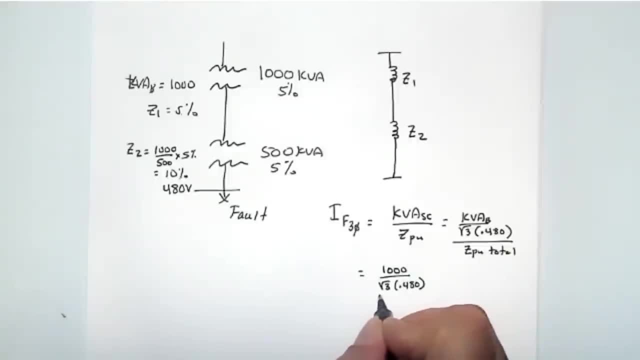 And I think we know what that number is by now, which is 1,200.. And then we divide it by our total impedance, which is 0.15.. Or 5% plus 10%, So we take 1,200.. 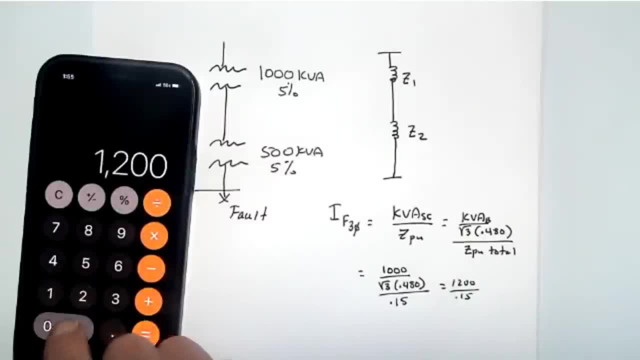 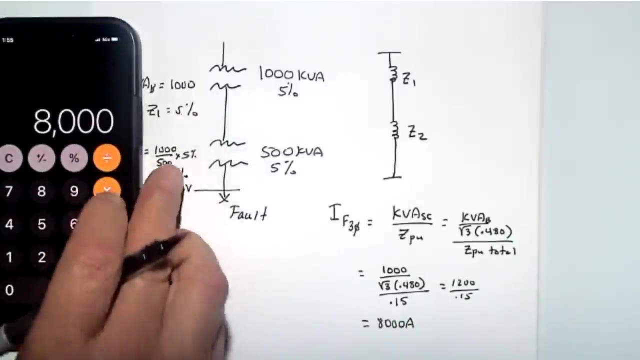 Divided by 0.15.. 1,200.. Divided by Divided by 0.15. And we end up with about 8,000 amps of full current. Now, what I'm going to do is I'm going to show you that it would be the same if we went the other way. 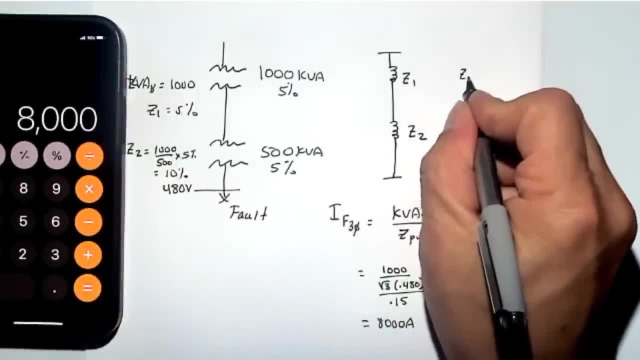 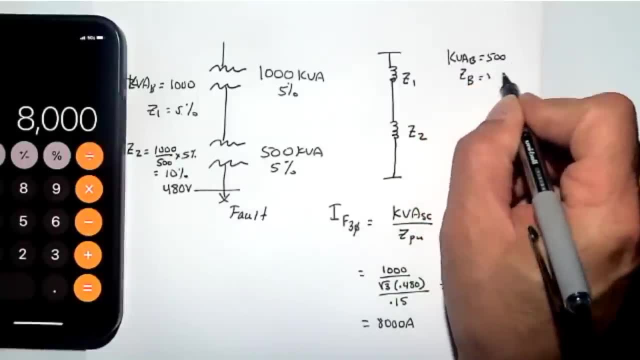 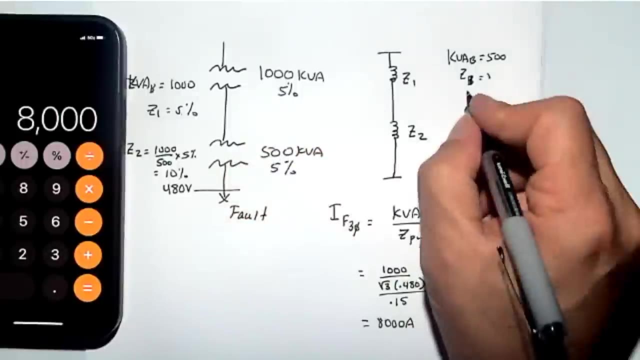 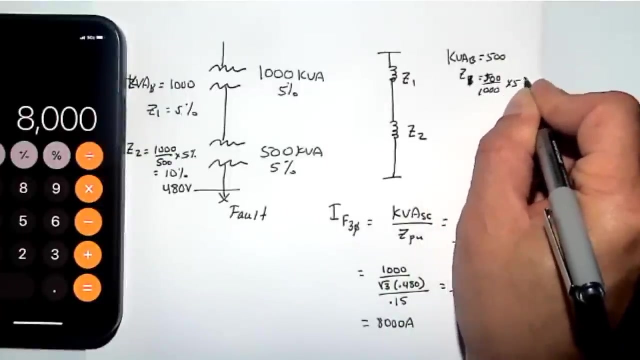 Let's say we take our Z base. Z base is 5, or sorry, KVA base is 500 KVA. So Z1, again delivers less impedance at that 500 KVA base. So it would be: Z1 would be 500 divided by 1,000 times 5%. 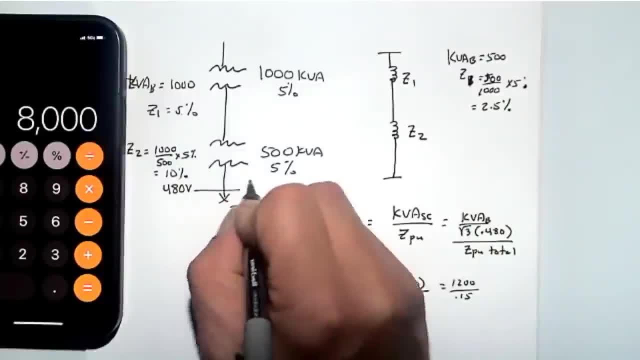 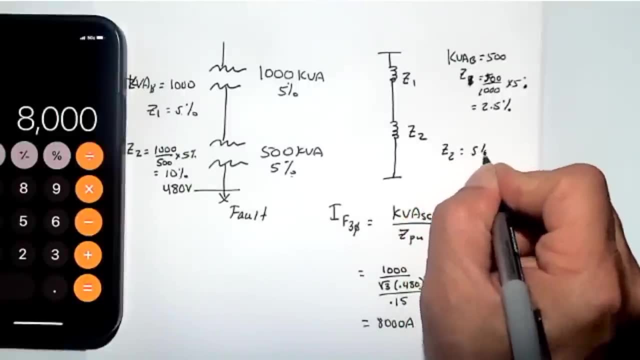 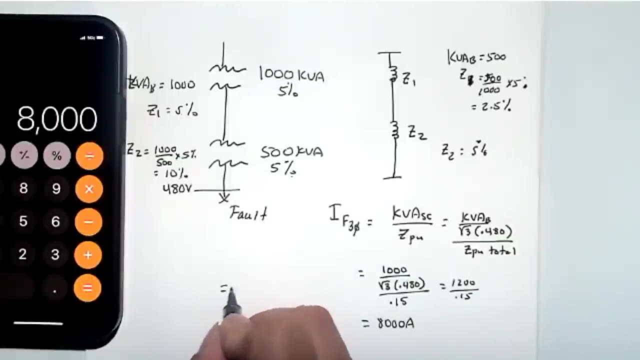 We end up with 2.5%. Z2 at 500 is going to be still 5%, So Z2 is 5%, And then we add those two together And we end up with basically: let's do it here. 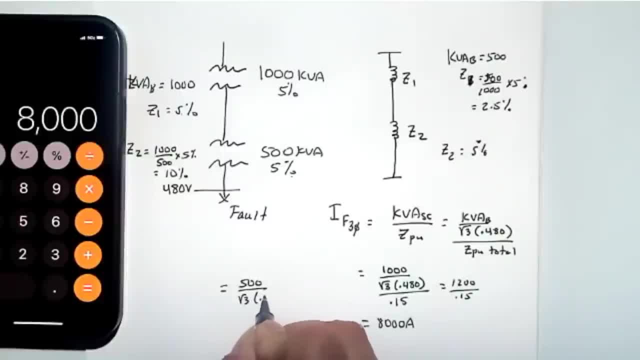 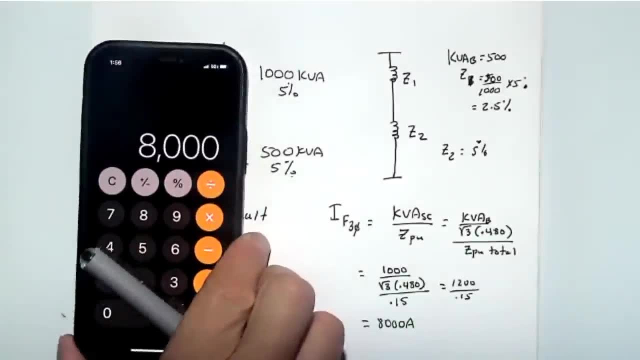 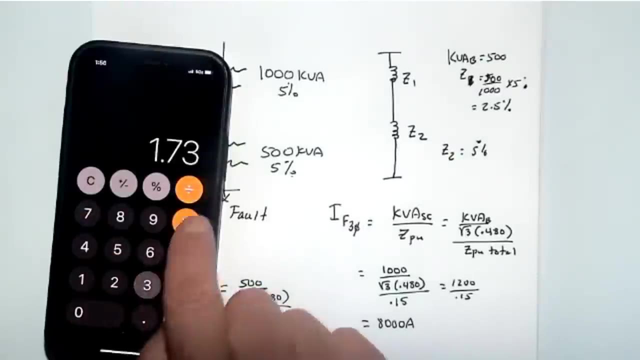 500 divided by square root of 3, or 80.. Divided by 0.075, which is 0.02, or 0.025 plus 0.05.. And we'll get 500 divided by 1.73.. 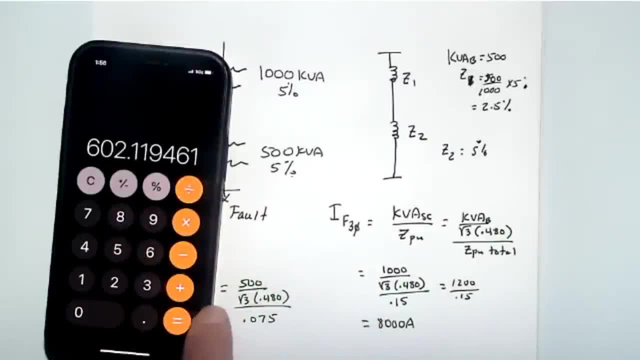 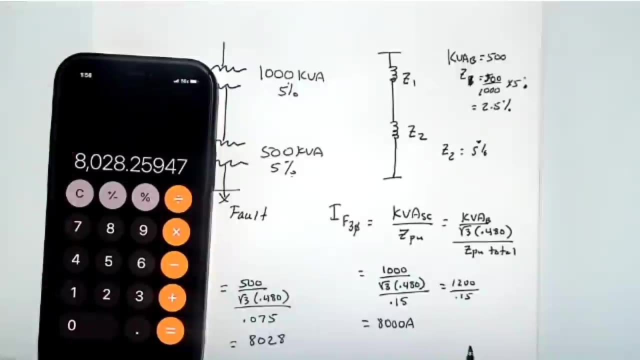 Divided by 0.48, which is half of that 1,200 that we should get right, And then divide that by 0.075.. And we get 8,000.. And again I'm still a little bit of rounding error for my square root of 3.. 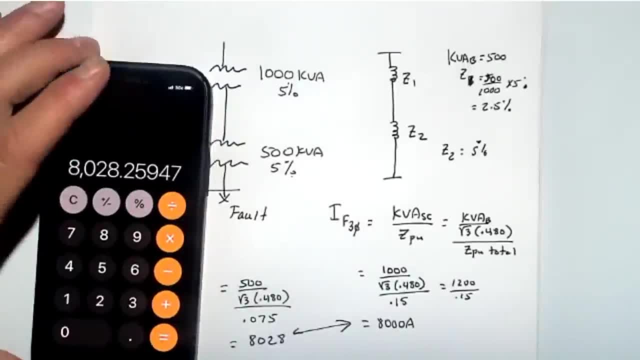 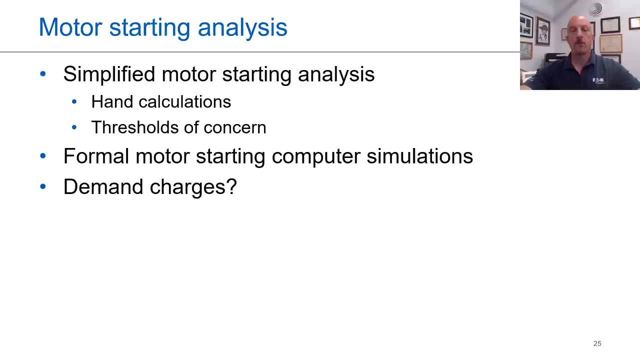 But these two numbers are the same. So again, we can calculate that full current either way, But we do need to combine those bases to make sure that the transformer impedances are based on the same thing. And now that you're all formal experts on calculations for anything transformer related, right. 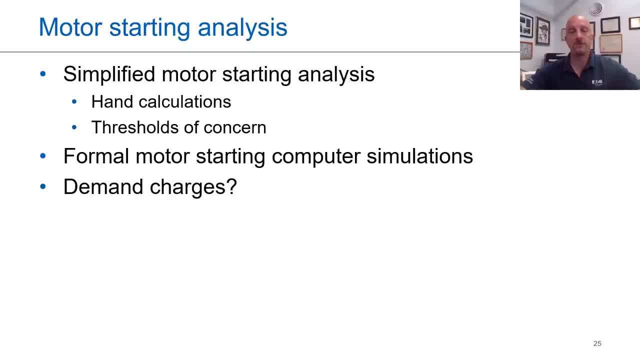 You can do the full load amps and the full current calculations. Let's talk a little bit about motor starting and what's important for that. We're going to do a couple of quick hand calculations And then we'll kind of figure out where those thresholds of concern are, wherever we're going to have voltage drop, according to motor inrush. 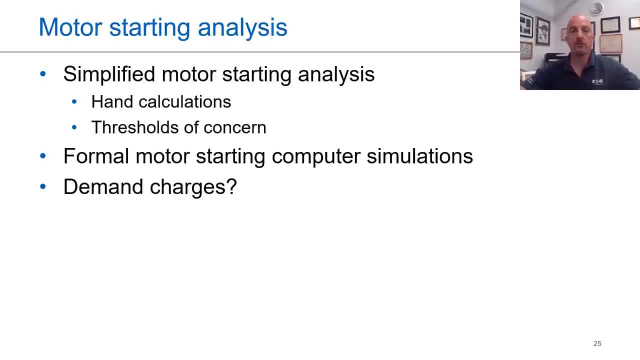 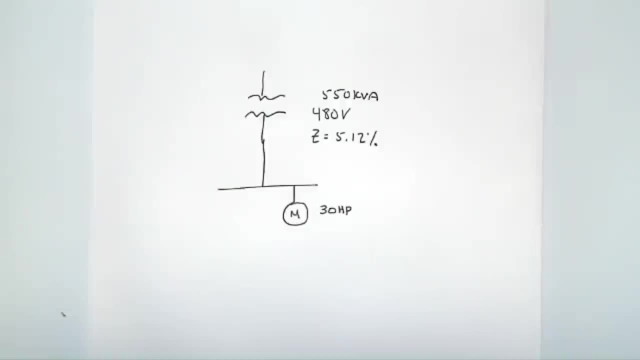 And then we'll talk a little bit about motor starting and basically using computer simulations for that analysis, And then finally, really, we're going to talk about how that might or might not work, That might or might not affect demand charges. So now we're going to do a simple hand calculation, based on motor starting, to calculate the voltage drop associated with the inrush current of a motor. 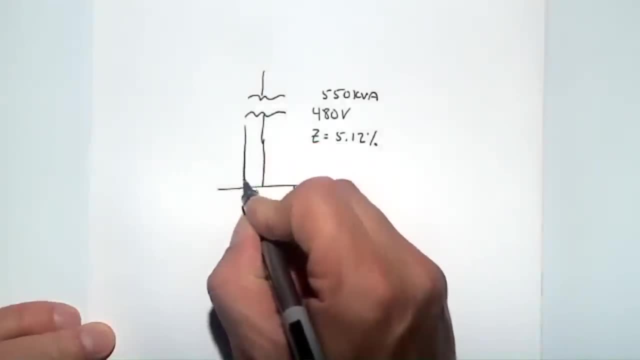 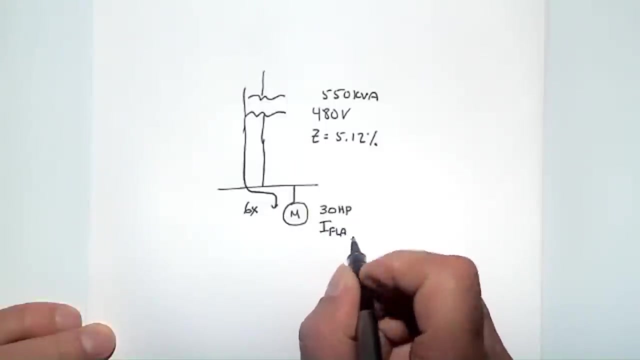 And, as we know, the motor inrush current is typically considered six times the load amps, So that current has flowed down through the transformer into the motor. And so when we talk about a motor, we have I full load amps. We calculate that. 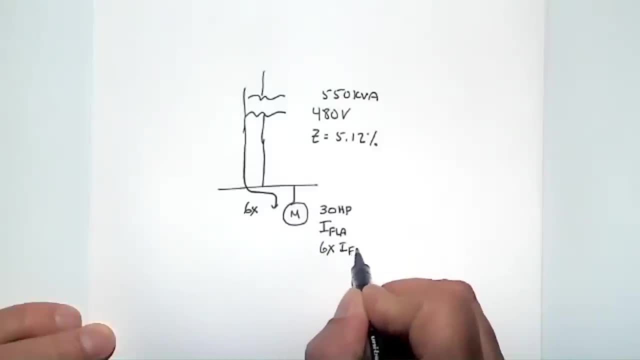 But the inrush current is six times I. full load amps equals inrush. Now what's interesting about that is horsepower is just about equal to KVA, And if you do the calculation and take out the efficiency and the power factor and everything, you end up finding out that horsepower is about equal to KVA. 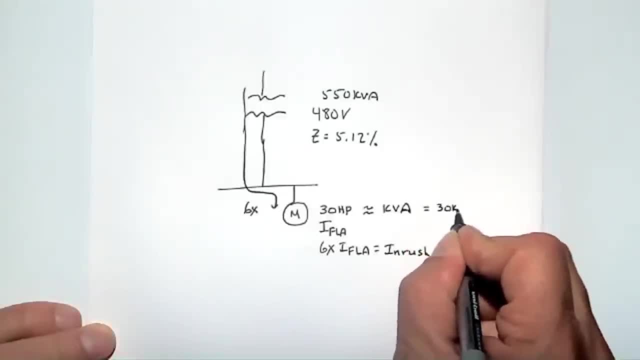 So we have about 30 KVA of normal load. you know KVA. As we look at inrush, then our inrush is six times, Then our inrush is six times our normal KVA, which is 30. So six times 30 was 180 KVA inrush. 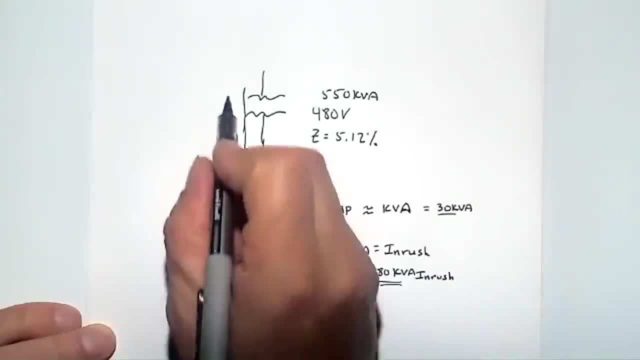 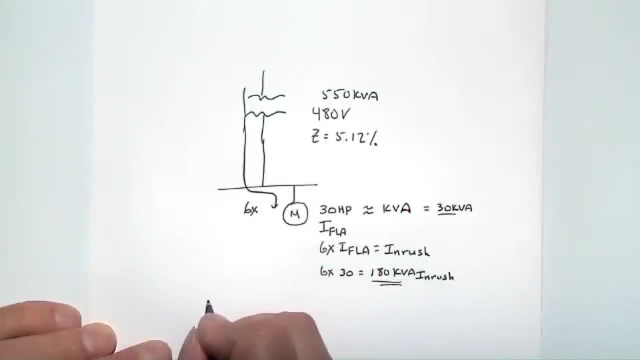 So if we just take that number, that inrush KVA, and look at the ratio of that inrush KVA versus this transformer size, So basically we take KVA Inrush Divided by KVA transformer And multiply it by percent Z. 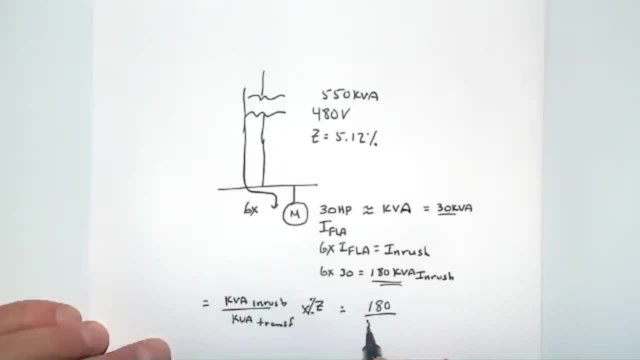 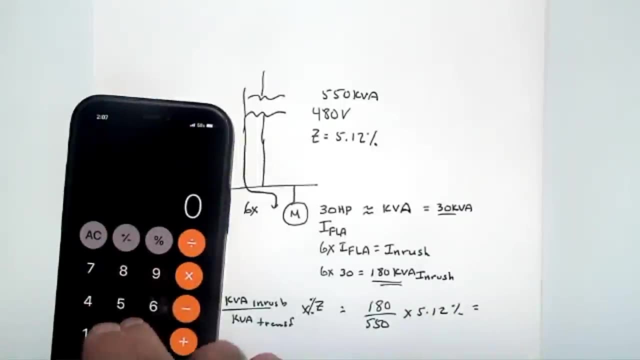 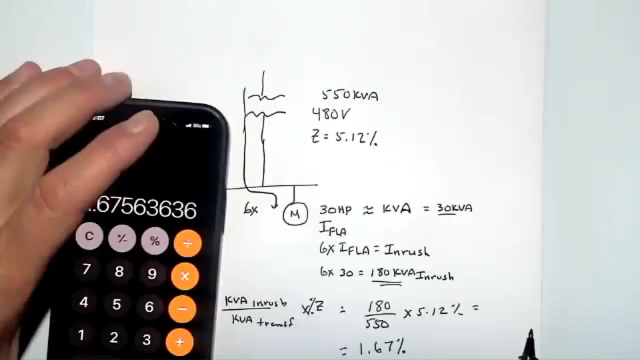 We get 180. Divided by 550. Times 5.12%. And Here's what we get: 180 divided by 550. Times one 5.12%, And that ends up being 1.67% voltage drop. 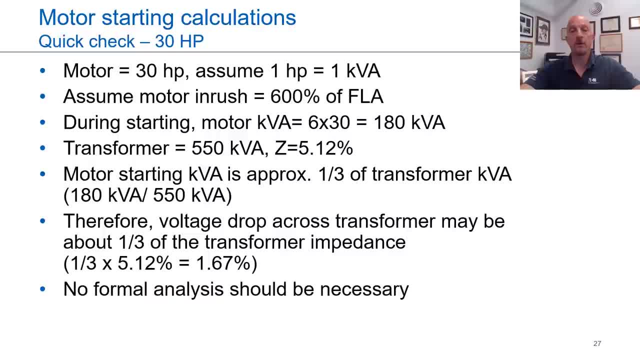 So again, in summary, what we saw there was that the motor is going to give us about six times inrush current, So once we create 600% full load amps, basically for that motor We had about 180 KVA of inrush KVA. 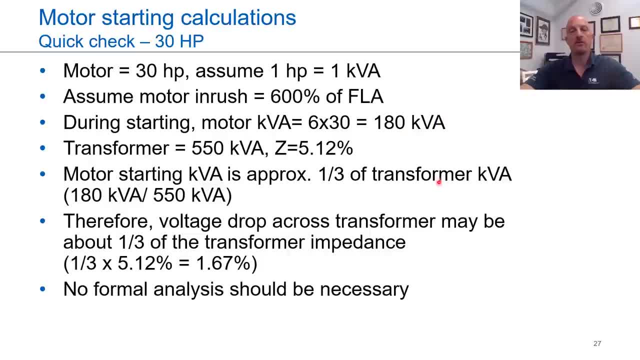 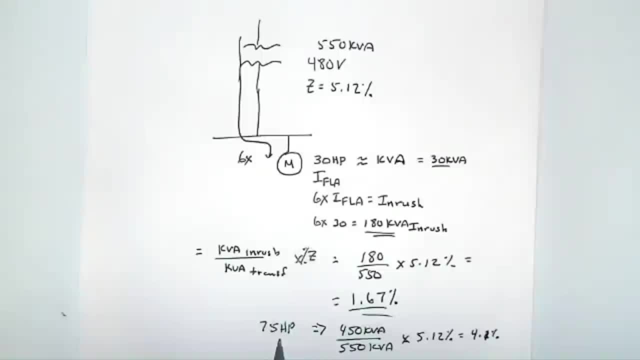 And then we basically ended up with About 1.67% drop. So really, for that percent drop we don't really need or require formal analysis And we should be good in this situation. So then, if we repeat that 75 horsepower, 75 KVA times six gives us about 450 KVA of inrush divided by the transformer. 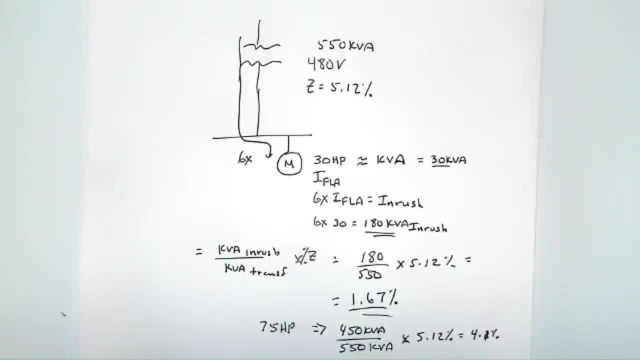 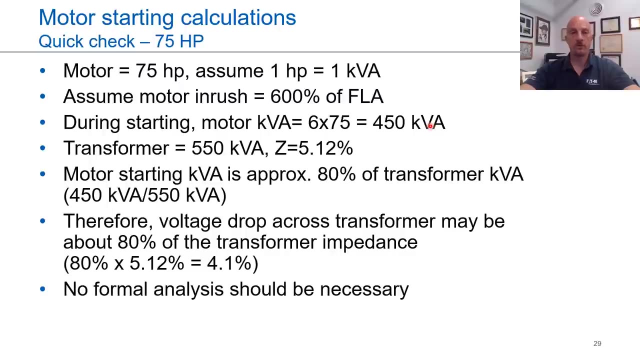 KVA times the impedance of the transformer, which gives us about 4.1% Voltage drop. So again in this case- you know, we have a little bit more inrush current because the motor is bigger- We have about 450 KVA worth of inrush KVA. 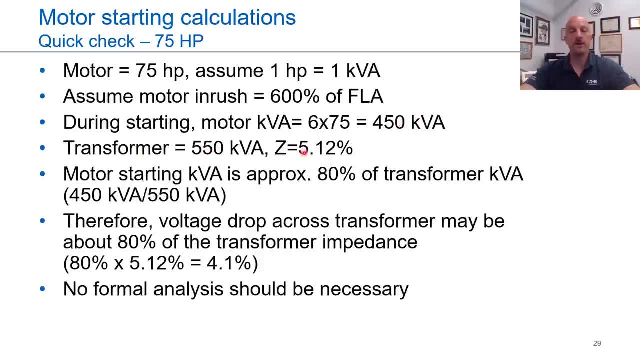 Compare that to our 550 KVA size of our transformer. You ratio that and look at the impedance and we get about 4.1% drop. Now, again, that doesn't really require formal analysis, but we will see that in terms of light flicker. 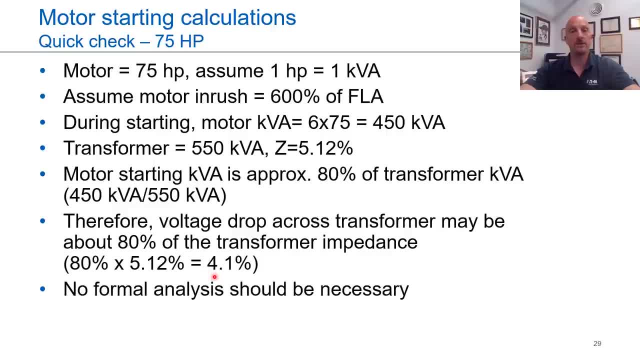 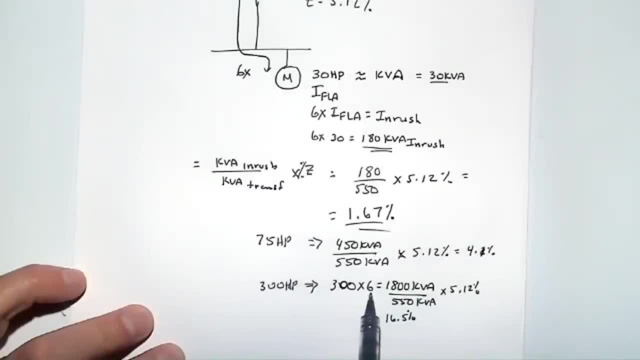 And so again, as you see, if it was, the motor was starting many times a day, you might get more of an inrush effect in terms of people noticing and maybe problems associated with that. And then, looking at it, for 300 horsepower motor, we have 300 times, six times inrush, to give us 1,800 KVA divided by 550. 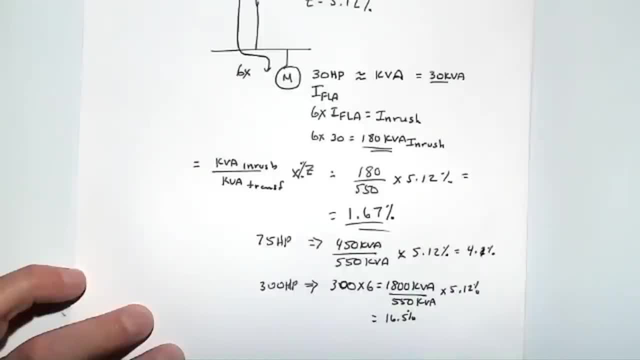 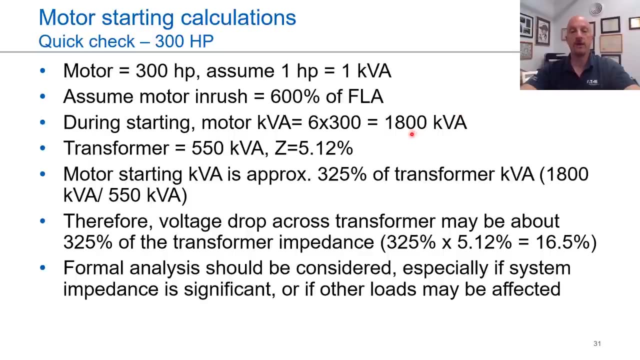 So again, that number is going to be bigger than the impedance. In fact it's 16 and a half percent Now, finally, for this one, What you notice, The interesting thing about this is our inrush KVA. our 1,800 KVA is actually bigger than the transformer by a good bit about three times, or more than three times. 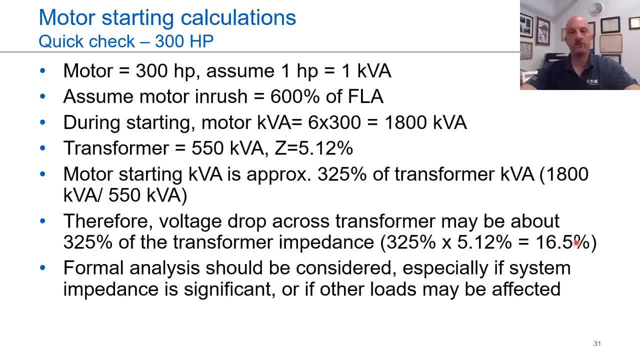 So we're seeing about 16 and a half percent voltage drop, as we mentioned. So if we do that, what's going to happen is we are going to see a significant notice on light flicker, but also we may actually have equipment dropout. 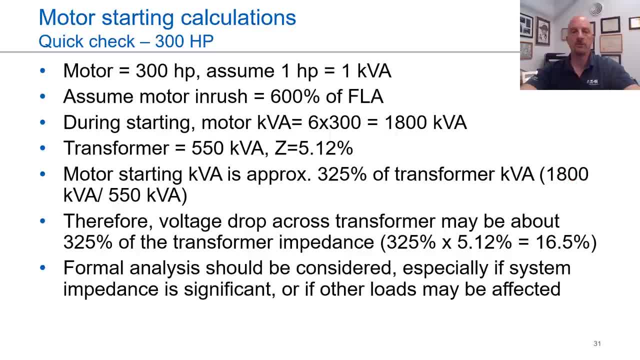 So this case we probably do want to do a formal calculation with some sort of a computer simulation to make sure that, again, these hand calculations are very rough, but to make some additional calculations to see what the actual drop is And really honestly how long it's going to last in terms of motor starting and so forth. 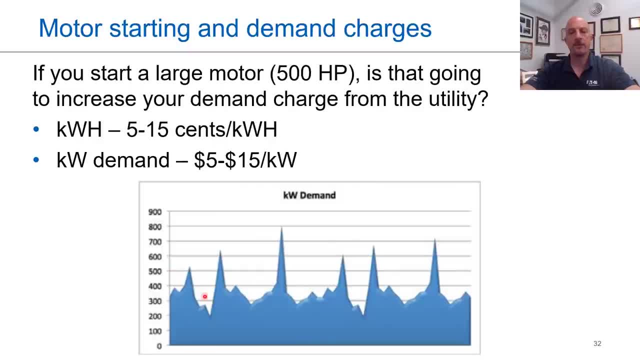 And one of the questions I get quite a bit of is: you know you have these peak inrushes of different things throughout the day. Is motor starting going to affect my demand charge? No, really, it's really more about understanding what demand charge is. 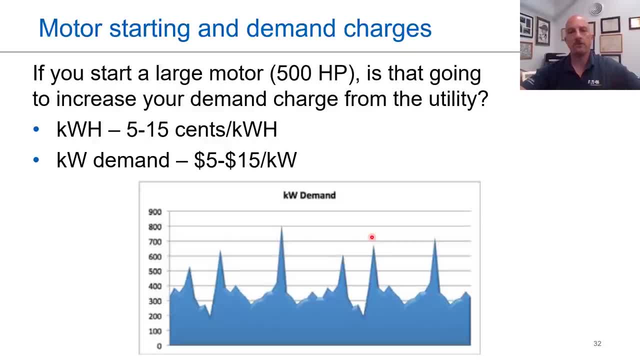 Demand charge is the 15 minute window That utilities look at and see what your maximum demand is for the month in terms of kilowatts or megawatts, And the reason that they need to have that number is so that they can supply a customer in the worst case scenario with the capacity of their system. 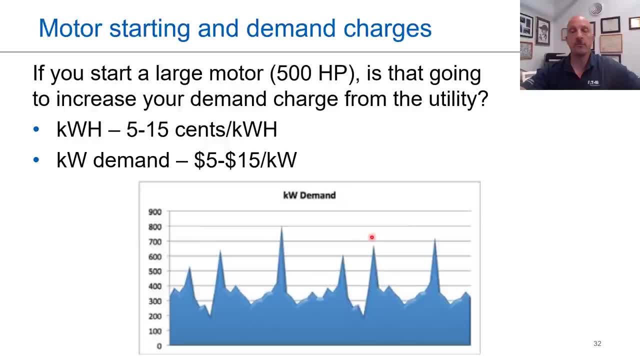 And especially if all the other customers have, you know, a maximum capacity at a certain time. The pipe, the actual wires, transformers and everything behind it. the system has to be able to withstand that. What's interesting about that is a lot of people assume that when you start a motor, 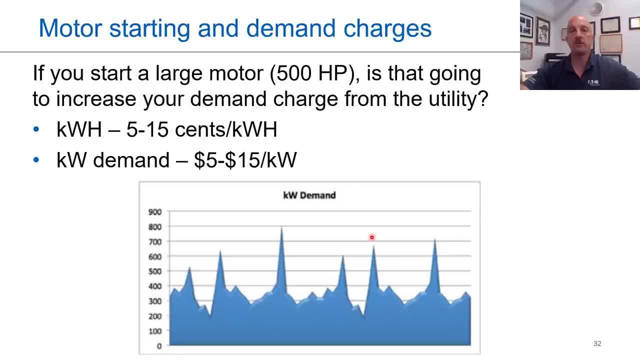 you get this big inrush current, you're going to affect that demand, And that's not really true. The fact of the matter is that the inrush for a motor is very short in terms of seconds. Even for big motors it's, you know, five to 10 seconds. 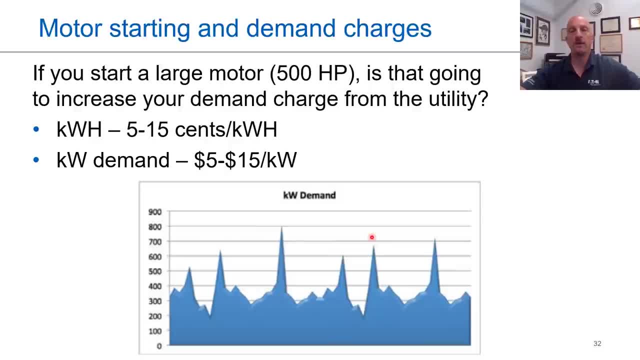 And so over that 15 minute window it's very minimal, And the other part of it is that that inrush current is actually reactive current for the most part. So even though it seems like it would be a big deal, it really doesn't affect the demand. 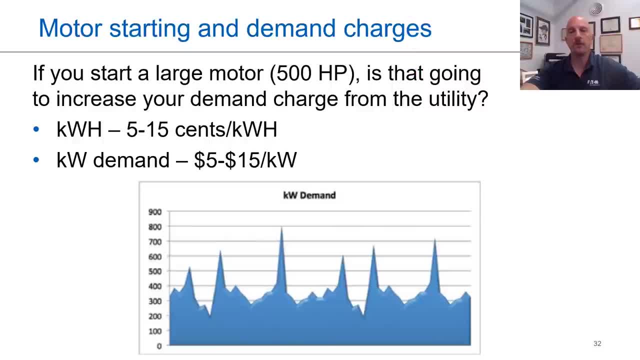 And that's very important to know as you think about. you know promising a customer, you know whether or not they're going to save money by putting in a soft start, for example, because it's not going to change your demand. 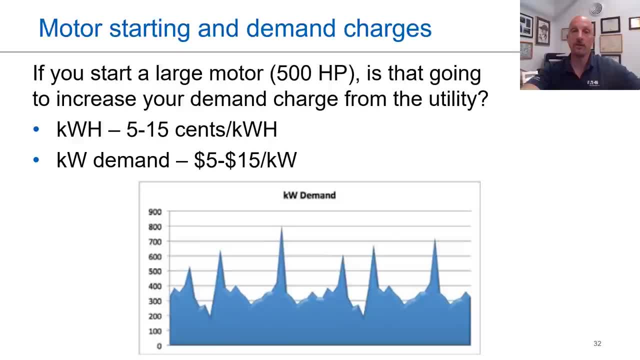 It will affect the motor inrush. It'll save the motor from being potentially damaged for doing that over and over again And it'll also save the voltage drop that's very important from these calculations. But it's not going to affect the demand. 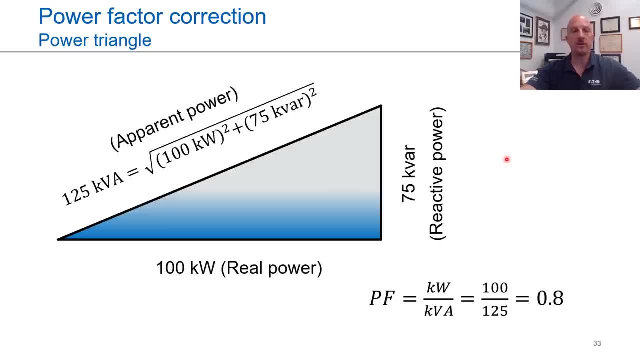 Okay, now let's switch gears again. So here's the power triangle. We're going to talk about power factor correction for a minute And we'll do a couple quick calculations here around that. But for example, when we look at the power triangle, 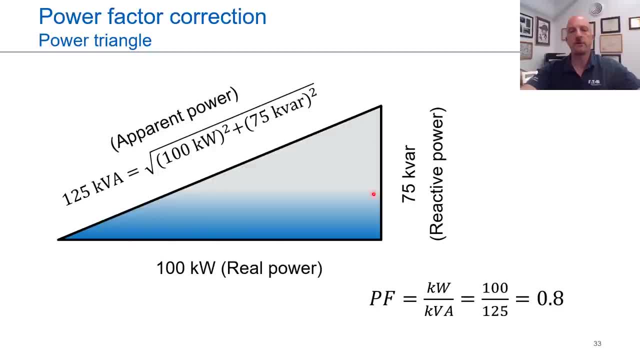 we look at the real power on the x-axis, reactive power on the y-axis And on this hypotenuse here, this is the apparent power of kVA. So how do we calculate that? We take the power factor, which is the difference between kilowatts divided by kVA. 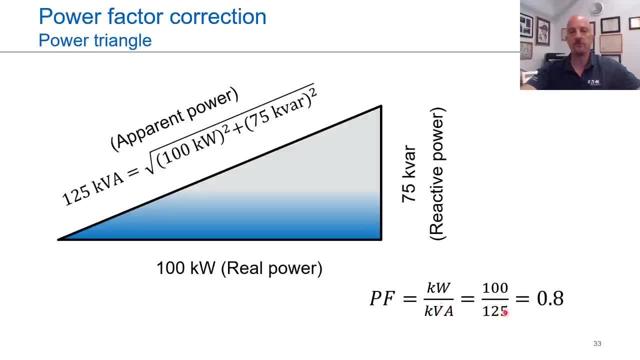 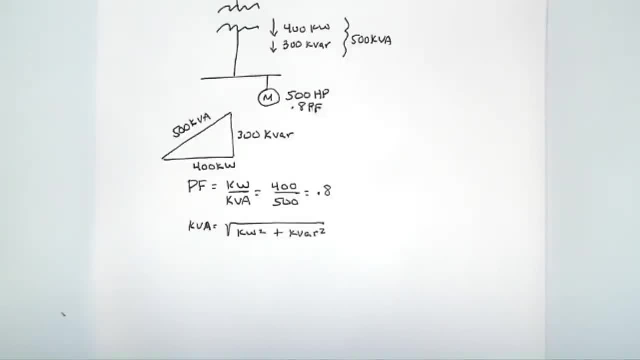 The ratio of kilowatts divided by kVA in this case is 0.8.. Okay, for the last example. then we're going to give you an example of power factor correction and how we apply capacitors to correct for a power factor. 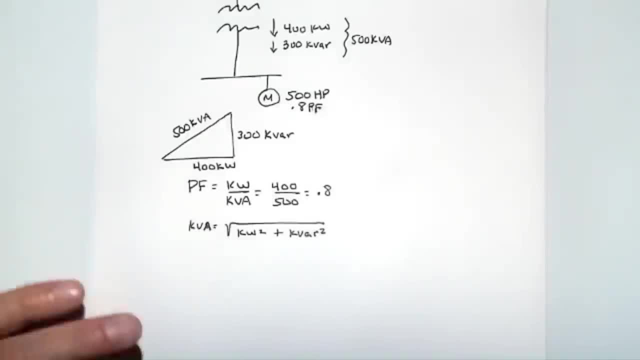 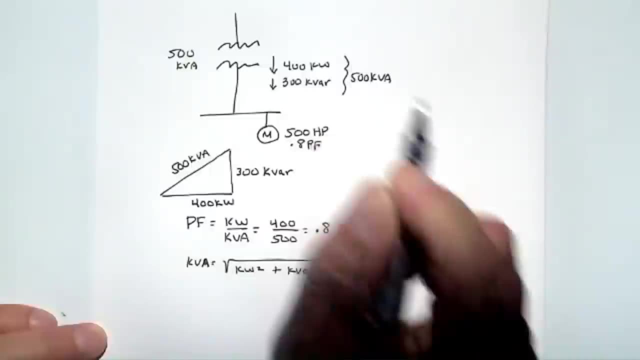 So that you could add more load. In this case, we have a transformer that's 500 kVA rated, 500 kVA rated, And it has a 500 kVA load flowing through it to this motor: 500 horsepower, 0.8 power factor. 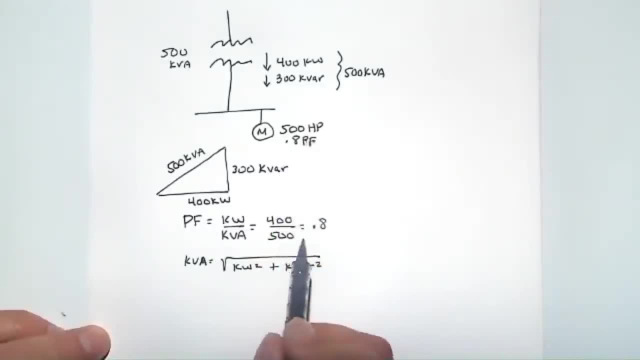 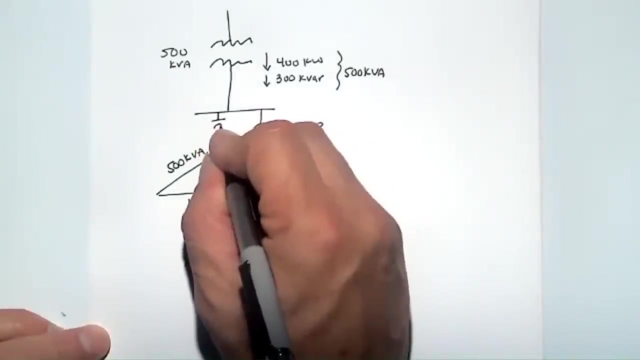 So at 0.8 power factor our kilowatts are 400, our k bar are 300, and our kVA again is 500.. So that's what's flowing through the transformer right now. We want to apply a capacitor to relieve some of the capacity of that transformer so that I can add another load over here. 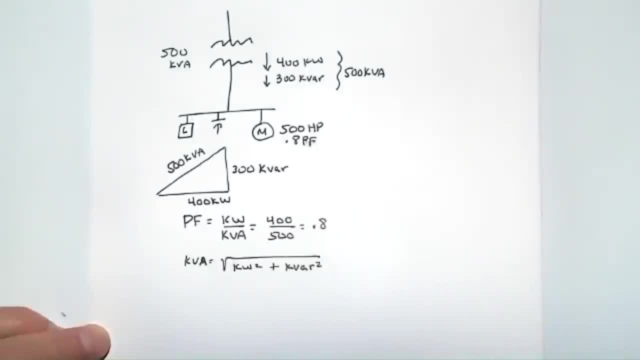 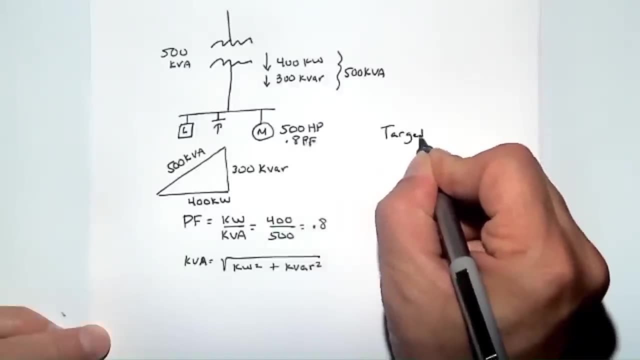 And I can put some other load, whether it's resistive or reactive or a combination of loads. So let's say the target power factor. target power factor is 0.95.. How do I get there? So my target power factor is 0.95.. 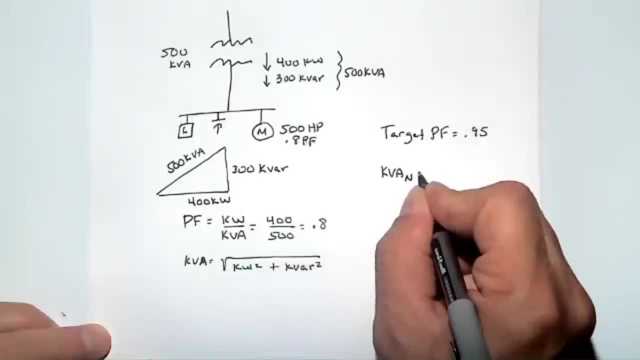 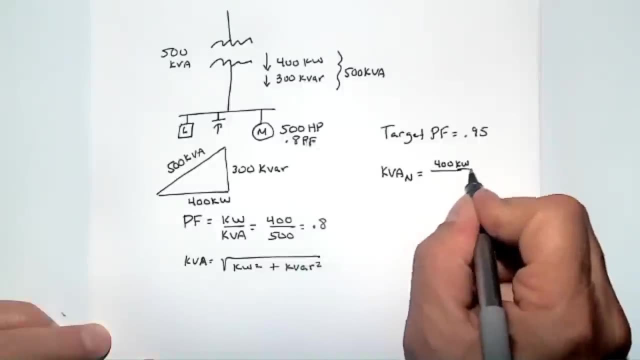 My actual new kVA. then kVA new Would be my existing kilowatts, which is 400.. My kilowatts aren't going to change. Those have to still come from the utility divided by my target power factor, which is 0.95.. 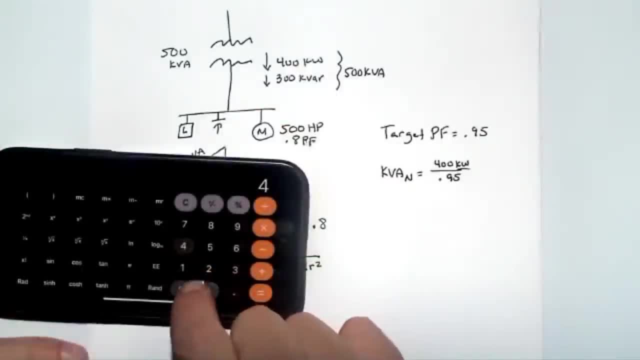 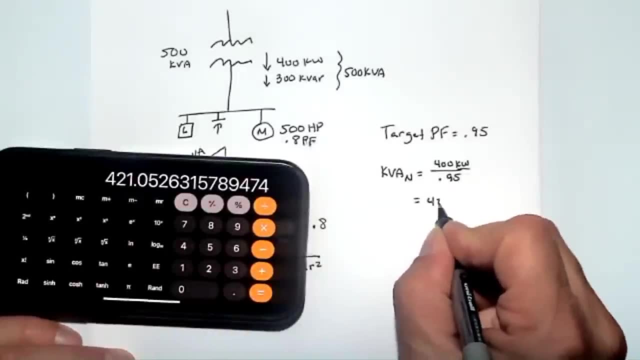 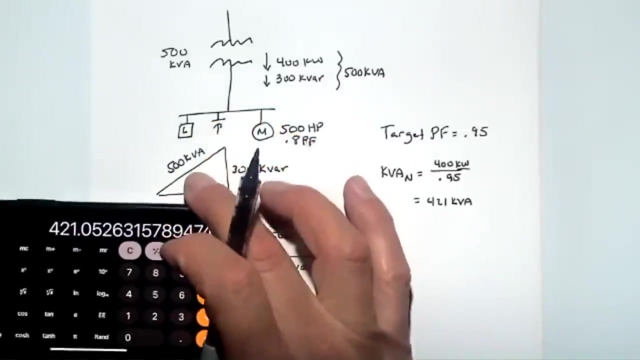 So if I do that, I take 400 divided by 0.95 and end up with 421 kVA. That's going to be my new kVA And that's what I'm going to shoot for by adding a capacitor. So how do I size that capacitor? 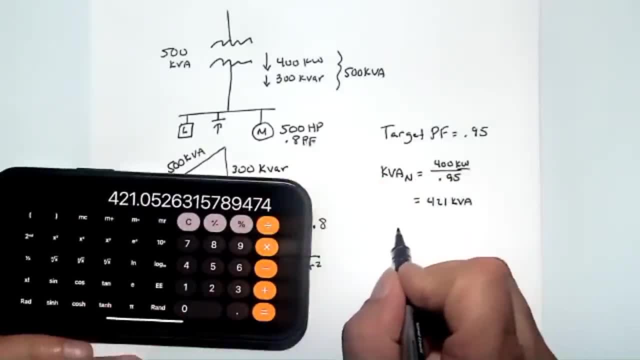 Well, first I have to figure out how many kVAR are left. if I do that- And I know my new kVA is that, So my kVAR would then be: kVAR would then be square root of 421 squared minus 400 squared, which is my kilowatts. 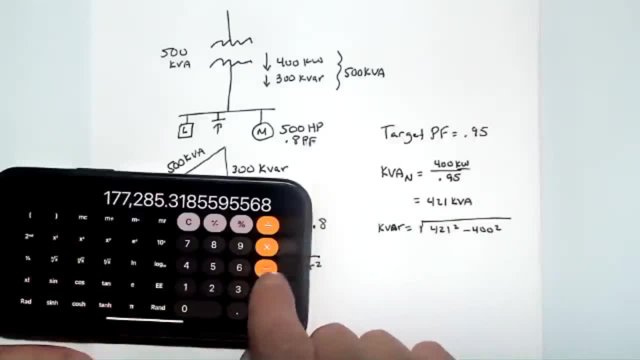 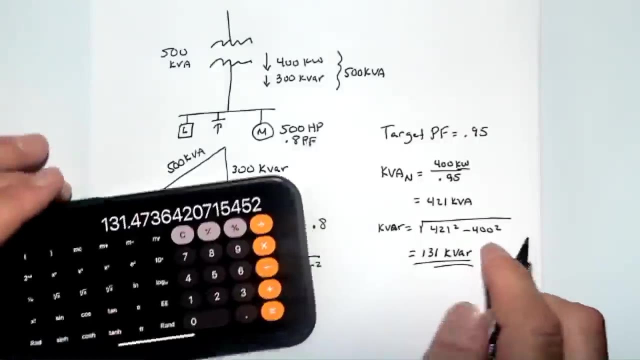 So 421 squared minus 400 squared. Take the square root of that And I'm left with 131 kVAR. Now, what's important to know about that is that's what's going to be flowing up through here on 31.. 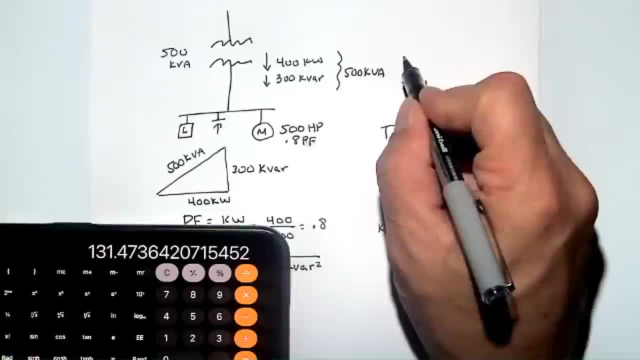 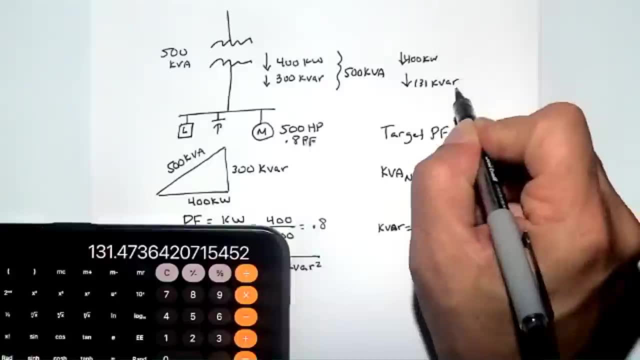 If we had perfect, if we had a 0.95 power factor, I still have 400 kilowatts flowing through there. What I have to do, though, is, when I apply a capacitor here, I have to negate what's already there, which is 300.. 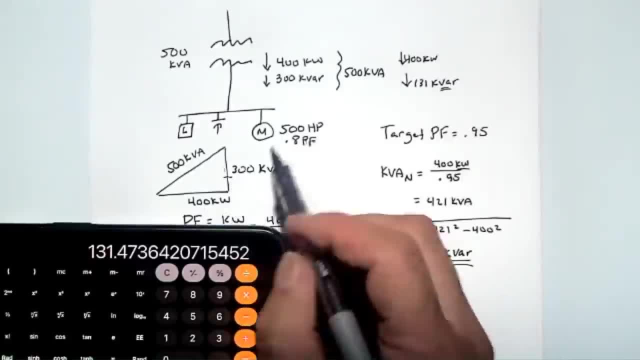 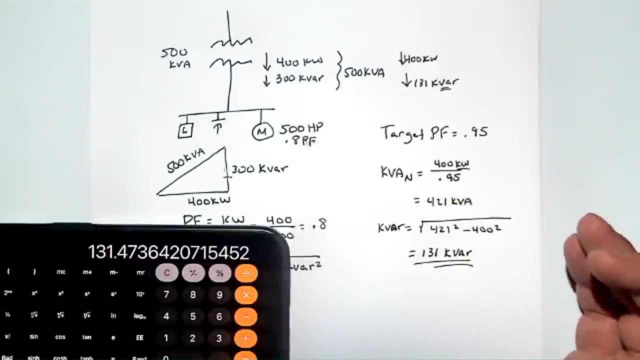 I have to get it down to 131.. So that means I have to add 169 kVAR capacitor. Well, we know we're not going to buy that, So because it's just not a standard size. So what we're going to have to buy is a 150, maybe, or 200 kVAR. 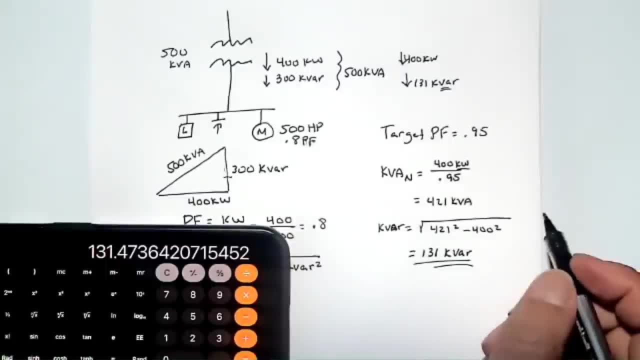 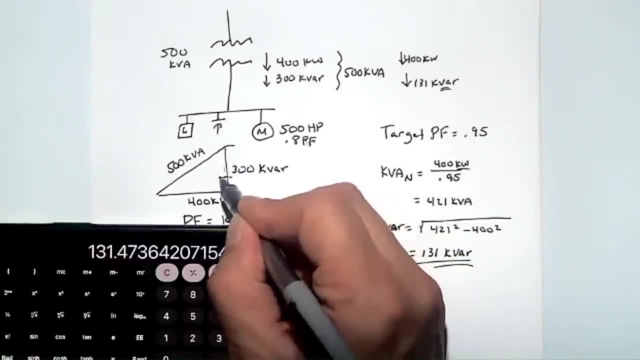 But since we know our target power factor is 0.95, I can't go lower than the number I came up with. So I'm going to have to go higher, And so what I'm going to do is I'm going to apply a 200 kVAR capacitor here. 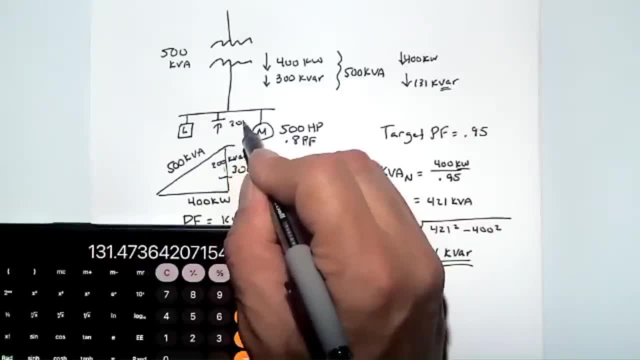 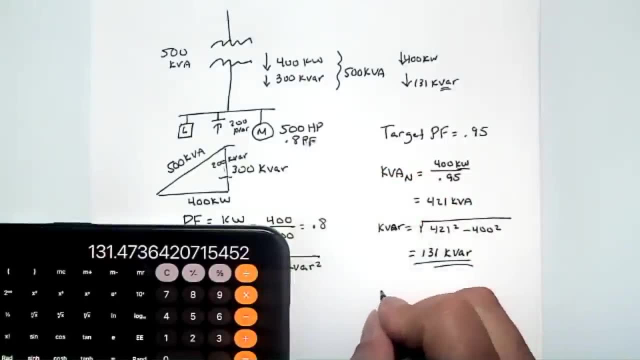 200 kVAR to negate that. So that means I'm putting a 200 kVAR capacitor here. And what am I going to end up with? Well, if I put a 200 kVAR capacitor in there, now my new kVA. 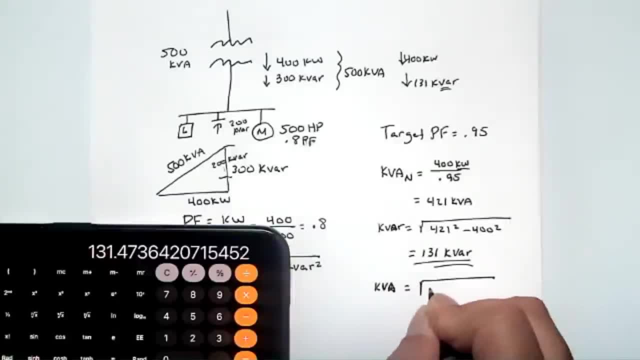 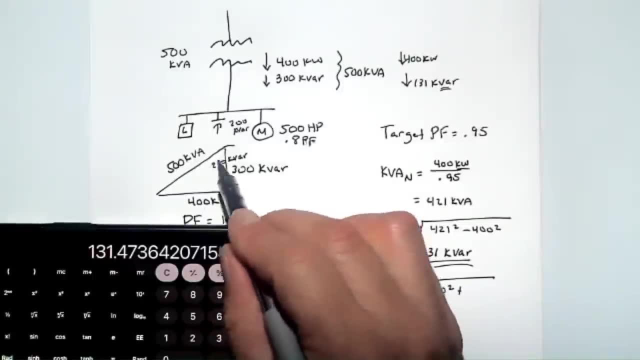 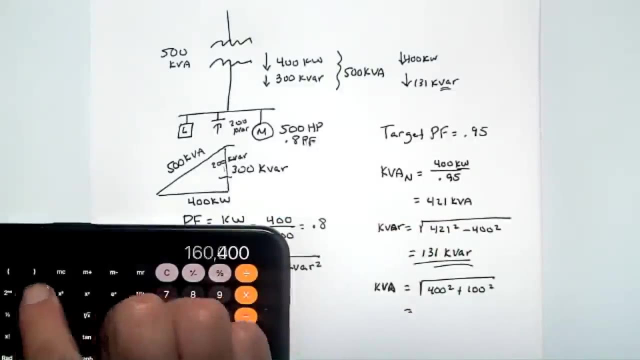 My new kVA is kilowatt squared, so 400 squared Plus 300, minus the 200 I'm putting in there, So plus 100 squared, My new kVA: 400 squared Plus 100 squared. And then take the square root of that. 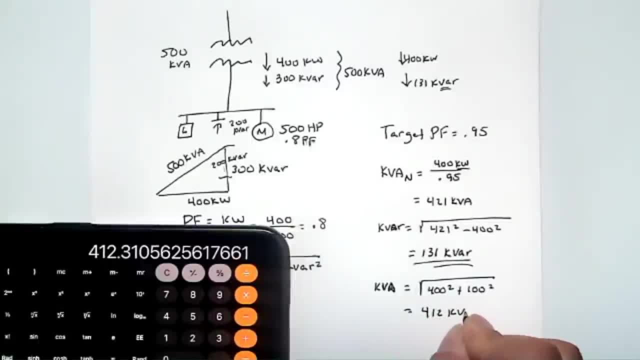 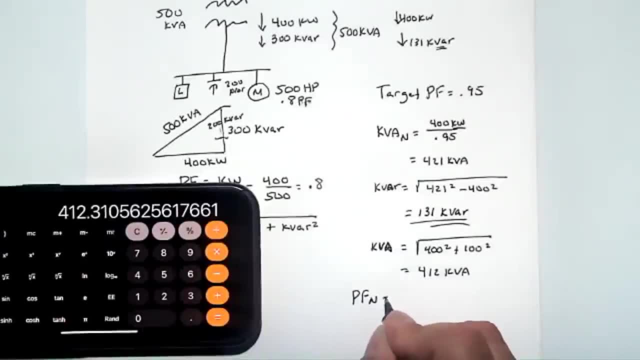 412 kVA. And so now my new power factor. My power factor new is not 0.95.. It's actually better than that. It's 400 divided by 412.. 400 divided by 412.. And my new power factor is 0.97. 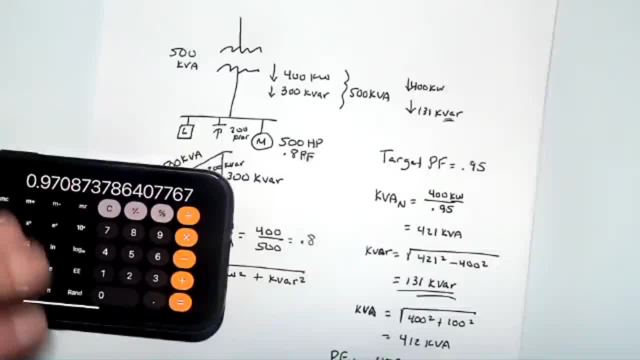 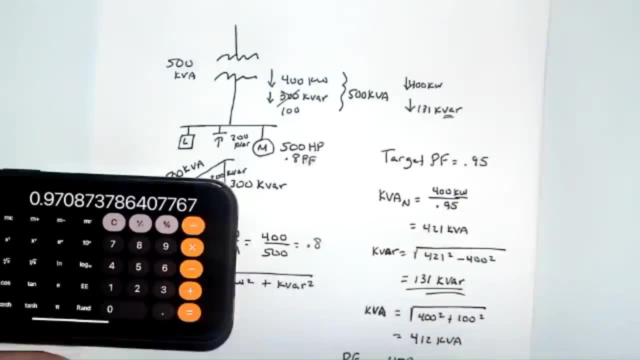 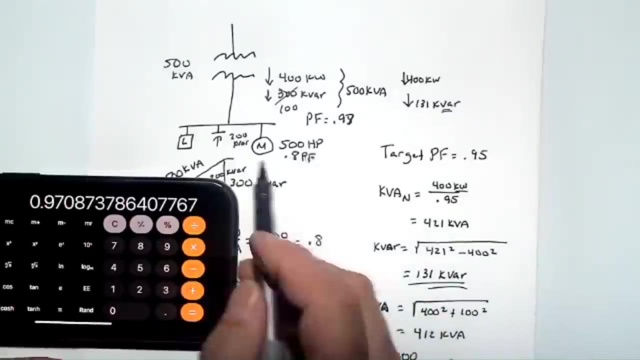 So what that means is I now have on my transformer up here. I have 400 kilowatts still flowing, I have 100 kVAR flowing And my new power factor is 0.97.. And that's how I do my power factor correction: by adding a 200 kVAR capacitor to an existing load. 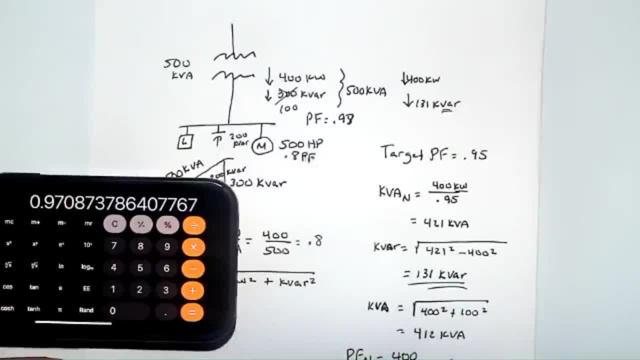 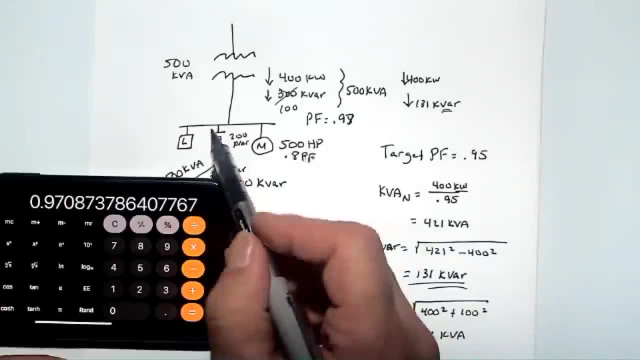 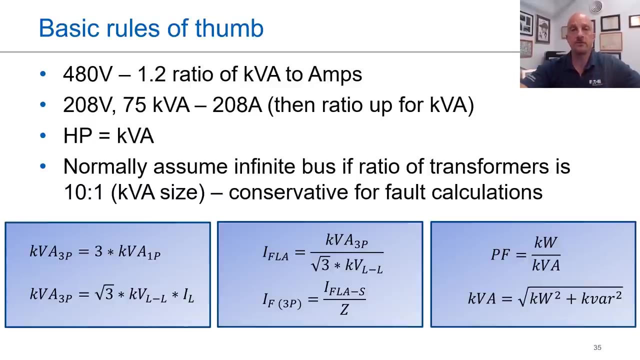 That frees up some capacity of the transformer in terms of 500 kVA. Now I can add another, you know roughly 88 kVA of load, without any concern. Okay, so we went through all these calculations. We showed you some examples of rules of thumb. 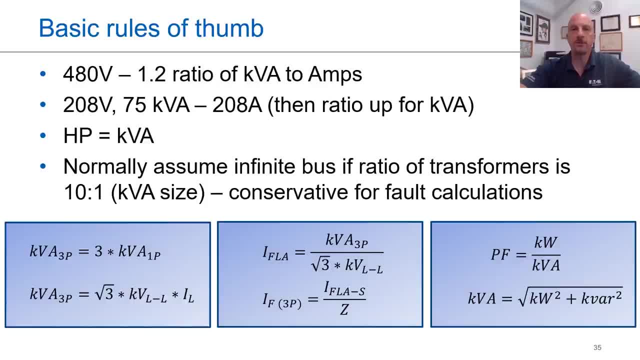 What are some of the key ones that we pointed out during the actual examples For four 80-volt systems? basically, the amps versus kVA is about a 1.2 factor. So if I'm at 75 kVA, I'm about 90 amps. 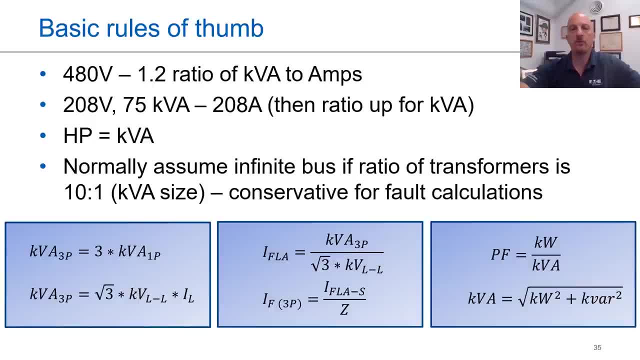 And that's a really important and easy one to kind of remember. So if I'm at 750 kVA, I'm at 900 amps. Those are things that you're going to want to keep in the back of your mind So you know when the person next to you has that kind of quick calculation in the back of their pocket. 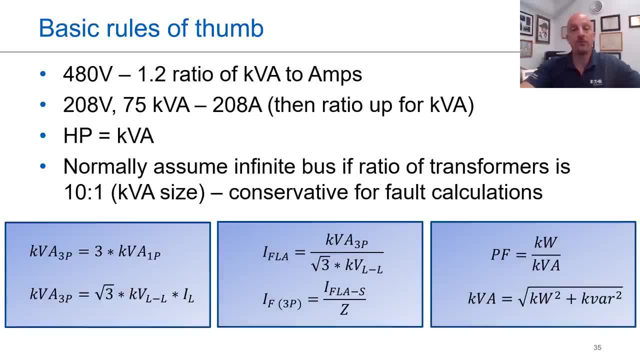 that's where they're getting that: 208 volts, 208 amps at 75 kVA And you can scale it up and down from there. So if you're at 300 kVA, you can multiply by a factor of 4, you know, and so forth. 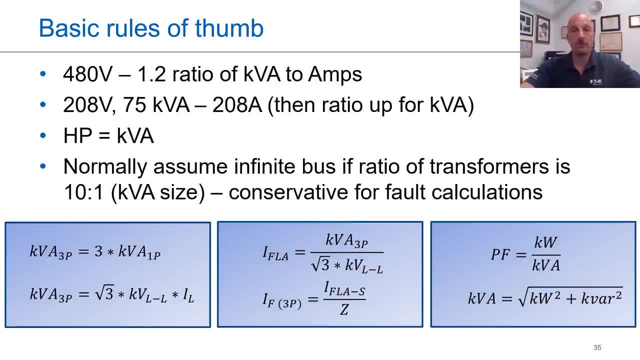 And I think that's a really important one to remember Again- you can impress your friends and your family. Horsepower is about equal to kVA, So if you're doing motor calculations you know you can put in the efficiency and you can put in the power factor and all that. 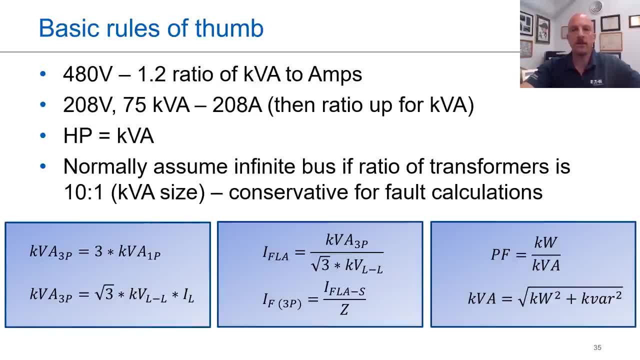 At the end of the day it's just about equal to kVA. So I think if you make those calculations you're not going to be off by much And if you are, again marginal on anything- And again this goes with any of these calculations- 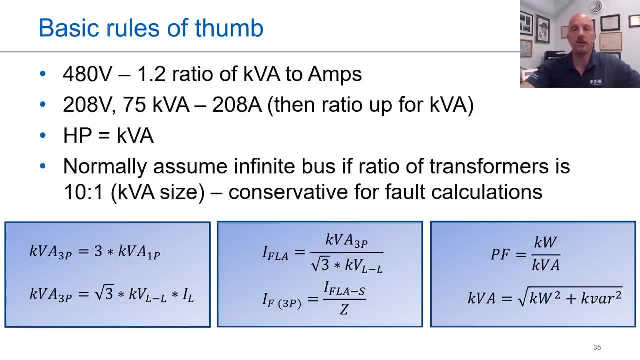 If you're marginal, you need to go back and kind of fine-tune it anyway And then normally assume an infinite bus if the transformer ratio is 10 to 1.2.. You know kVA-wise. So if I have 1,000 kVA transformer and I'm fed by a 10 mVA substation upstream or even bigger, I usually don't have to worry about anything in terms of my fault calculations and using that impedance to really affect things. 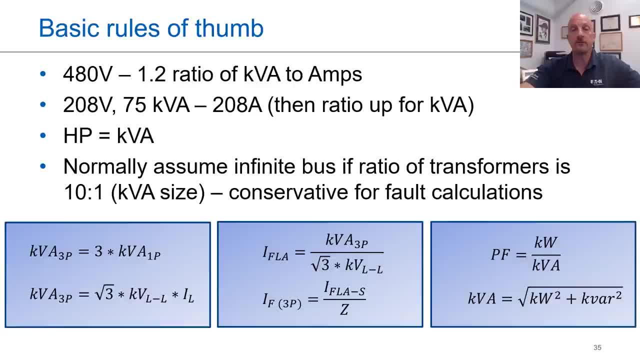 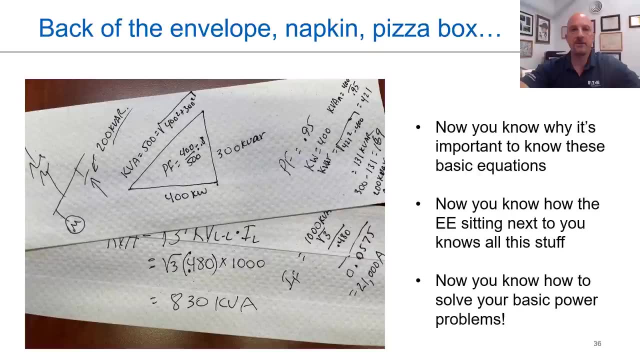 So I had a lot of fun doing this session And I think it's important that you kind of understand some of these basic calculations and things like that So you can do the back-of-the-envelope napkin or pizza box calculations as well. So now you know why it's important to know these basic equations. 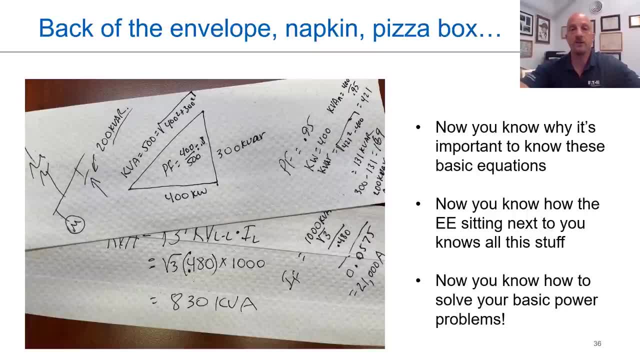 And I think, as a consultant, it's really important to understand where they come from And how you can get to these basic calculations. The second part is really knowing that the person next to you, through all that experience, this is the knowledge they've gained and they've been using these kind of calculations for a long time. 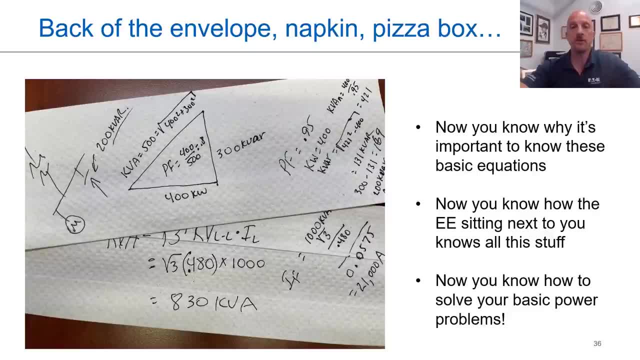 Power systems. if you understand those kind of key equations, you can get through a lot of the calculations that you need, And now you have all the tools to solve your basic power problems. So I hope you enjoyed it. Thank you very much for joining us. Thank you.